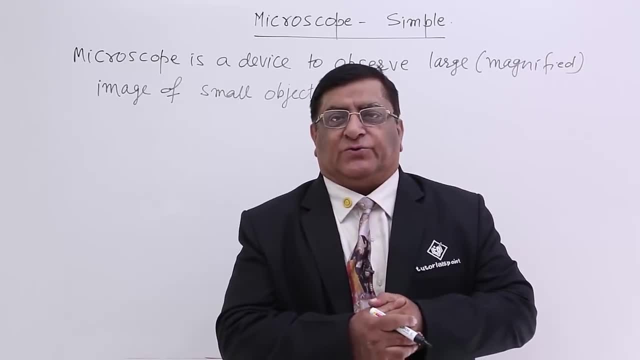 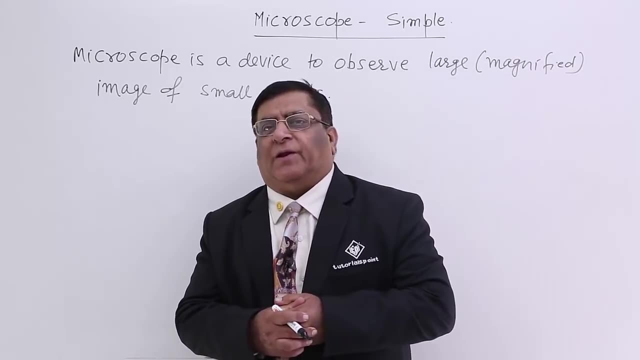 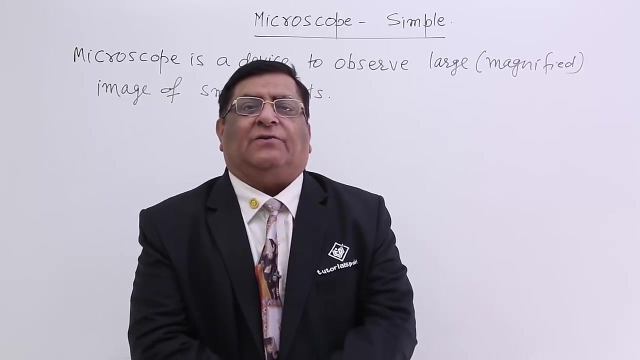 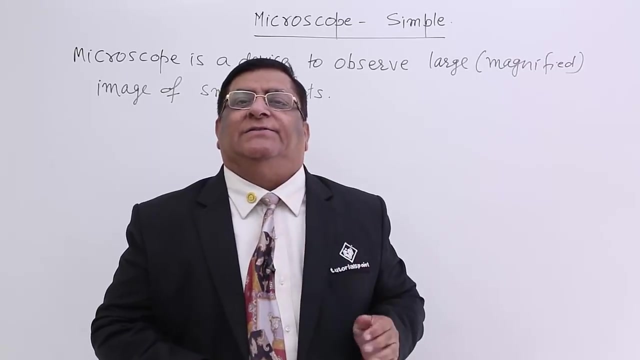 objects in microscope, what is power of a microscope and how we construct it. So, the first thing, we will study the principle of microscope, that it makes a large image of a small object. and we start with the simplest microscope. simplest, yes, it is only one convex lens. 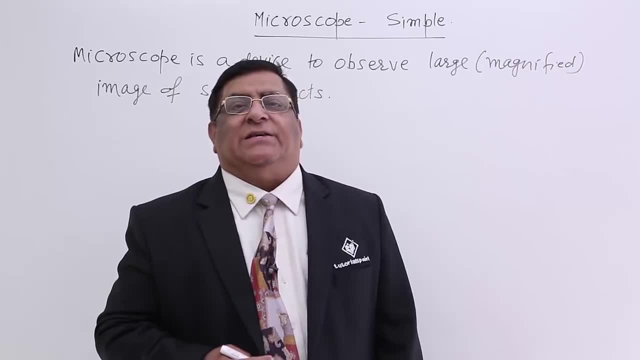 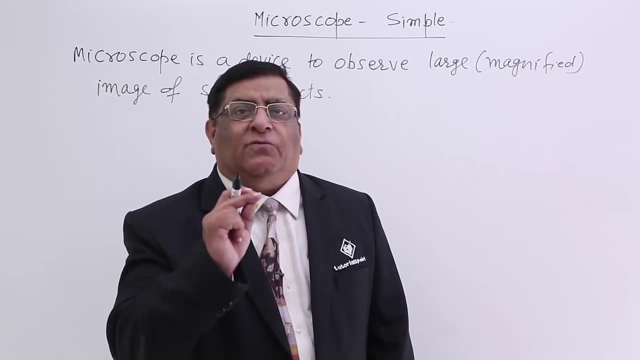 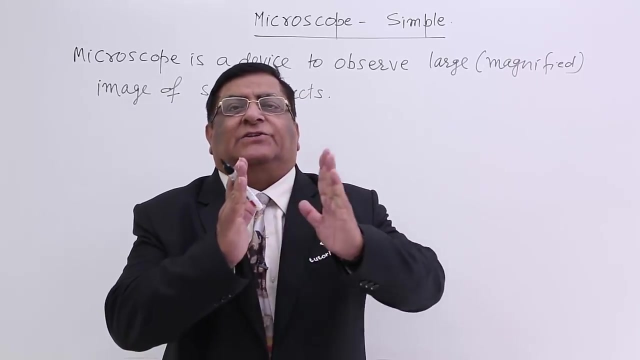 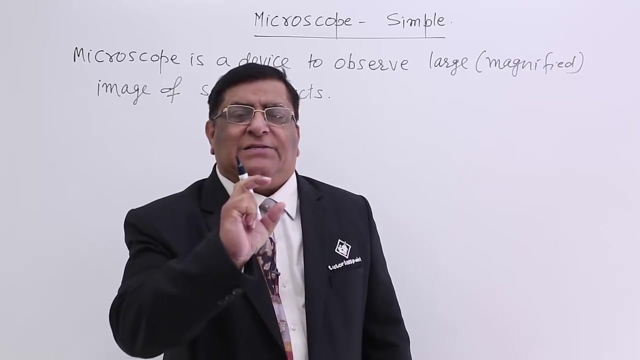 How a convex lens is used as a microscope. The answer is: a convex lens is used as a microscope if we place the object at a small distance, the distance which is less than its focal length. If an object is placed close to the spherical lens at a distance less than focal length, 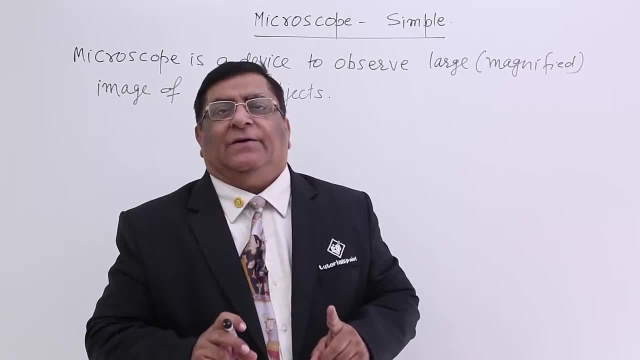 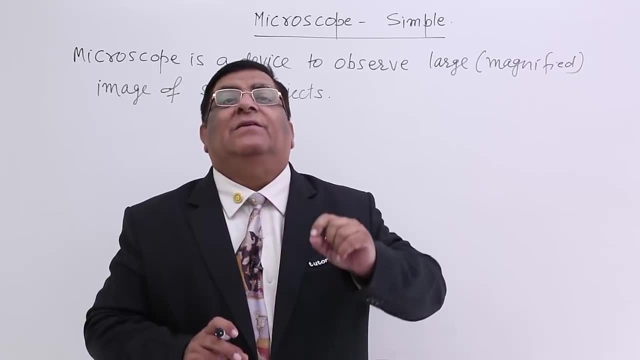 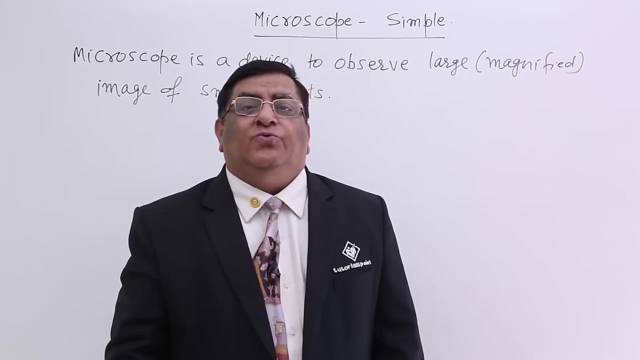 that is, between focus and optical centre. Then from the other side We see the image and that image is large image. ok, that is one thing. other thing: how do we see the things large and clear? this is very necessary for us to see that if the things 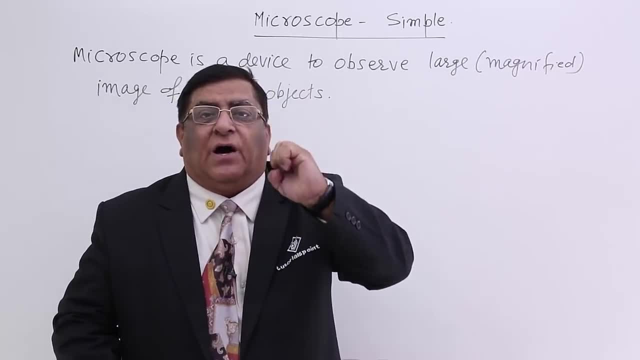 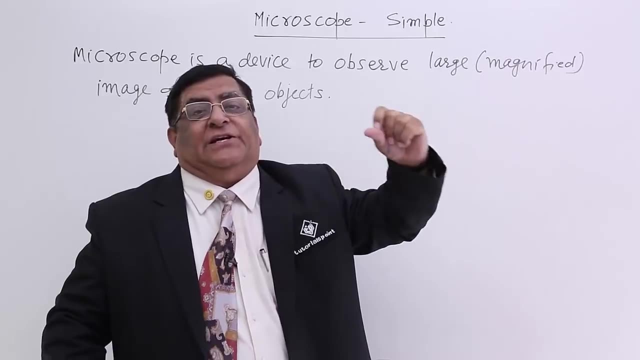 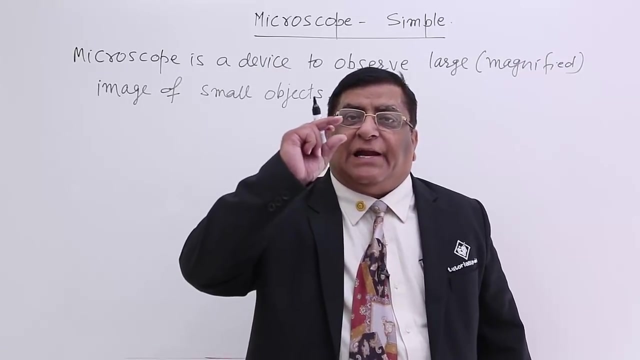 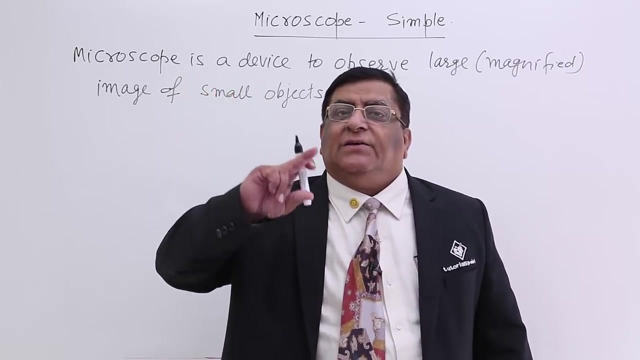 are large, magnified, how large, how magnified they are? how do we measure this factor? we will call it magnification. If there is a microscope which is enlarging an object 10 times and there is another microscope which is enlarging it 20 times, we will say: the second one has got better magnification. 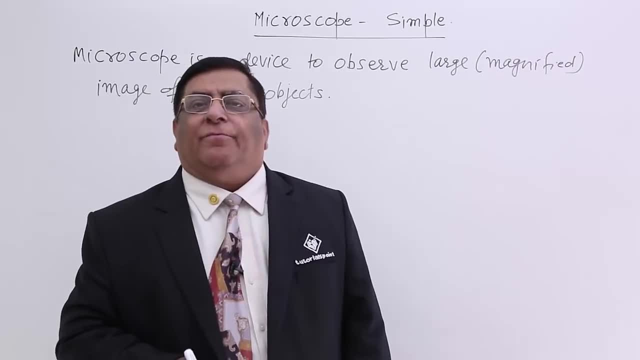 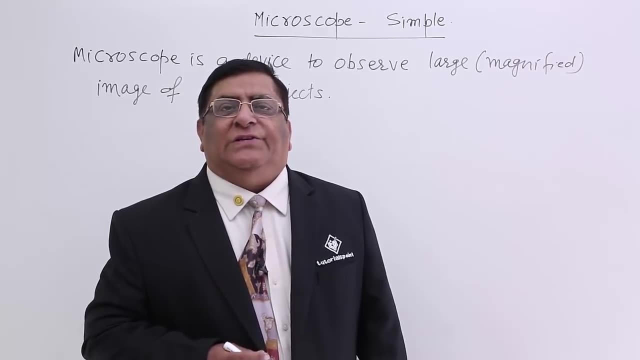 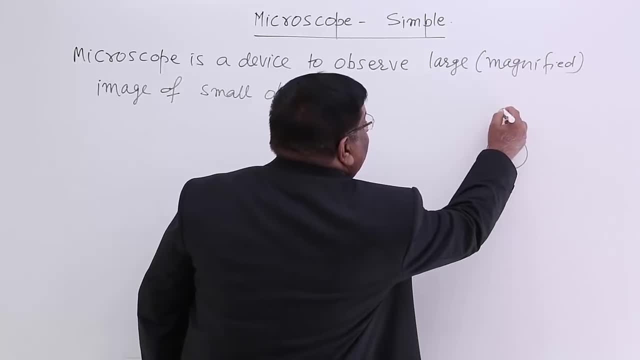 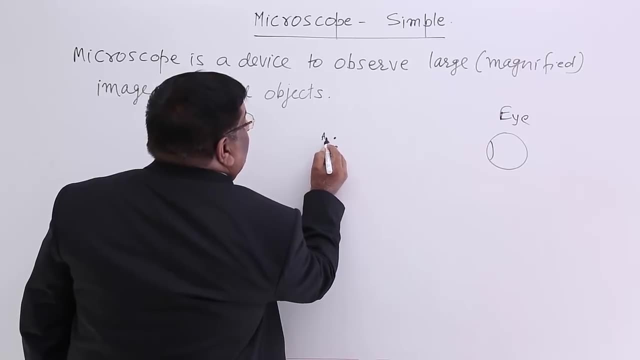 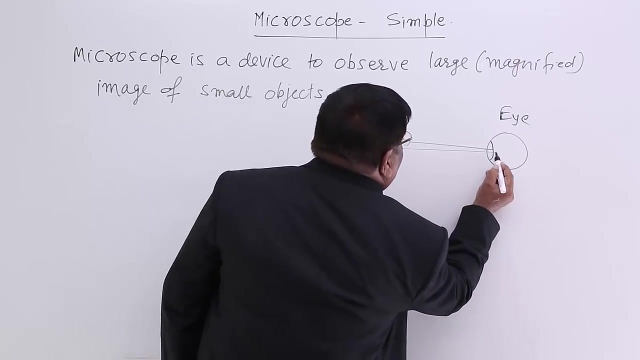 to our eyes. This is our eye. Here is an object. A to B. from A, the rays are coming in this direction and from B, the rays are coming in this direction. from B, the rays are coming in this direction and they make an angle between them. 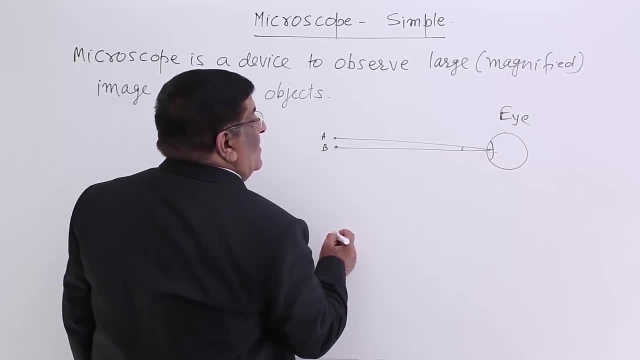 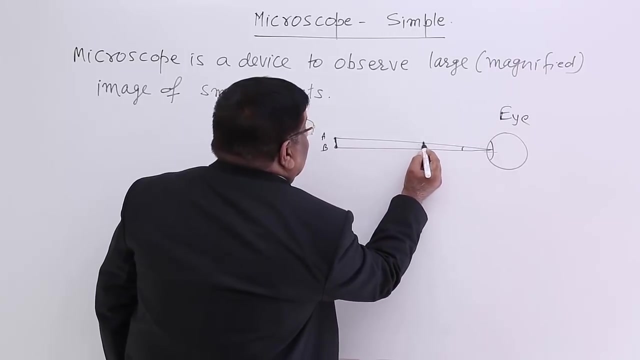 decision point in common And according to this angle we see this object, how large it is. Now, suppose for the same eye if we bring this object at this place. bring it at this place, same object here. Now, this makes angle on the eye, this and this. 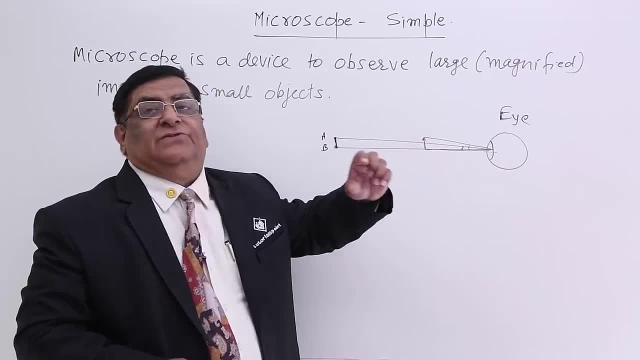 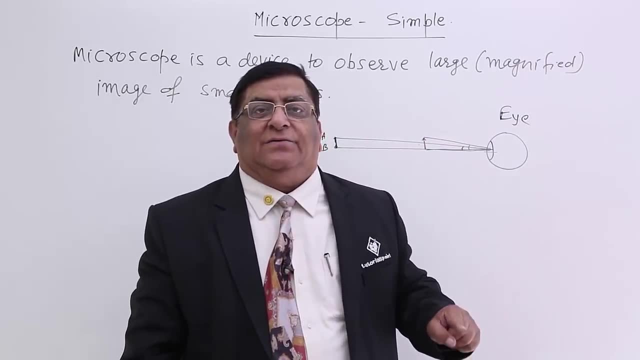 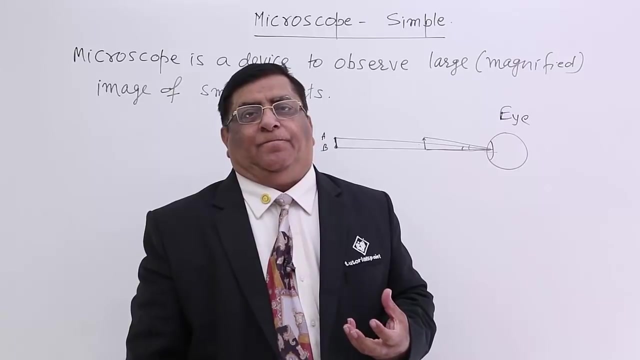 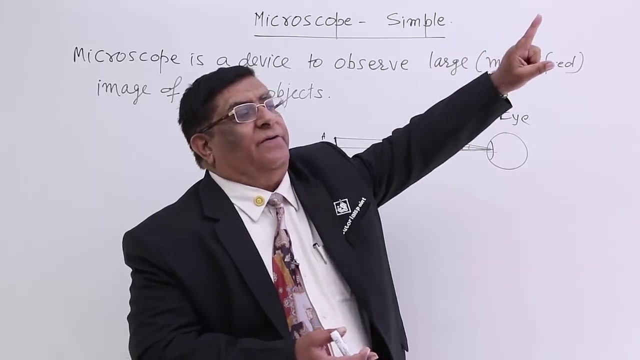 This is a larger angle and we see this object is large. So this angle subtended on the eye decides whether we are seeing that object large or we are seeing that object small. I can see a very large hill Here which is far away. that makes a very small angle on my eye. 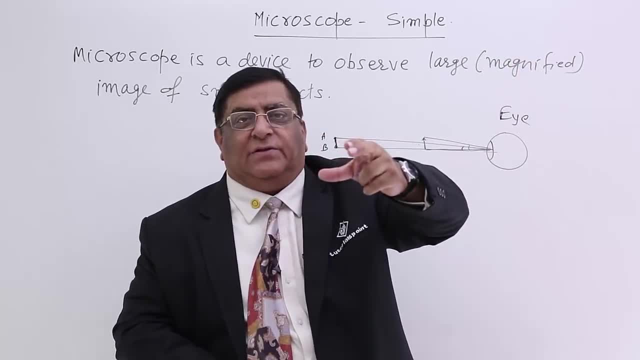 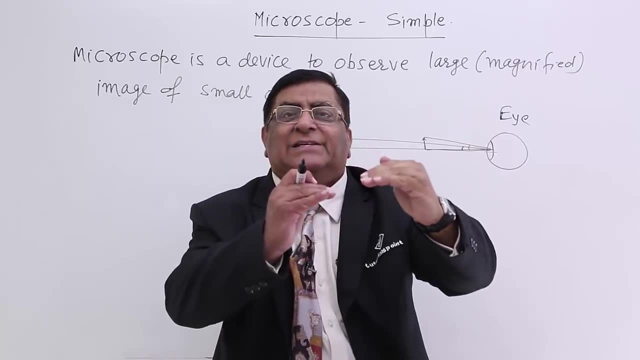 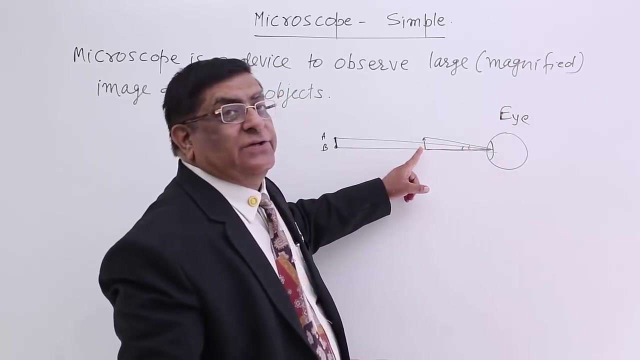 So that appears to me like this: You have seen Taj Mahal within this. Why? That was far away and it looks small, because that makes a smaller angle. But as we go close and close to this hill, we are moving closer to this hill. then we 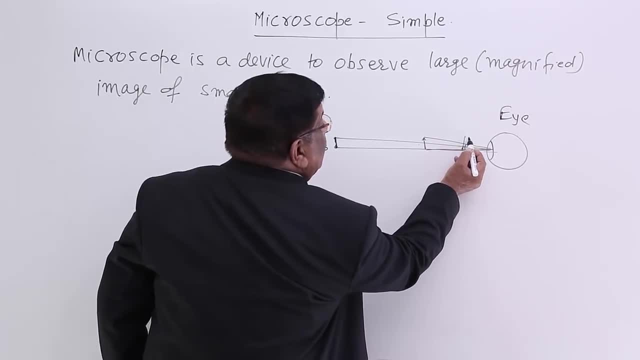 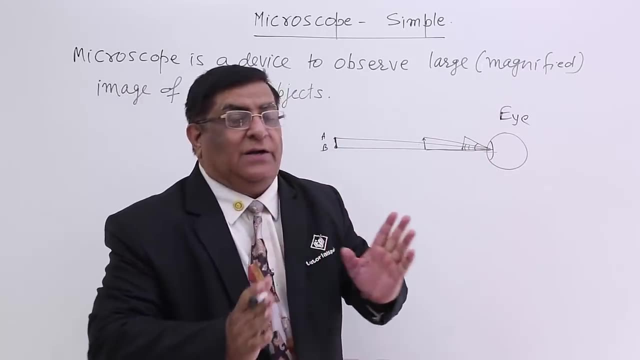 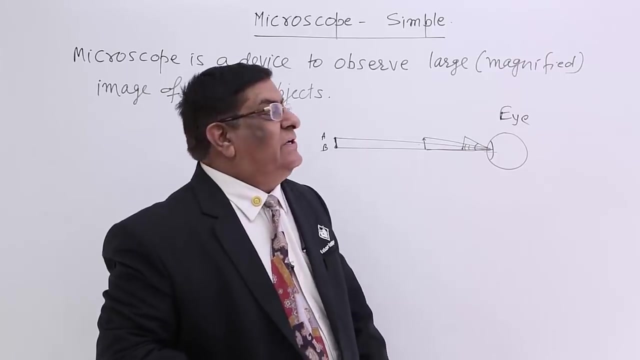 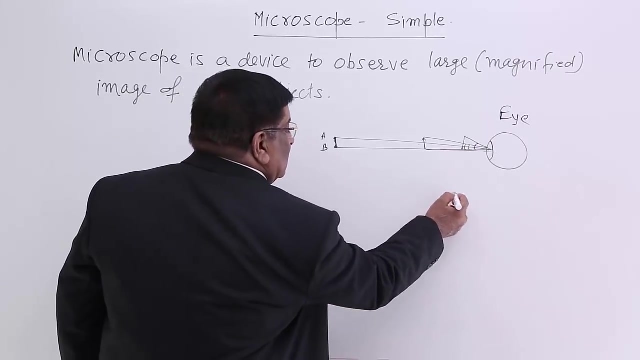 see this angle become large. It comes here. This angle becomes so large, So more is this angular size and that gives us a feeling that it is a large object. So this is angle dispersed by the object. Now, if I see an object which is this much large, 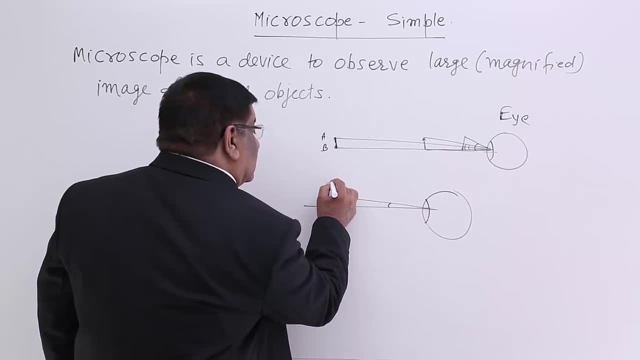 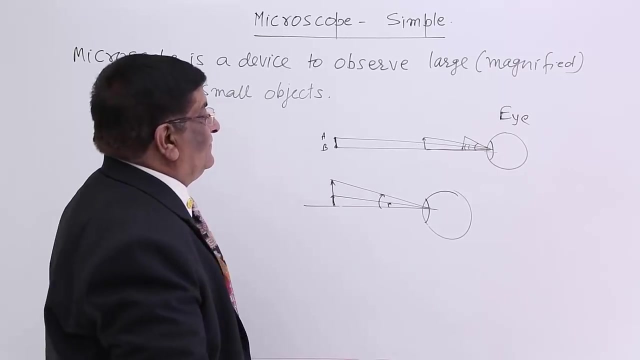 This is the angle. If I place an object here which is this much large, this is the angle made. This is angle made by one object. this is angle made by the second object. Second object is obviously larger, So there is one way this larger than this. 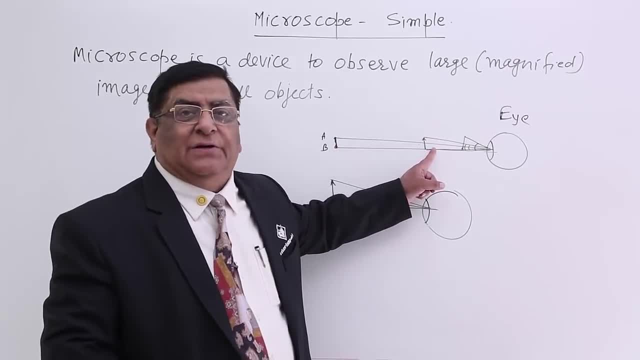 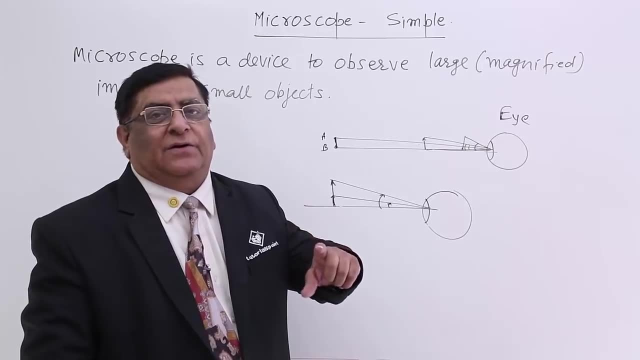 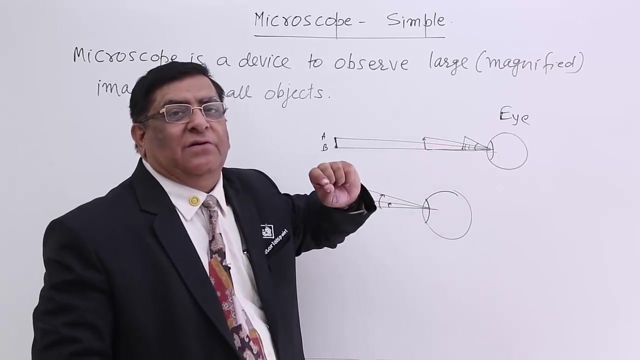 There is other way. bring it closer, it will appear larger In both the cases. what is the factor which decides that we see a thing larger? Answer: it is the angle subtended on the eye which decides whether we are seeing this thing. 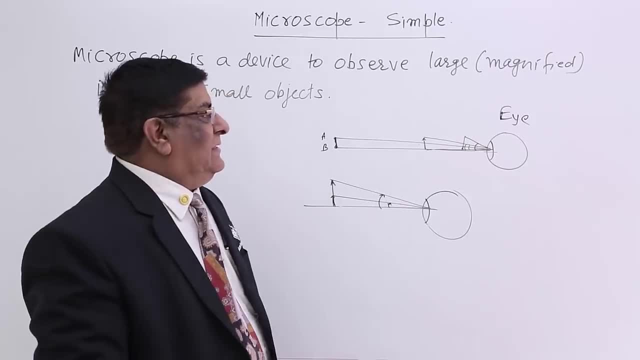 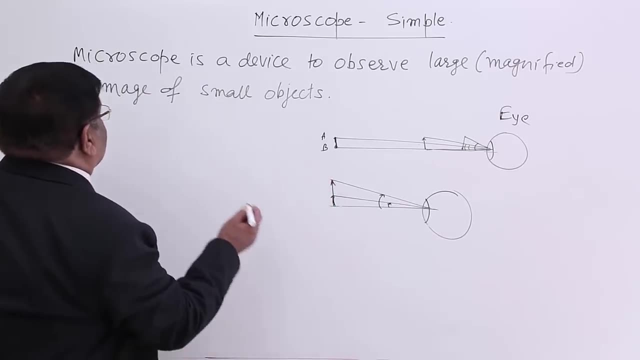 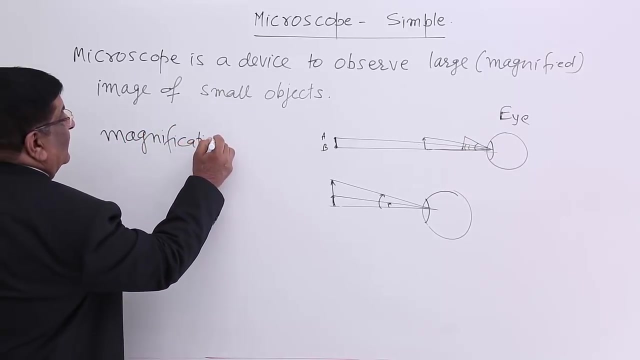 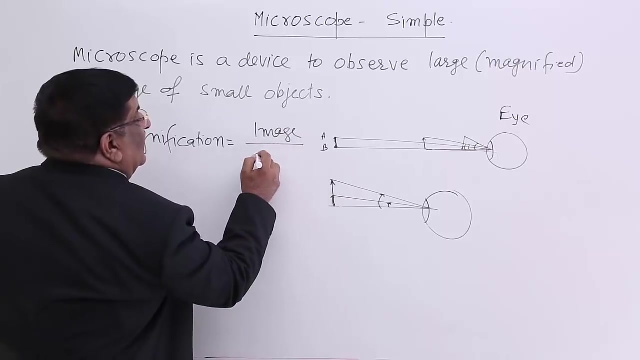 larger or smaller. That is one thing. Now here is a term which is how large. that is magnification. We have seen this term earlier. magnification And magnification is what size of image, image size divided by size of object. 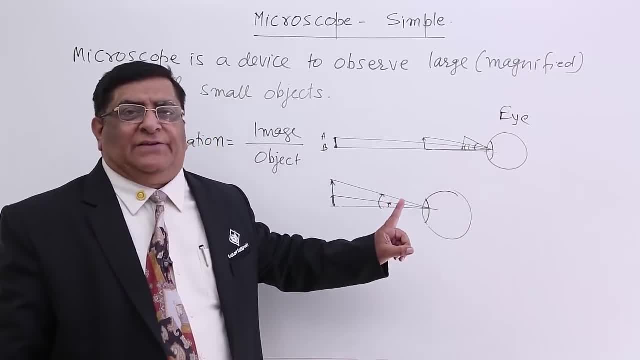 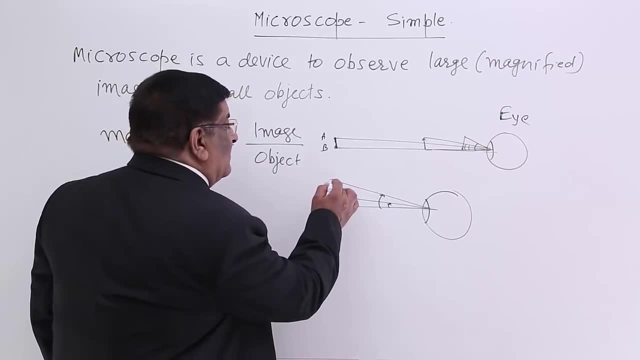 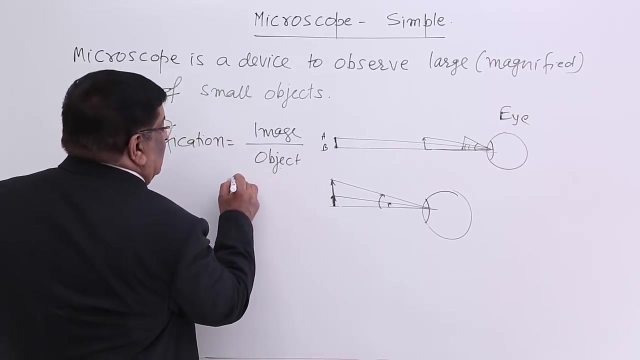 Now for any instrument: size of image and size of object, if you want to compare. there is a compulsory condition. The compulsory condition is that they must be placed at the same location. here This is image, This is object. Then the magnification will be size of image, size of object at the same location. 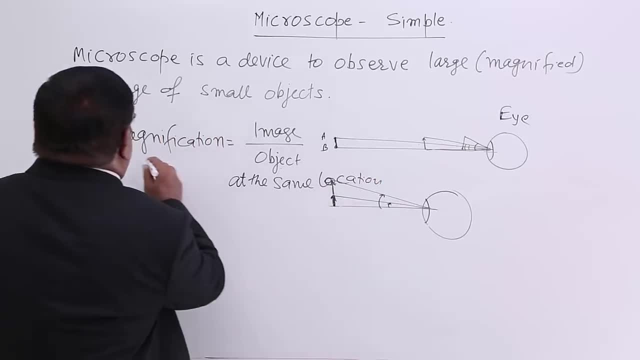 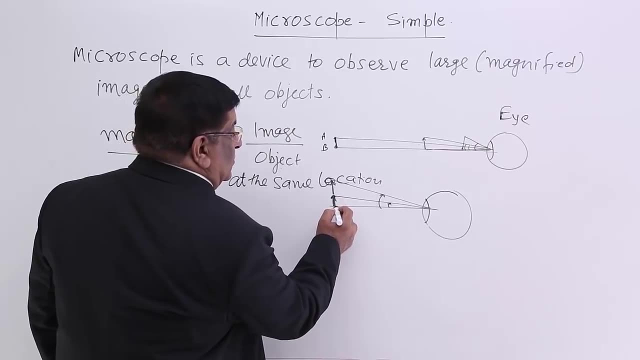 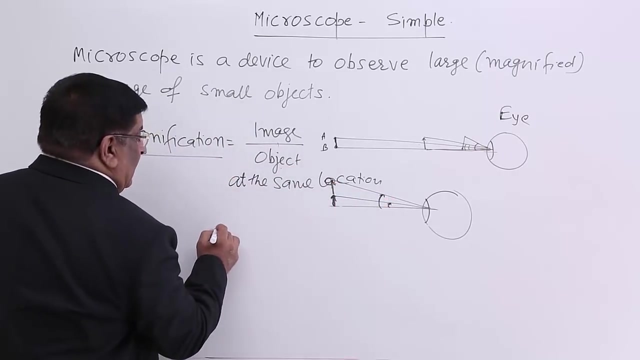 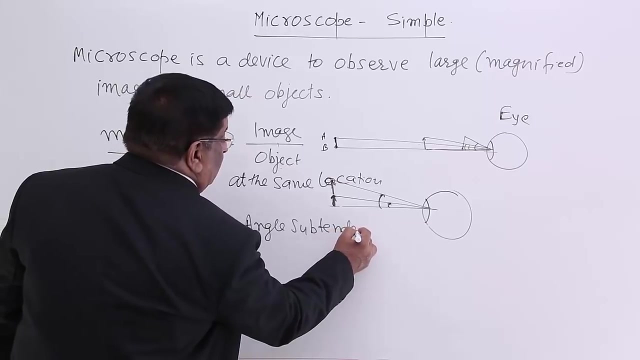 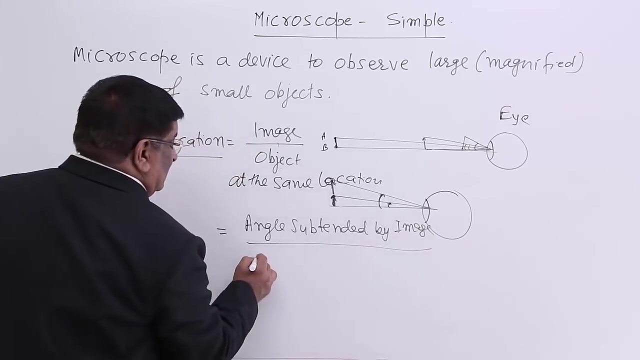 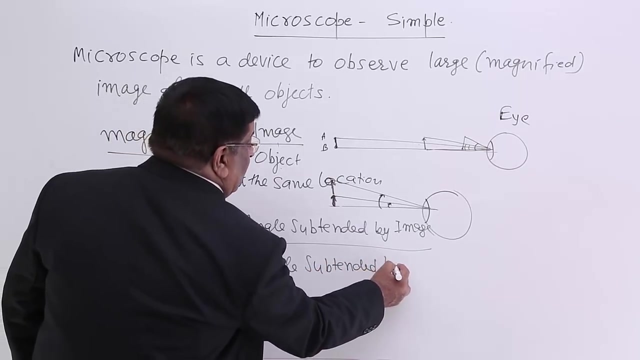 Please note it. This is the formula for magnification. Now, by geometry, we know that this is proportionate to this angle and this is proportionate to this angle. So this we can write. So we can write angle subtended by image divided by angle subtended by object. 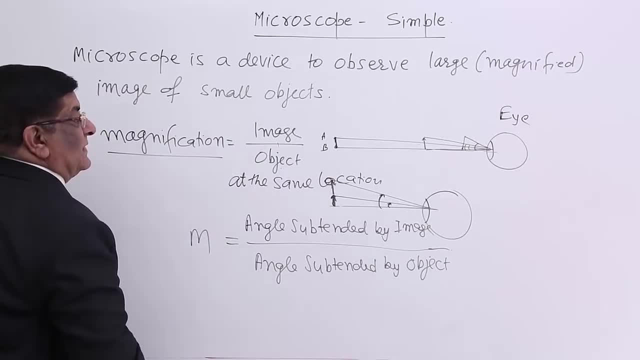 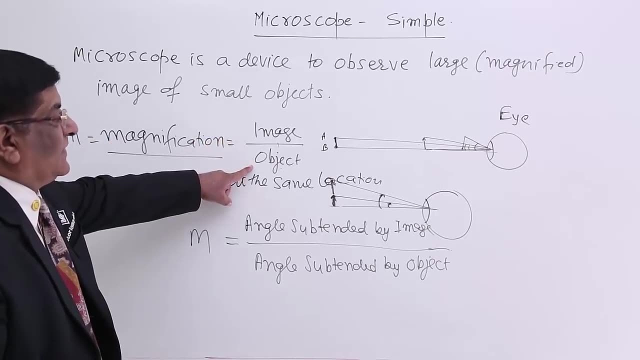 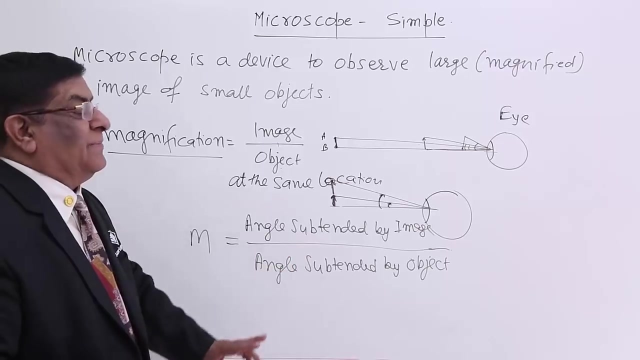 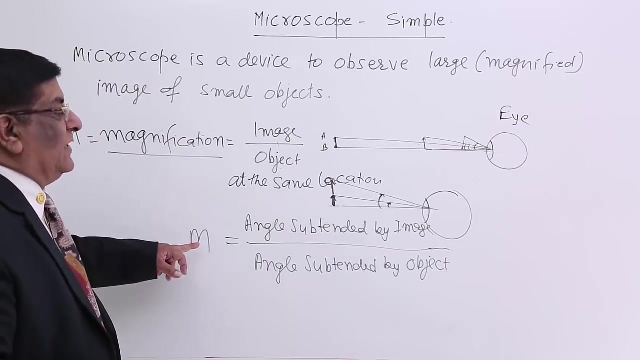 This is magnification. So this is magnification. So we have two formulas for magnification: Size of image upon size of object at the same location, or angle subtended by image divided by angle subtended by object. So this gives us magnification formulas. 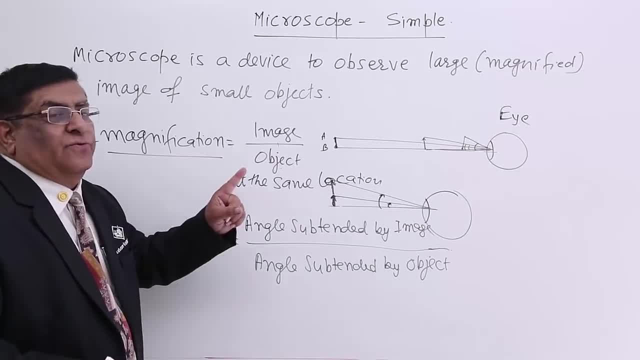 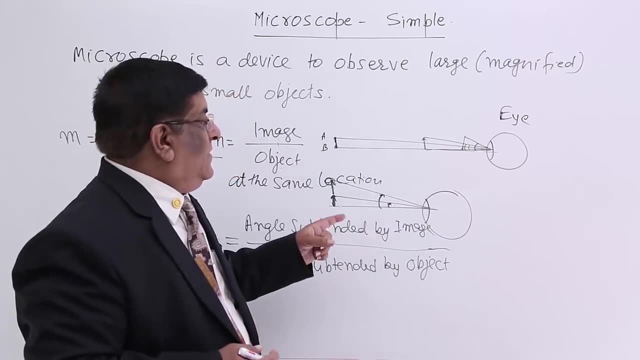 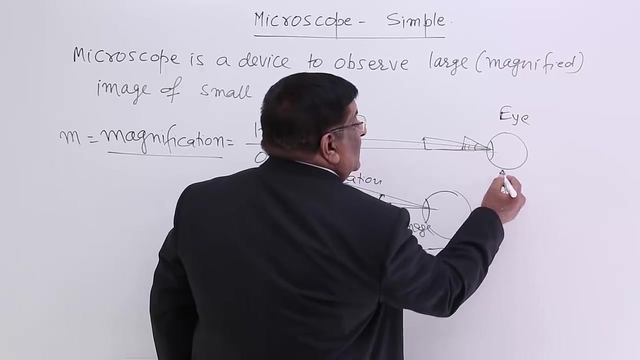 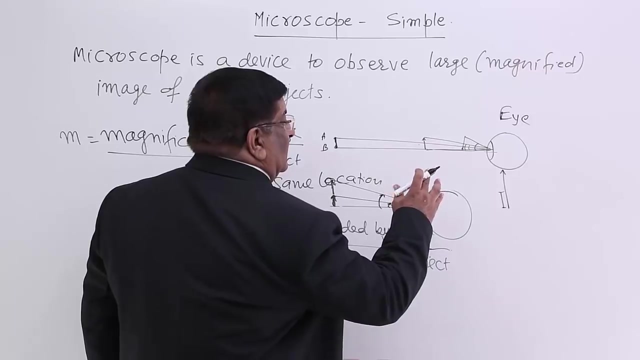 Either we will do this or we will do this to find out how much is the magnification. If we have an instrument which makes this object appear this much double, then its magnification is two times. So if we have an object, if we have a machine which will bring this object at this place, 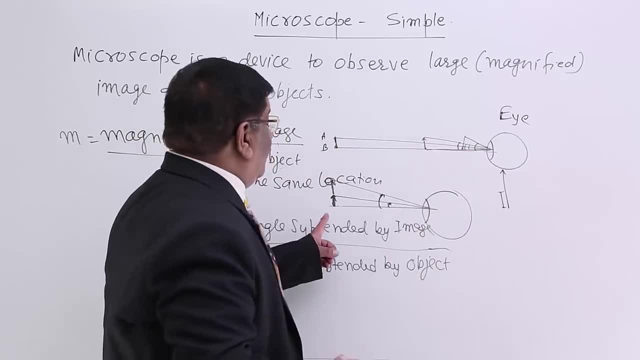 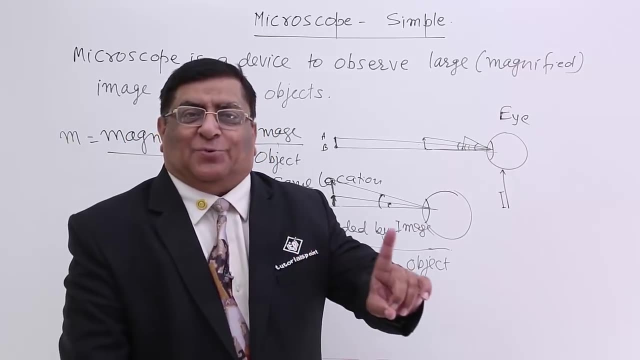 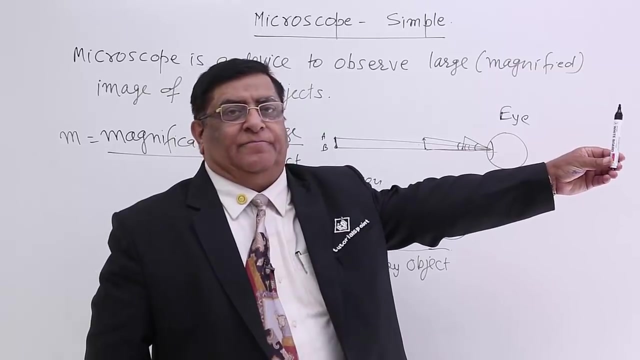 so that angle become larger, again there is a magnification. So in both the ways magnification will be there. Now another point, and that is very important point, If I want to see this object clearly- and this is far away, I am not able to read what it- 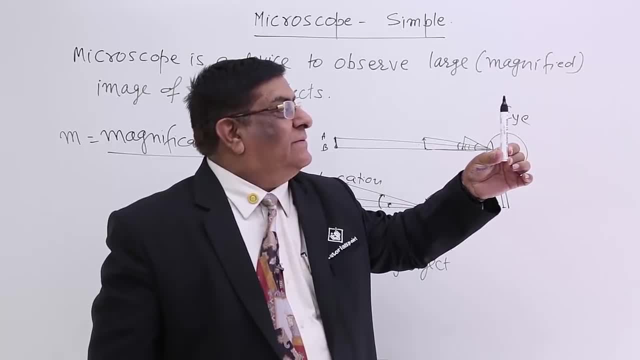 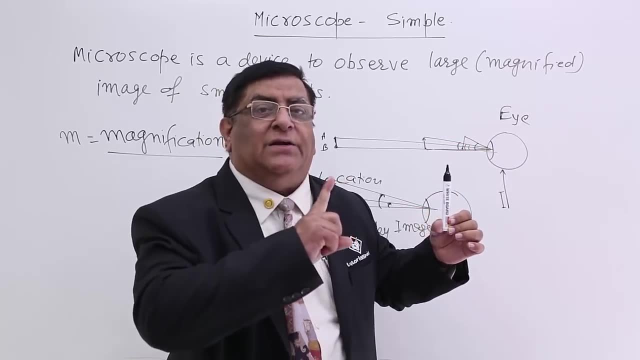 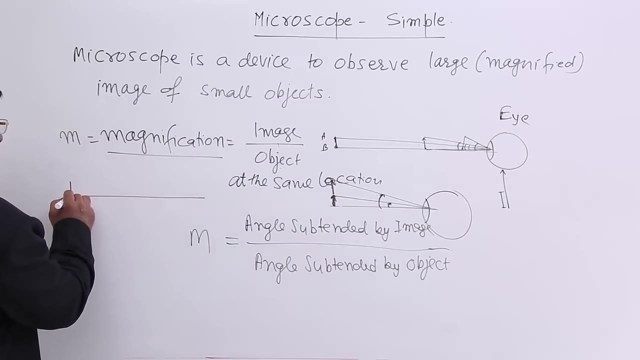 is. Then I bring it closer, It appears larger and clearer to me. Bring it closer, It again becomes more clear, more, larger. What is happening here? This is the object, This is the object. This is the object and it makes certain angle. 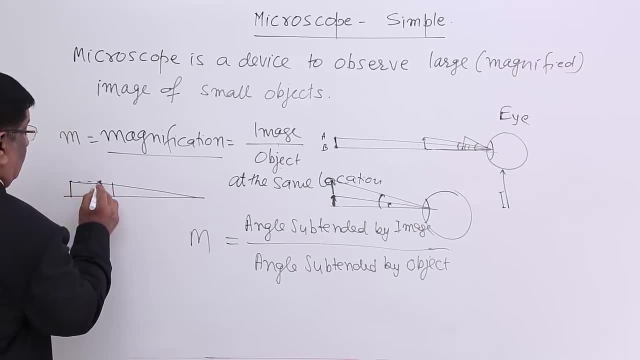 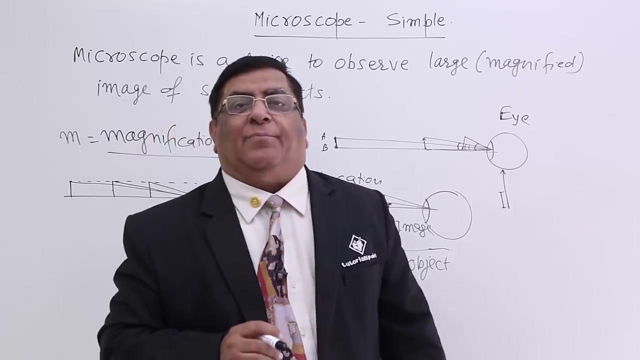 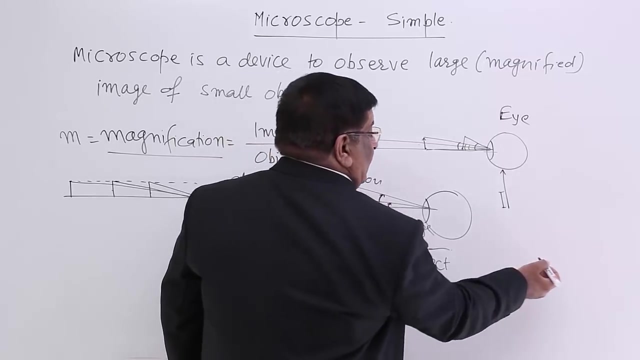 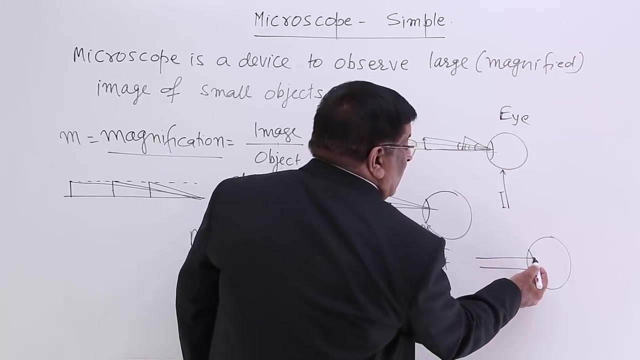 I bring it closer, Then it makes a larger angle, Further closer, it makes a larger angle and it becomes clear. But there is one special thing happening in our eyes and that is when this object was here, far away, When object was far away. these are the parallel rays coming from the object and they intersect. 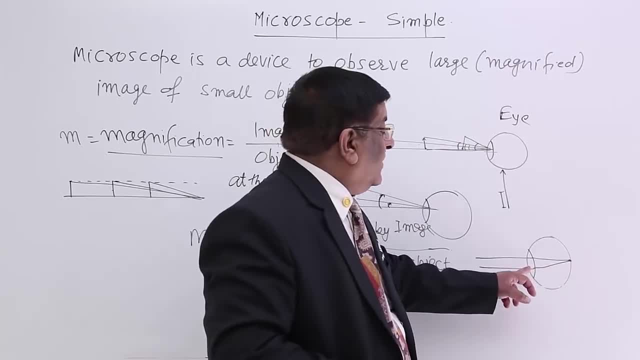 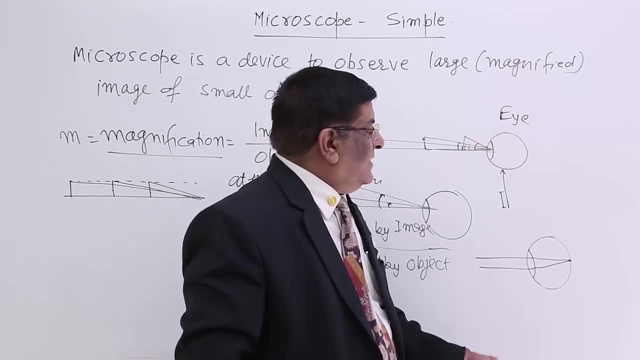 at this point, they meet at this point. This is the focus of this eye lens and it has got a certain distance, 2.5 cm or so. We are not studying that, but it is making a sharp image on retina and this object is. 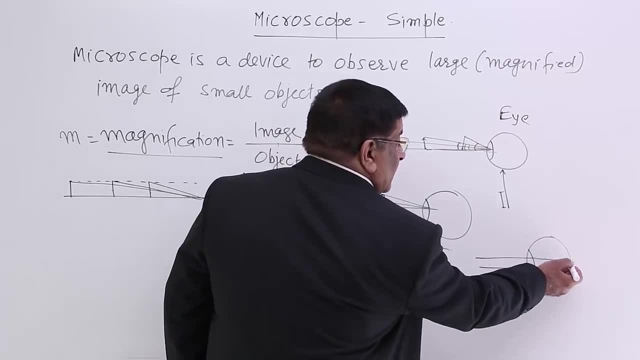 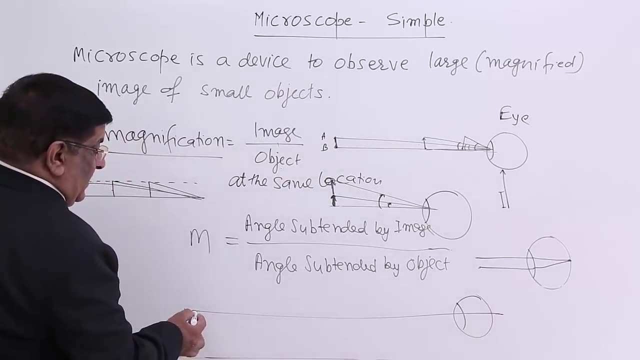 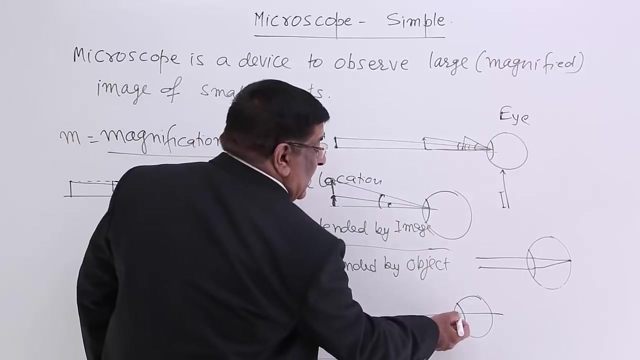 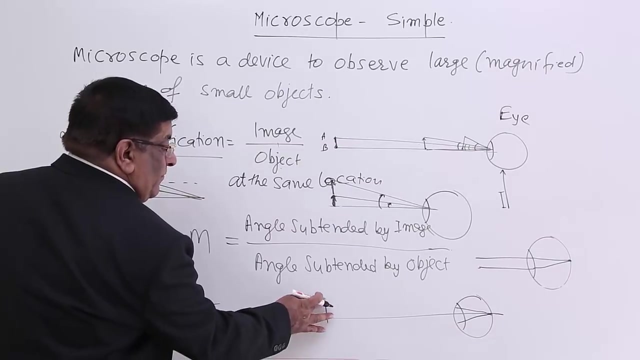 clear to us. Now suppose this object which was far away, It was here. So the rays going from here become parallel, almost parallel, and these parallel rays were meeting here. Now this object has come here. If this object has come here, naturally the angle will be less. 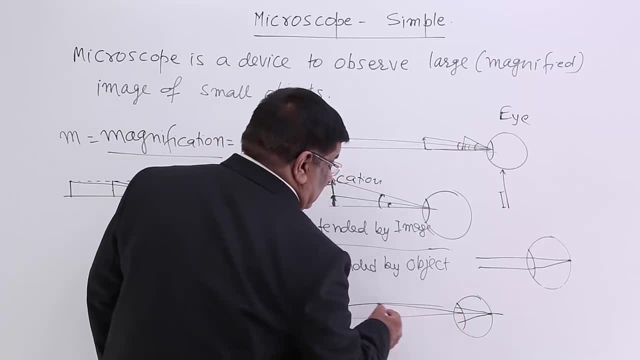 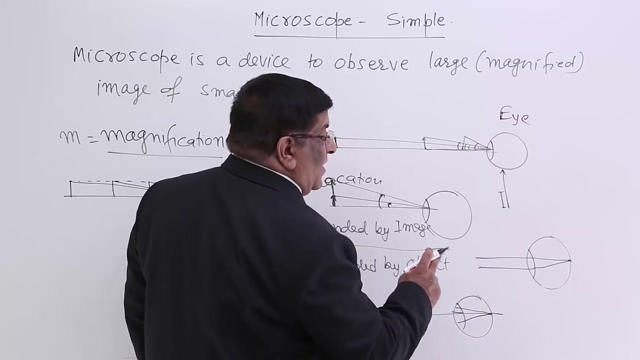 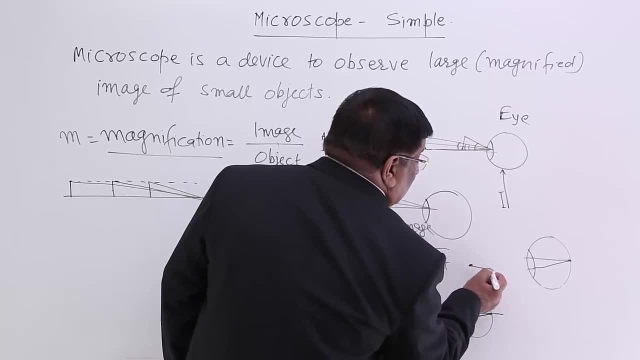 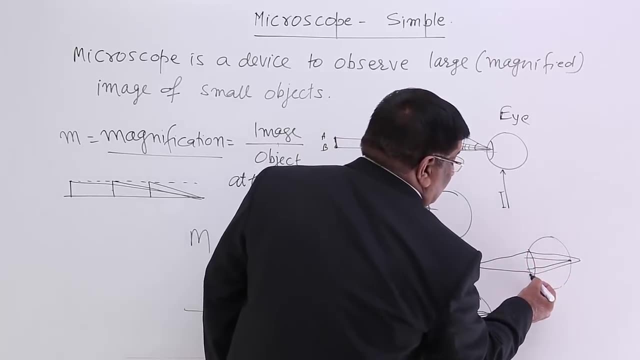 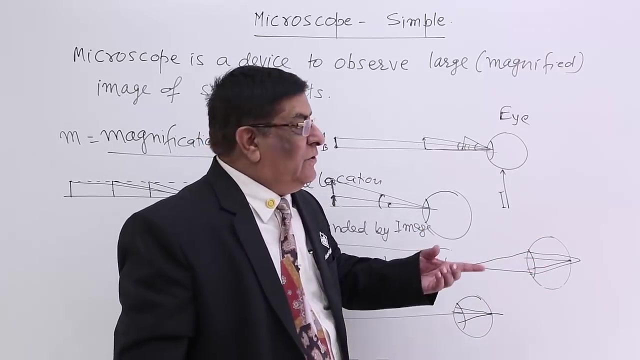 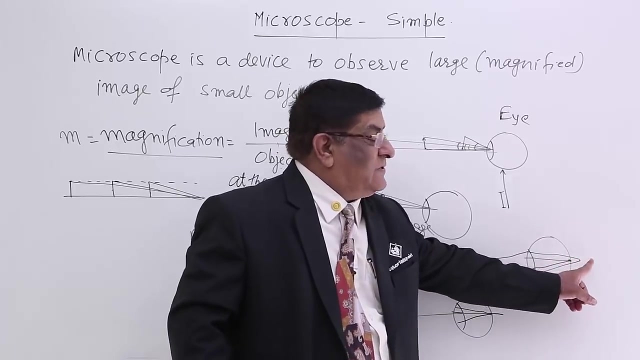 shape. If here is the object, then these are the two rays coming from this object, and when it bends, then they meet here. This way, This you can calculate by 1 upon v minus 1 upon u or by any method. So when we bring it closer, the image goes away. 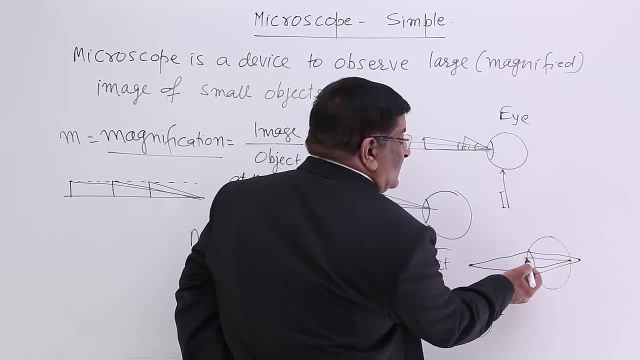 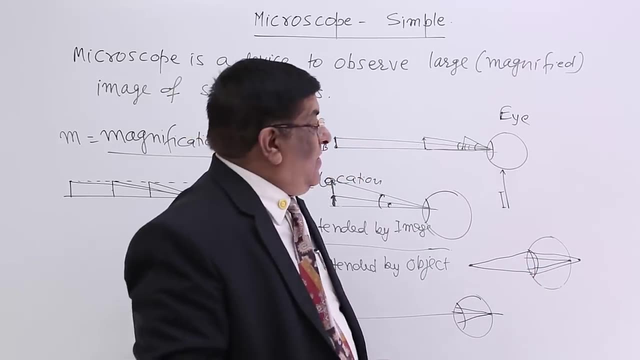 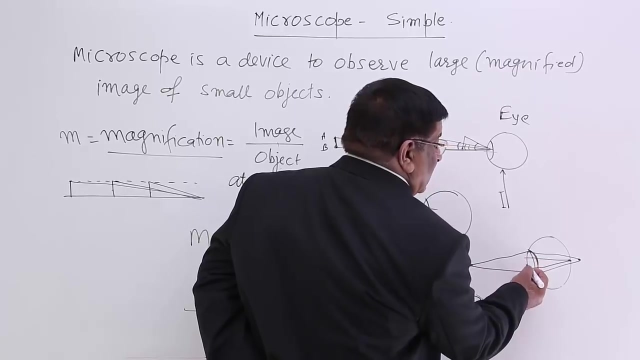 But we cannot see here. So what do we do? We change the focal length of our eye lens with help of ciliary muscles. With help of ciliary muscles, we change it And increase the focal length by changing this radius, by pressing it. 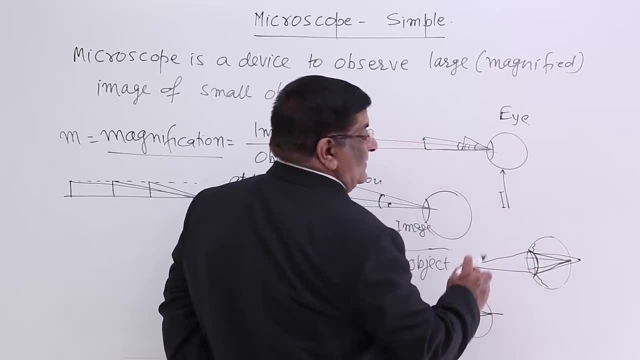 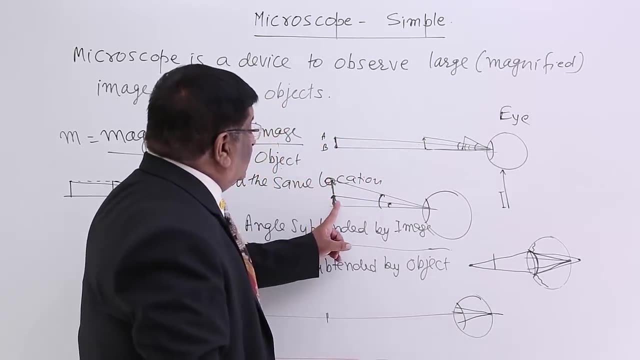 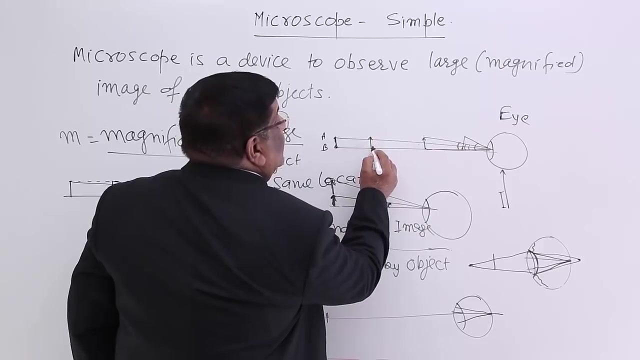 And again we focus it at this point: Again we bring it closer. Why we are bringing closer. When we bring it closer, closer, closer, it appears more clear: Here it is better looking, Here it is better looking, Here it is better looking. 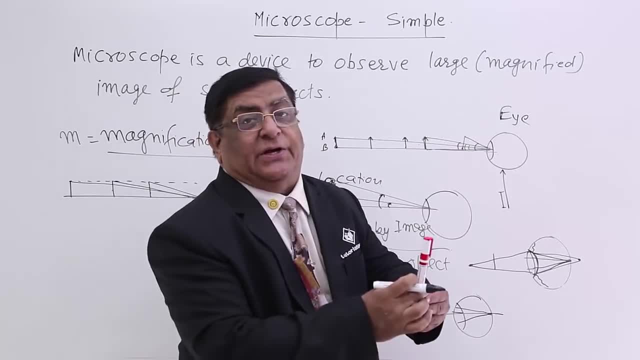 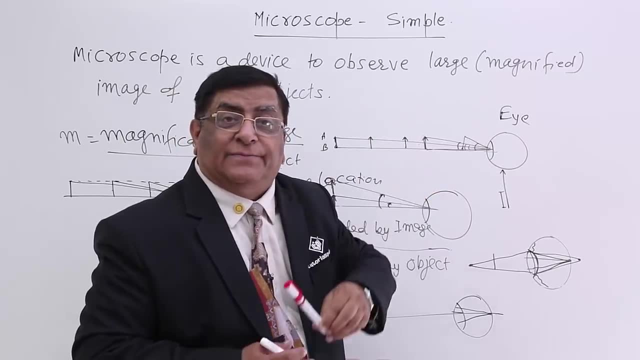 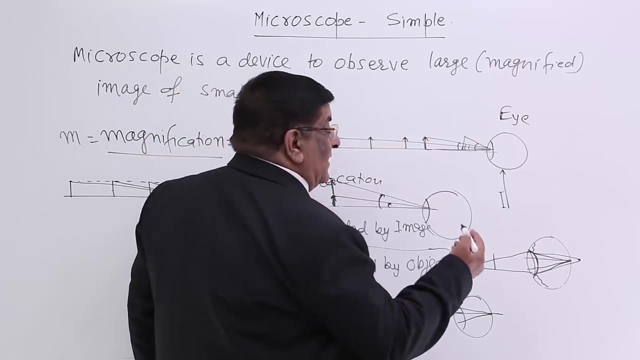 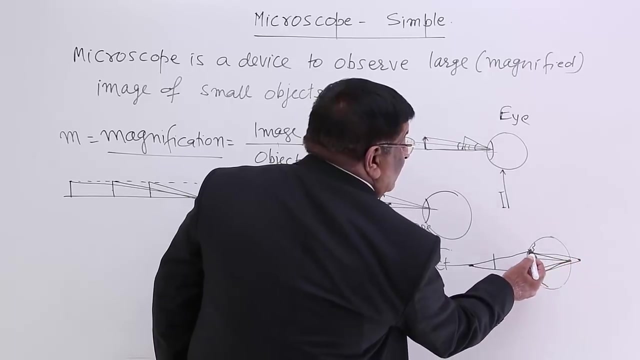 More clear, much less More clear, much larger. Here I see small, This is more clear, This is more clear, This is more clear. Bringing closer, Okay So, but what is happening inside my eye? When I bring it closer, from this distance to this distance, the image goes out, and immediately. 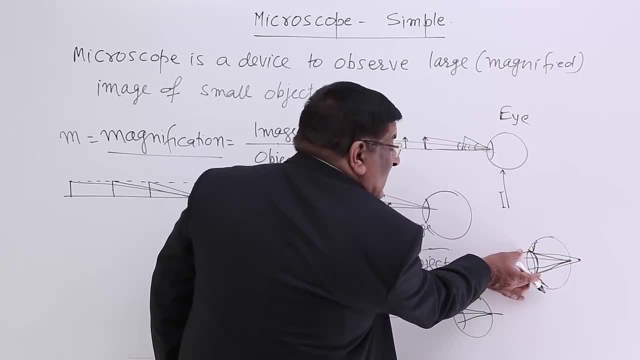 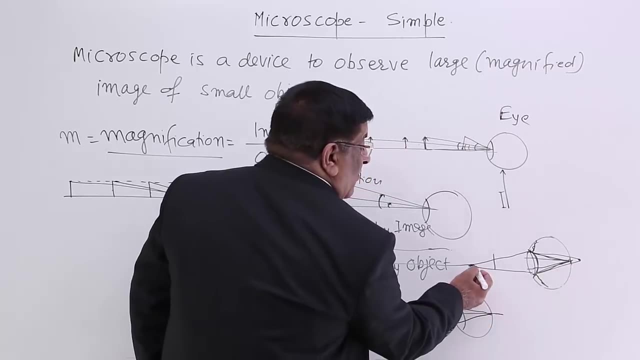 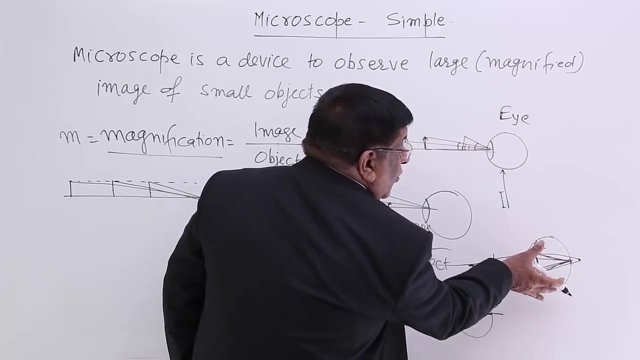 these ciliary muscles. they press this lens, increase its power and again it goes away And again they focus on the retina. Now I bring it here. If I bring it here, this angle is again more And it needs more power to focus on retina. 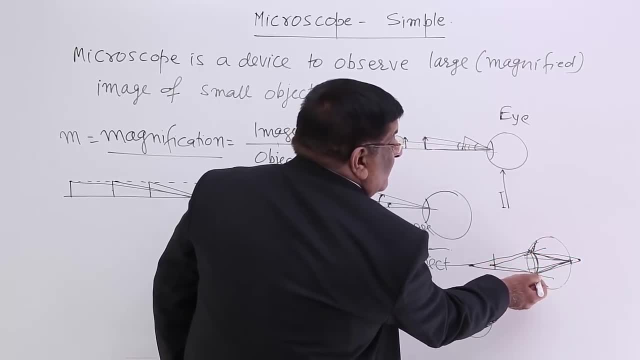 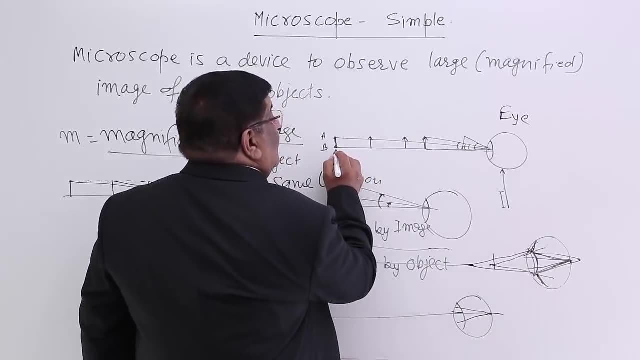 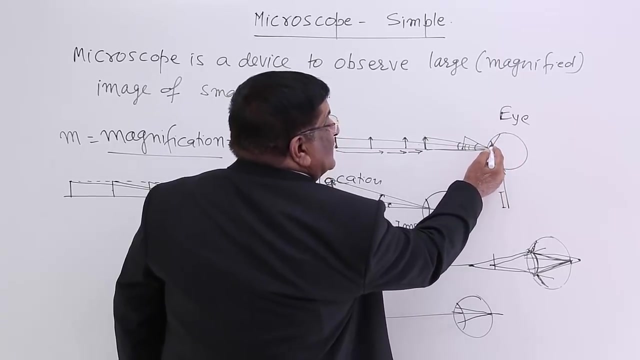 So ciliary muscles press more, The power is increased And they meet here. In the same way, if we bring it from a very large distance, closer, closer, closer, Ciliary muscle keep on pressing the lens. pressing the lens, increasing the power, increasing the power, increasing the power. 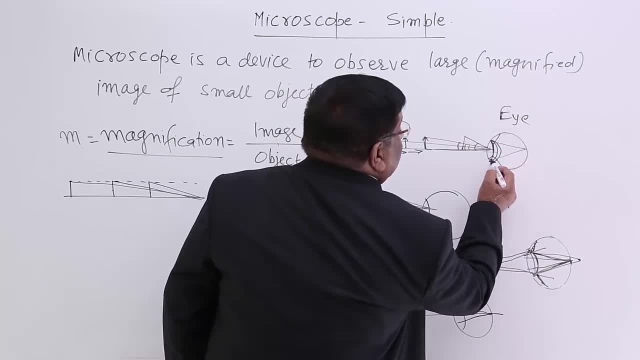 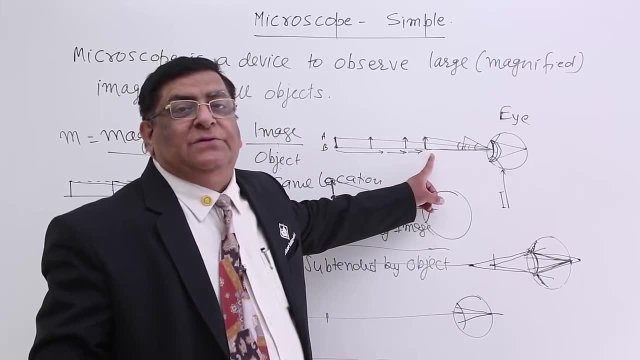 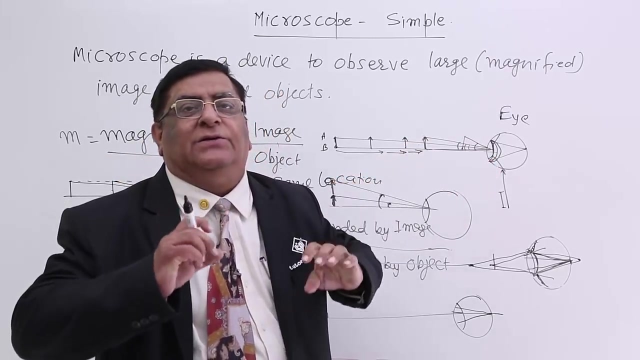 So that every time the image is made on the retina, Now what happens At a particular distance when it comes, it is very clear. But the ciliary muscles have compressed the lens to their maximum power. Now, if I compress it, 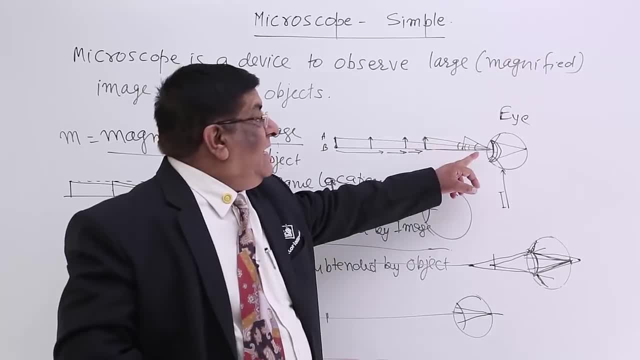 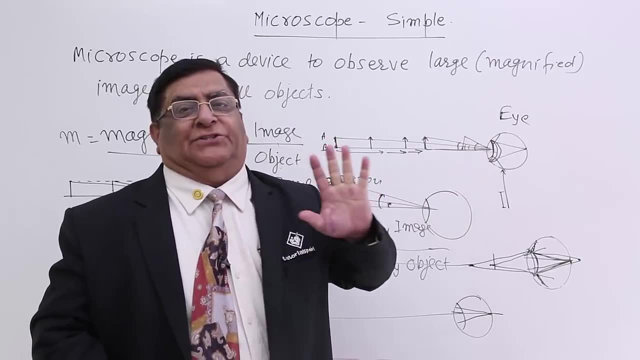 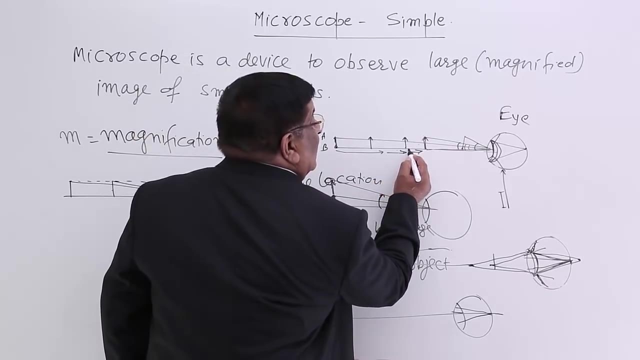 any more. if I compress it any more, it is not possible, Because ciliary muscles have applied their maximum tension. They cannot apply it any more. Then what will happen? I am making it clearer, clearer, clearer. I bring it here: 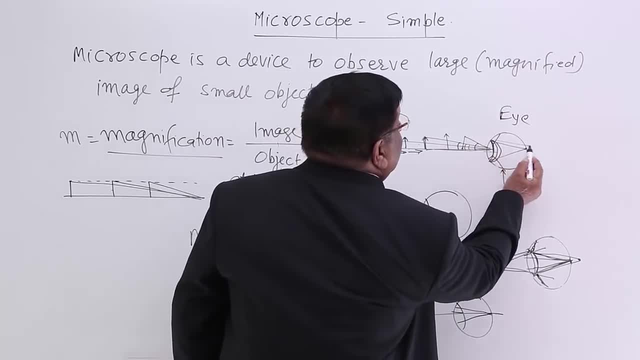 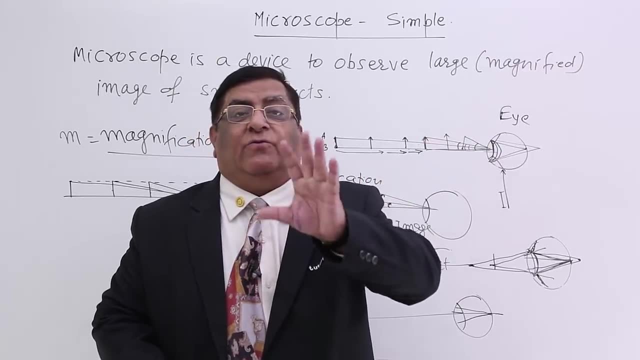 When I bring it here again, the image goes out And there is a signal from the brain: please press it more. Ciliary muscles say no, We cannot, Because we have already pressed it to the maximum. They don't do it. 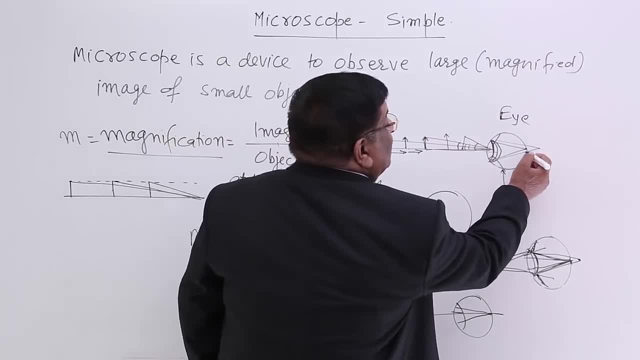 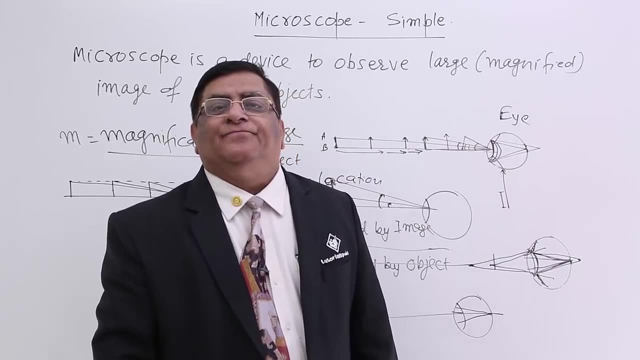 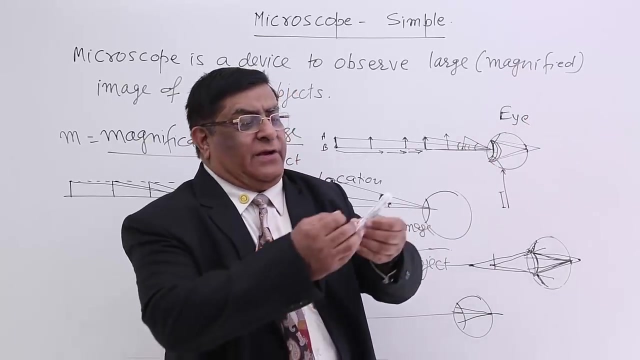 So now what happens? The image is formed here. There is no sharp image here. If there is no sharp image here, I can't see it clear. Okay, You have seen this, You can read this. It is far away. It is a very small writing. 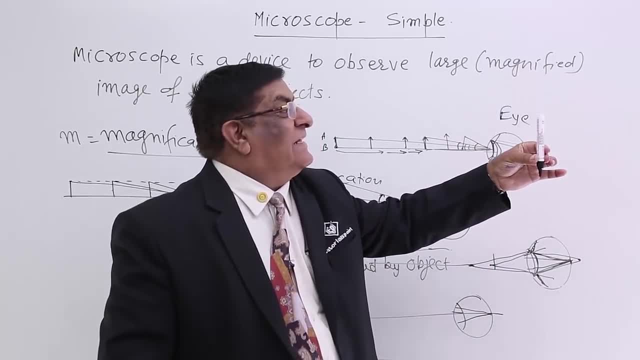 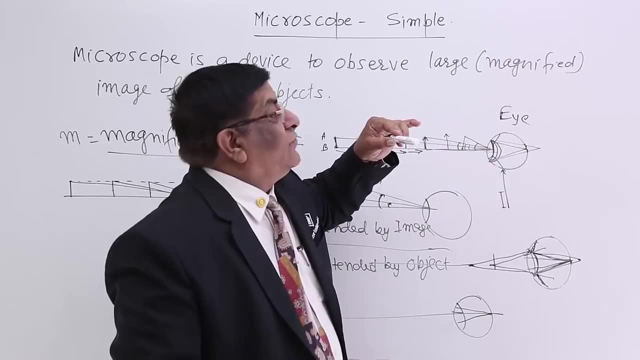 I am not able to see from this distance. I bring it closer. It is clearer, Closer It is clearer. More closer, It is clearer, Clearer, Clearer. So what I find bringing closer is making it clear. So I bring it like this: 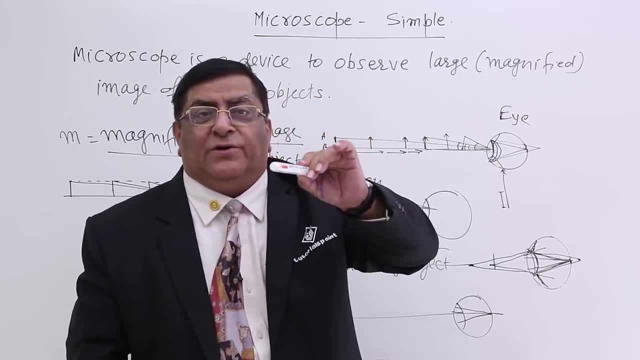 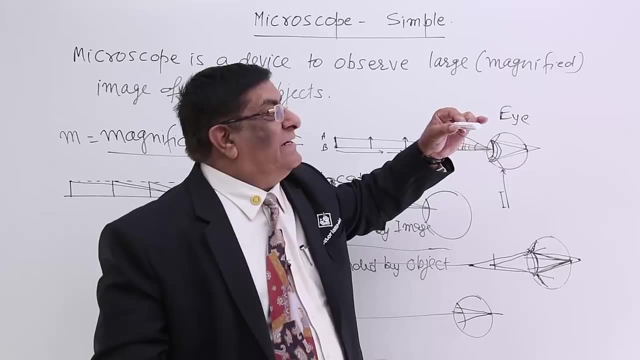 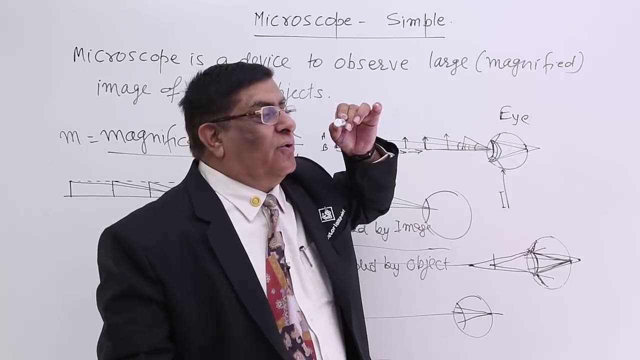 And now I am not able to see this. Why I am not able to see this? Because my ciliary muscles were adjusting my eyes, This Increasing the power, Increasing the power, Increasing the power. They have stopped increasing the power. Now, if I bring it more closer, they stop working. 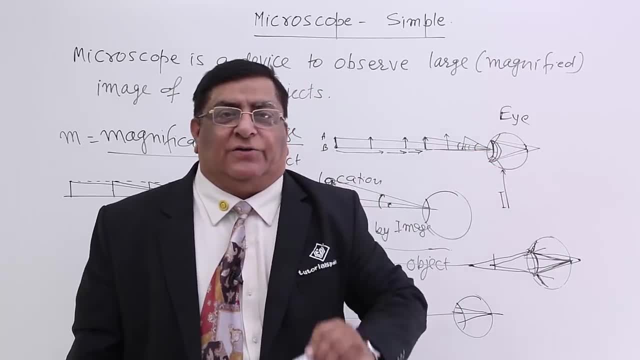 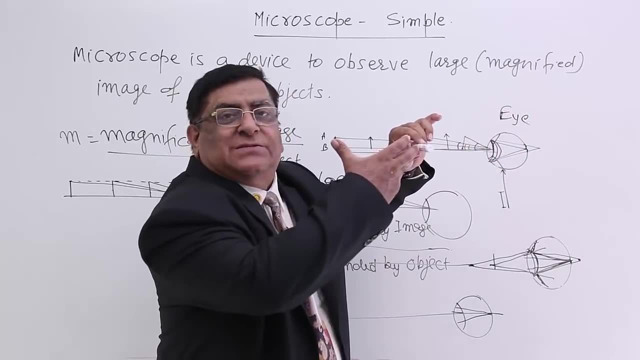 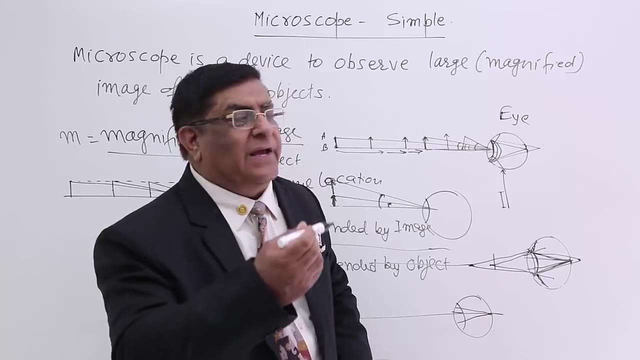 And this goes out of the eyes. I cannot see it. So I can see the things more and more clear up to a distance. After that I cannot see. So there are two actions taking place. One, when I bring an object- infinity- to this distance. 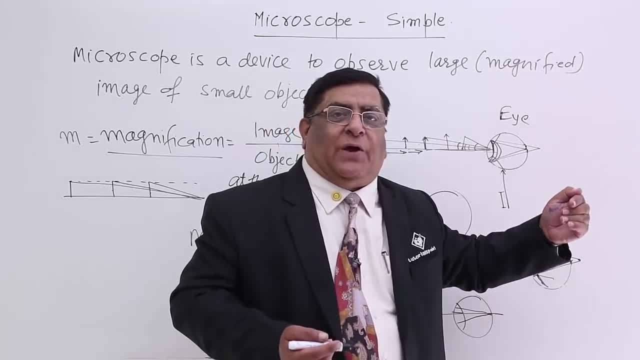 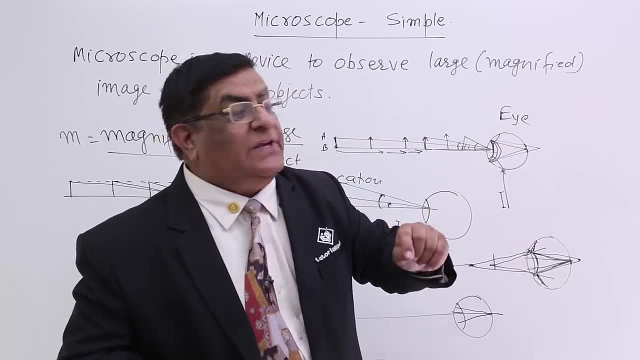 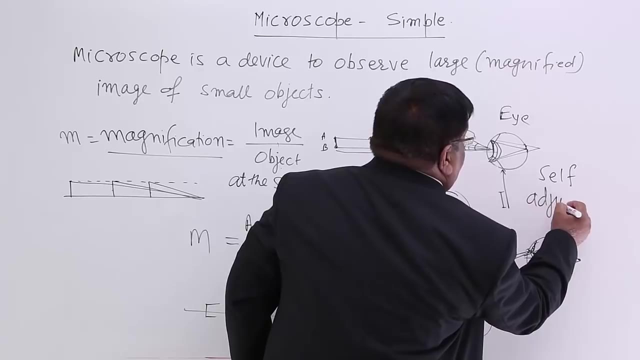 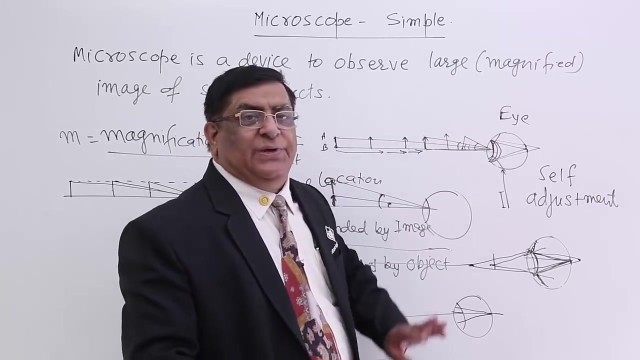 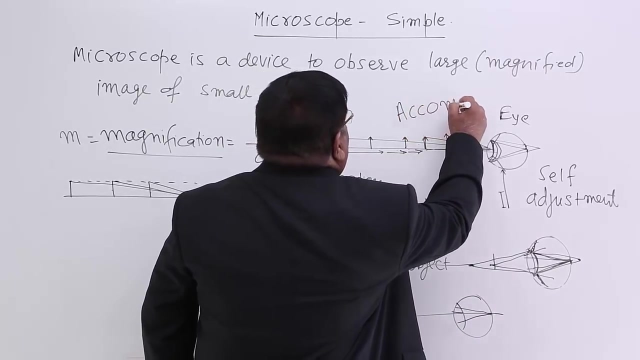 The clarity goes on increasing Because the focal length of my eye is getting adjusted according to the distance. This feature of the eye is known as self-adjustment. Self-adjustment: That eye is doing it. Or a better technical name for this is accommodation. 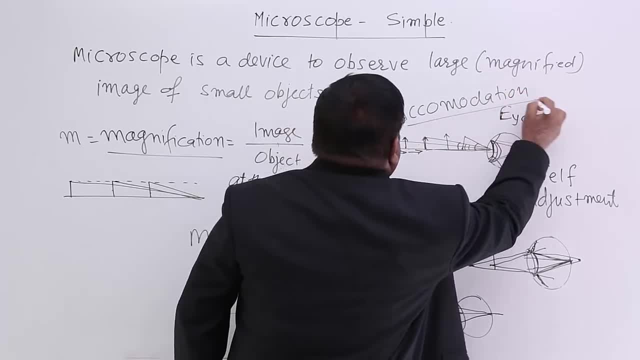 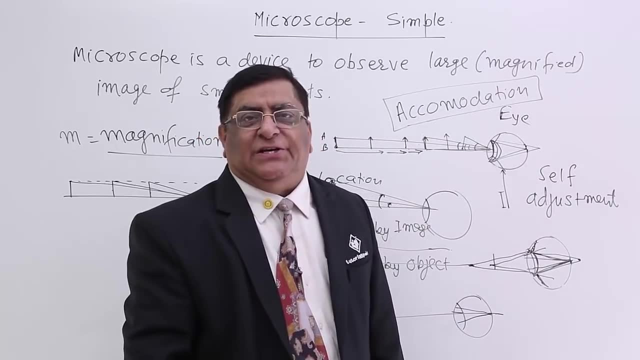 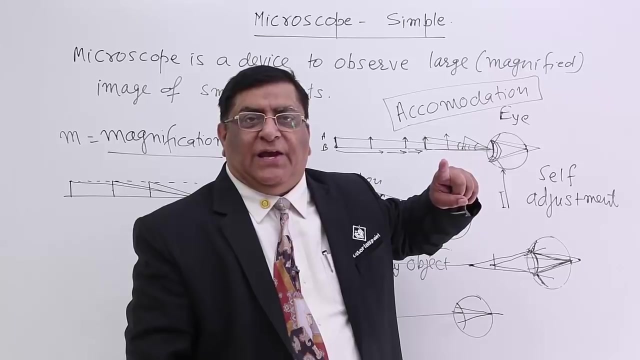 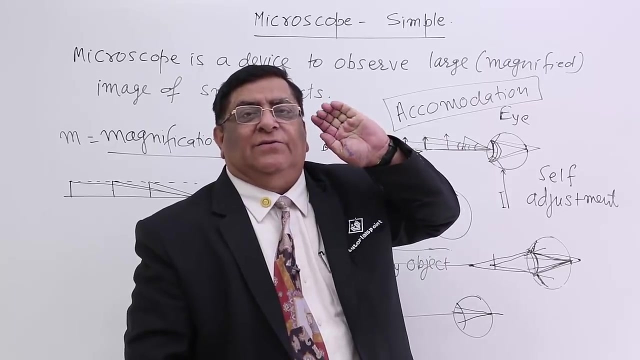 This is mostly used in physics. What is accommodation of the eye? Accommodation of the eye is a feature that it adjusts the focal length in such a way that, according to the distance of object, the image is formed on the retina. Image is formed on the retina. 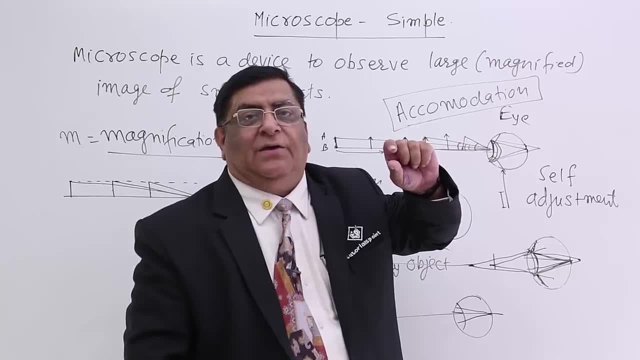 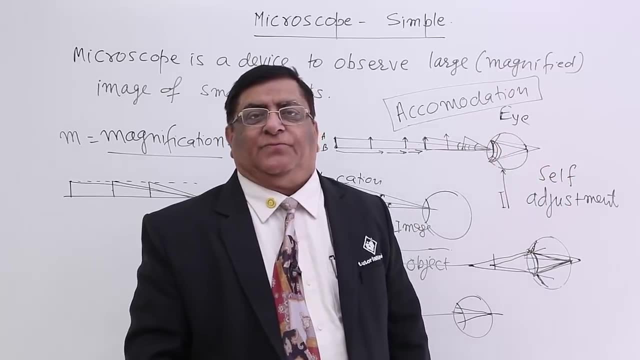 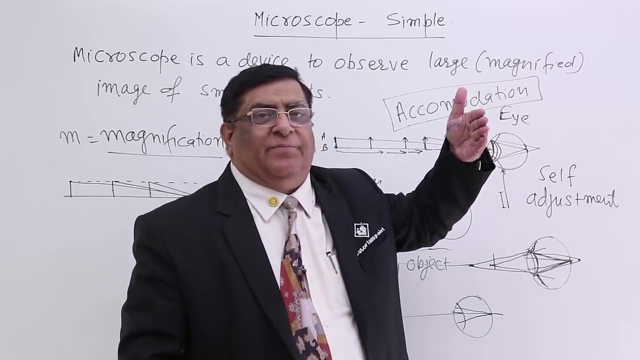 The focal length is adjusted in such a way. So This phenomena of the eye, This characteristic of the eye, is known as accommodation. Okay, Will the accommodation work for all the distances? Answer: no. It has come to a minimum distance. After that it will stop working. 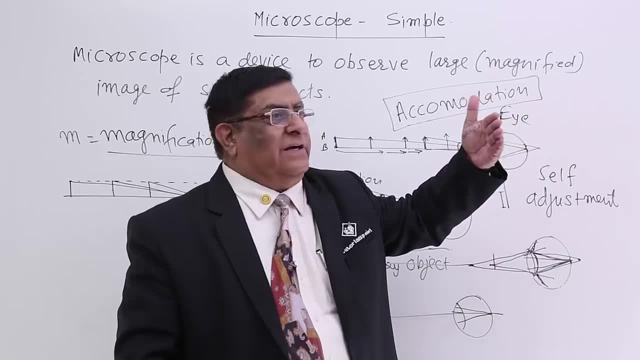 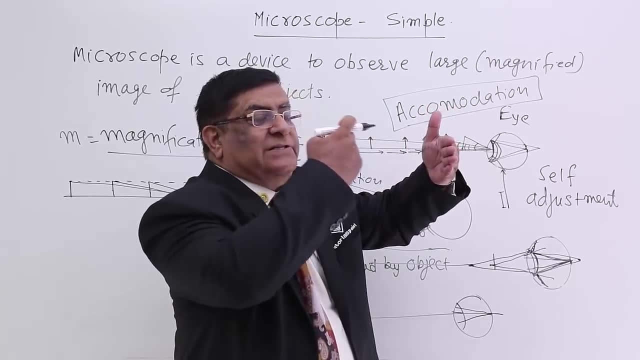 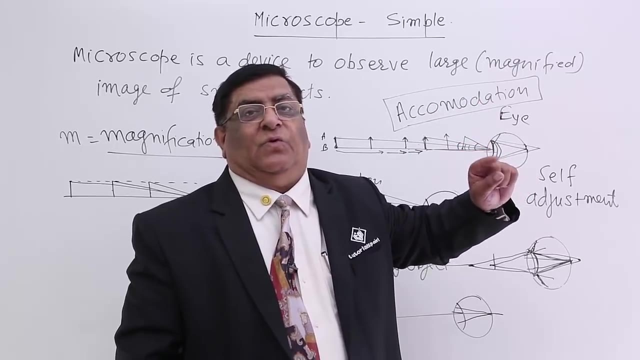 That means we are making it clear, clear, clear, most clear, And after that it has stopped working. So this distance is the least distance of the eye, The distance of clear vision, Distinct vision- What are the words we are using? 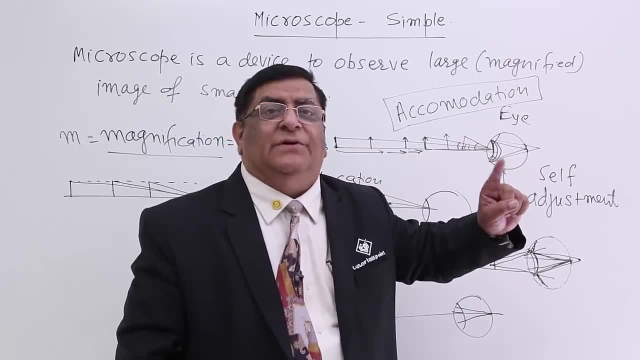 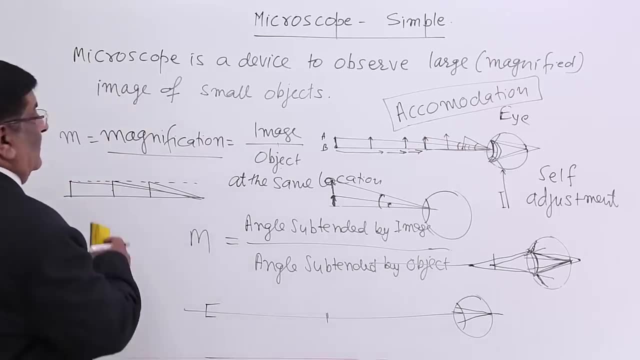 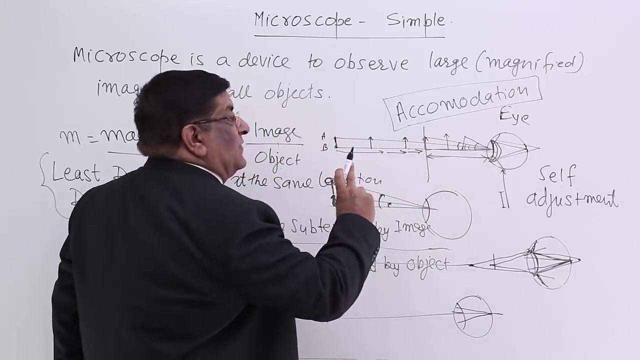 Minimum distance, or the least distance of distinct vision, And this is a very important distance, What we call it The least distance of distinct vision. This is the minimum distance from the eye where we have to put an object to see it clear most. 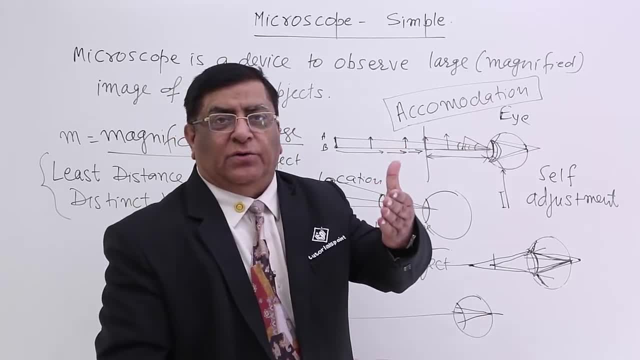 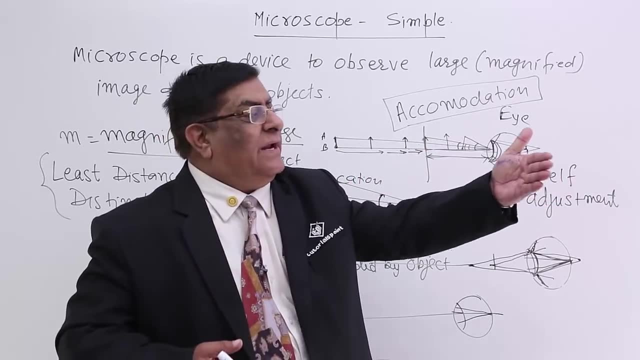 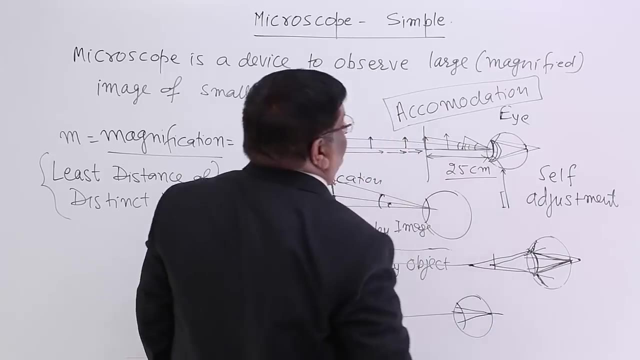 And this is normally we do. when we read a book, When we see our mobile, When we read any newspaper, Anything, We bring it to that closer And for a healthy eye, this is almost 25 centimeter. At 25 centimeter, I see the things most clearly. 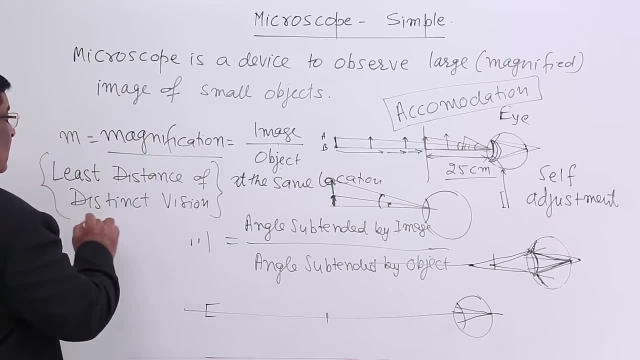 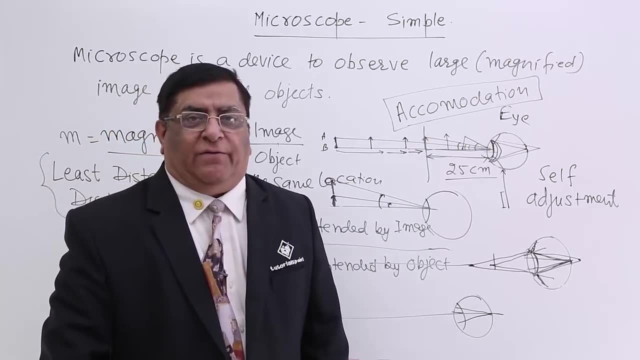 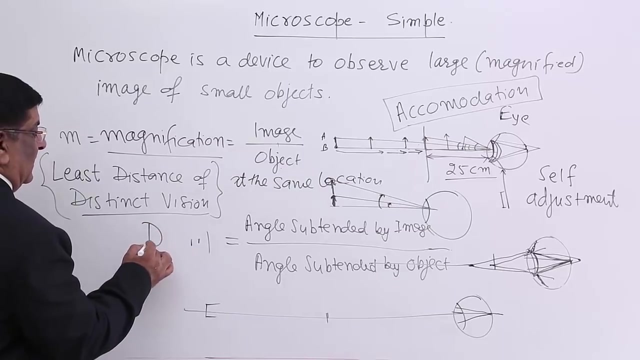 Okay, What is that Least distance of distinct vision? When I use this distance in our optical instrument, we do not write 25.. We do not write this long. We have put a symbol for this And that symbol is capital D: Distinct vision. 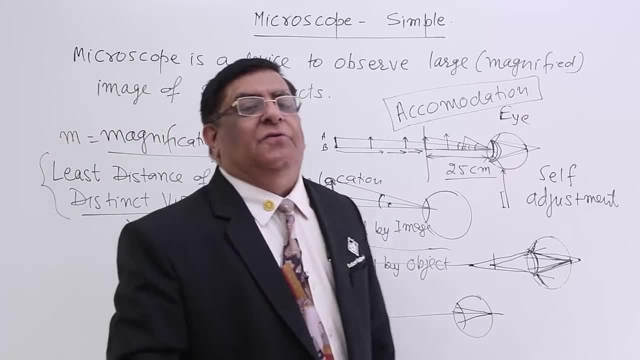 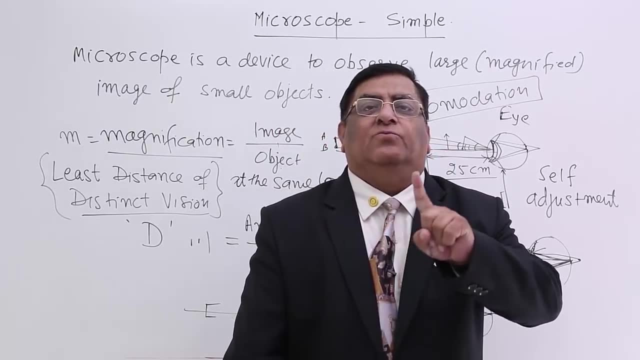 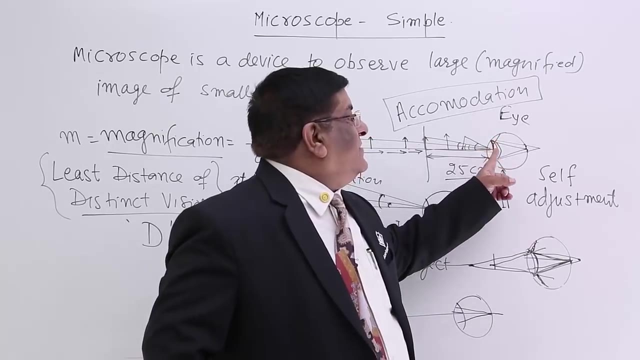 So this is the distance of distinct vision. We will keep on using it. At that point, everything will be most clear to us. But at that time, what is happening with the muscles? Answer: Muscles are under great tension. So when we keep a book very close to us, 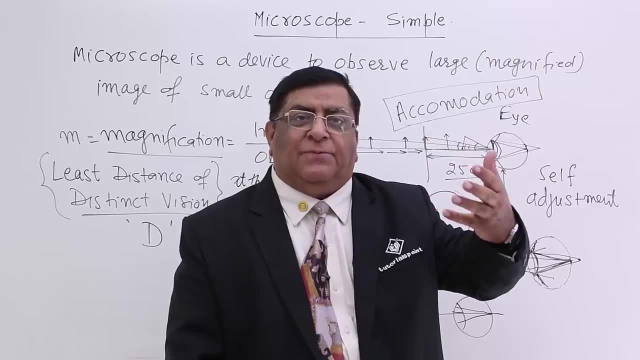 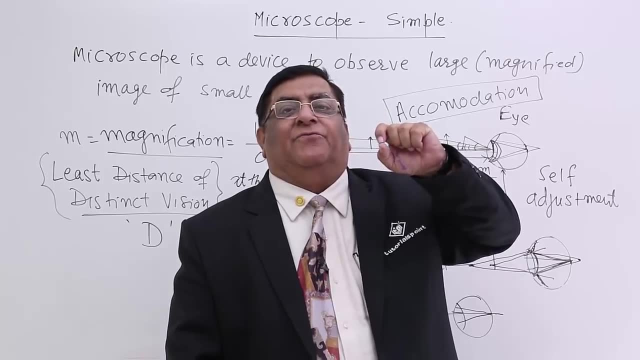 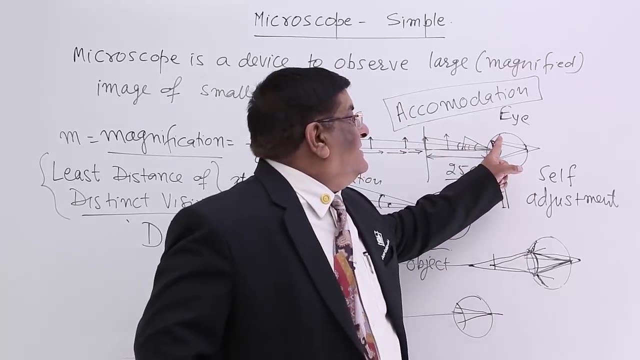 When we keep our mobile very close to us And keep working on it for hours, Then these muscles under tension, they have a fatigue And we say we are tired. There is pain in our eyes. That pain is in the ciliary muscles. 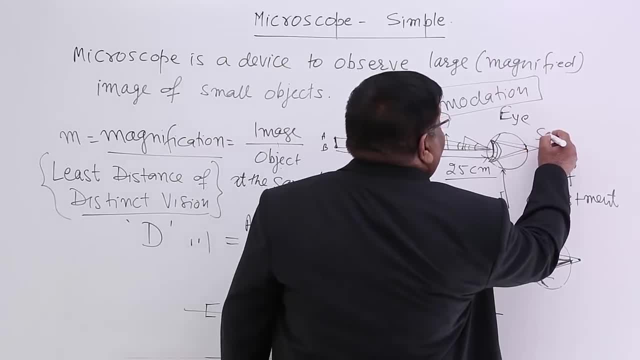 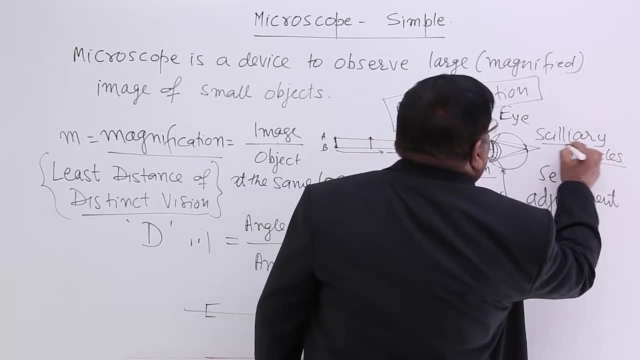 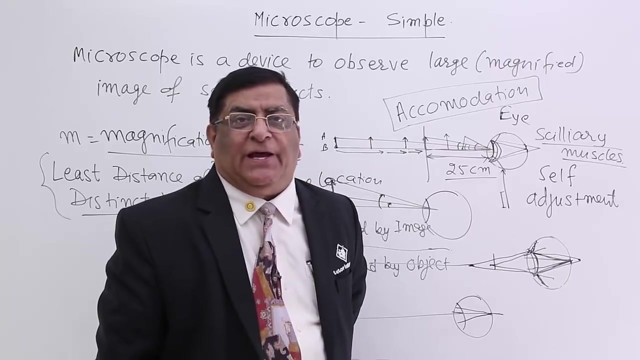 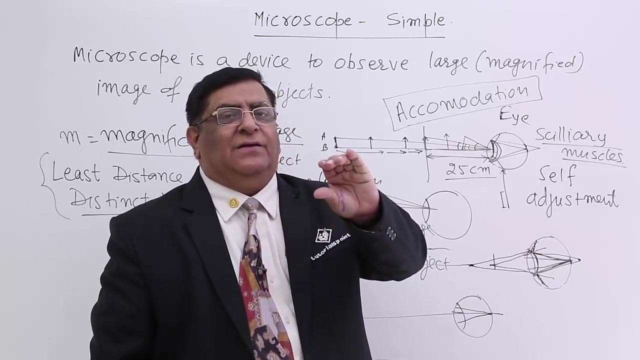 Okay, So I will tell you, I will tell you, I will tell you. They are under tension when we are seeing the things clearly. Is there any remedy for that? Yes, There is a remedy. We can see the objects little, not so clear. 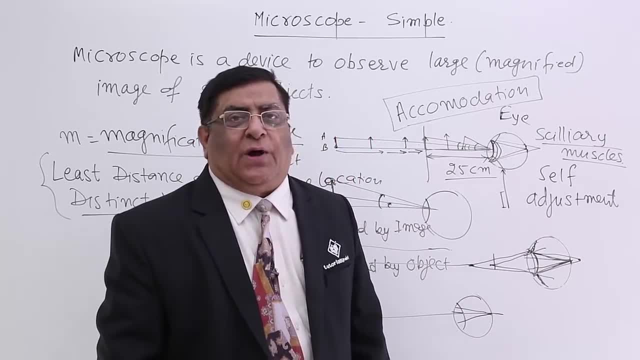 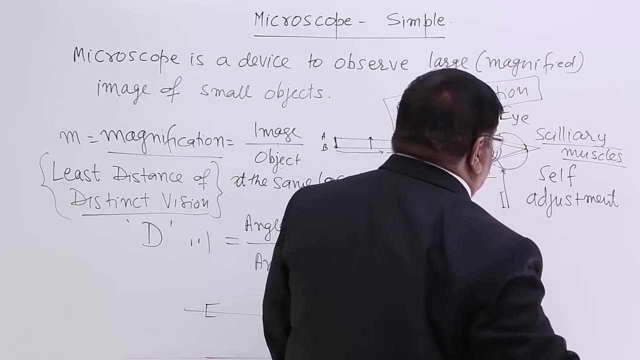 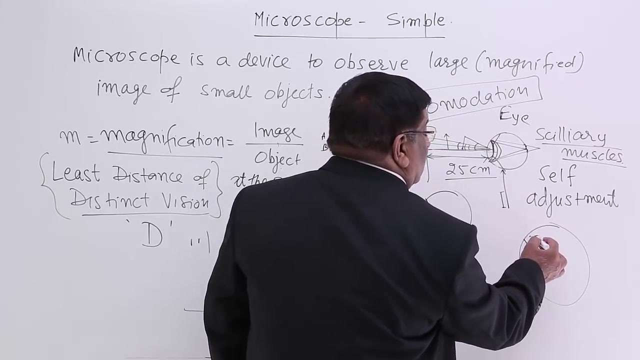 Little less If we allow the rays to come parallel. If we allow the rays to come parallel, Then what will happen? Our eyes natural setting is for parallel rays. That means No pressure by the ciliary muscles. Ciliary muscles are relaxed. 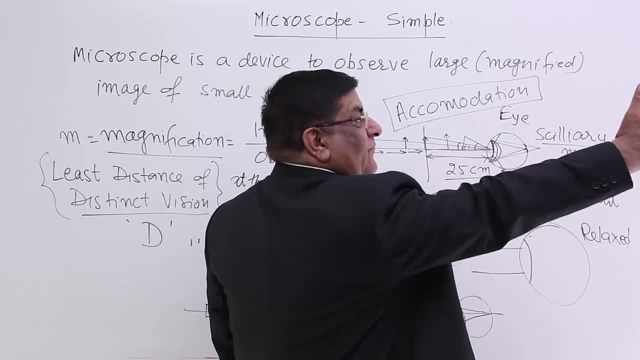 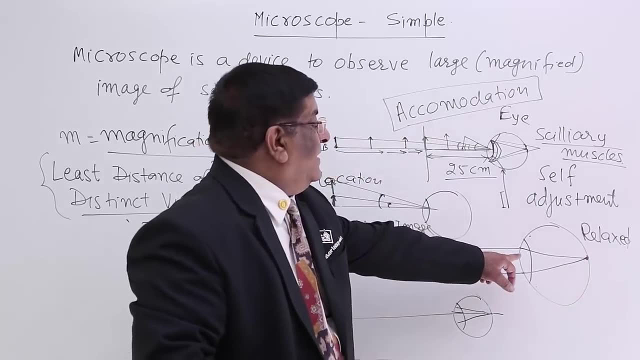 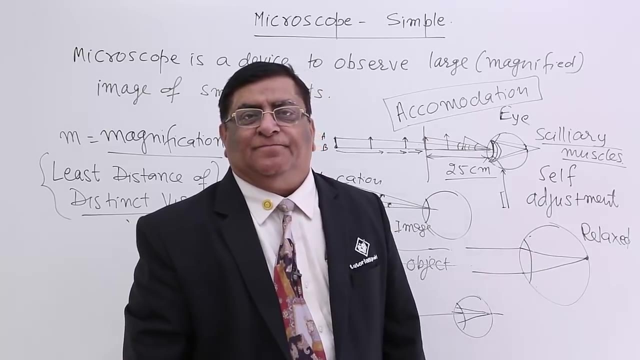 So parallel rays are coming from far away object: They will meet automatically at the retina. This is natural setting of our lens. How much is the tension on the ciliary muscles? Zero, No tension. Now, if somebody ask me to work in this situation for few hours, 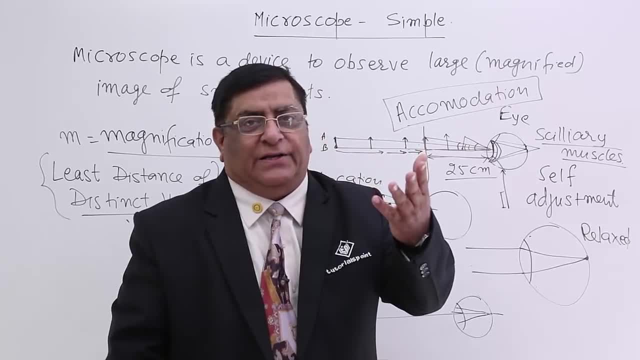 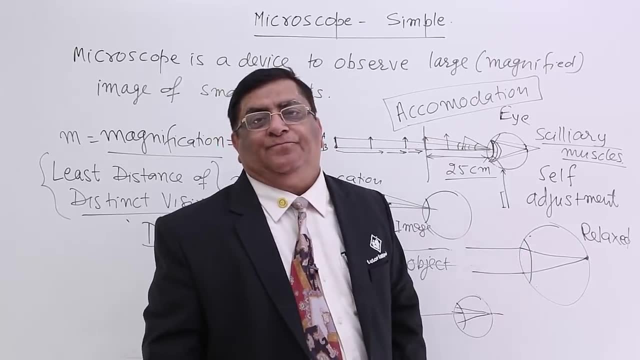 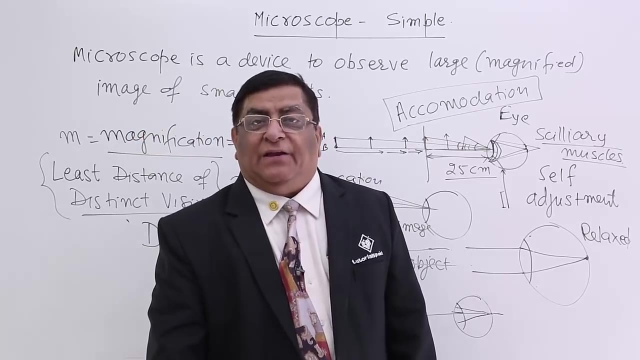 I can work. There will be no fatigue, There will be no tiredness in the eyes, So this is a very comfortable state of work. Now we see the objects magnified. We can see the objects magnified. We can see the objects magnified large in two settings of our optical instrument. 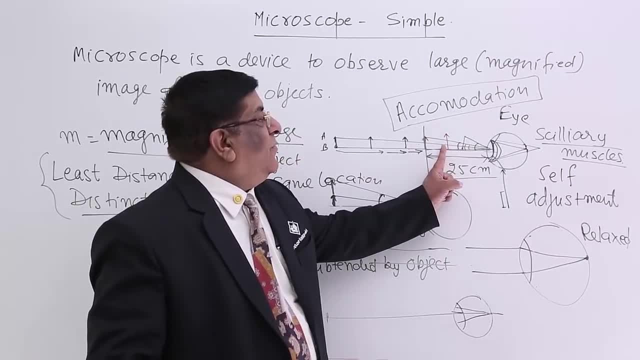 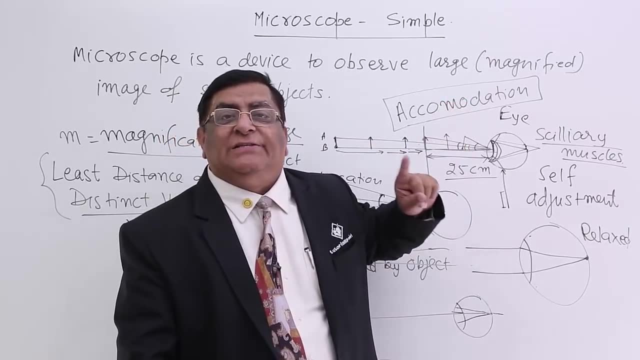 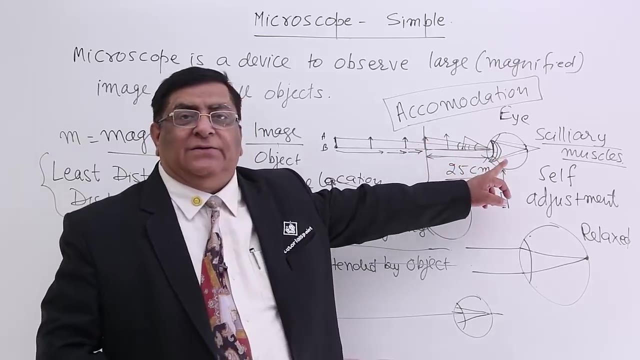 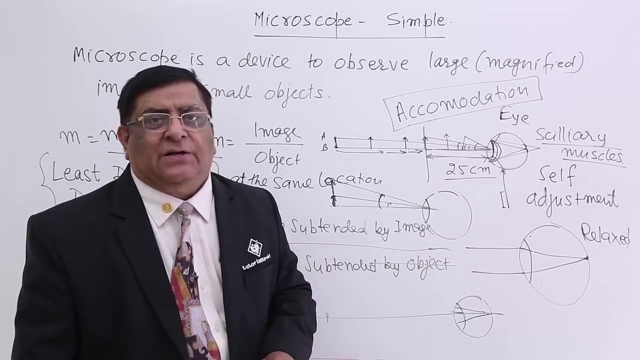 One setting is for this setting: When we have brought the image so close that it is most clear, Where is the image? at that time The image is at D. At that time it is very clear, But the eyes are under tension. The second setting is when we allow the parallel rays to enter the eyes and still there is a magnification. 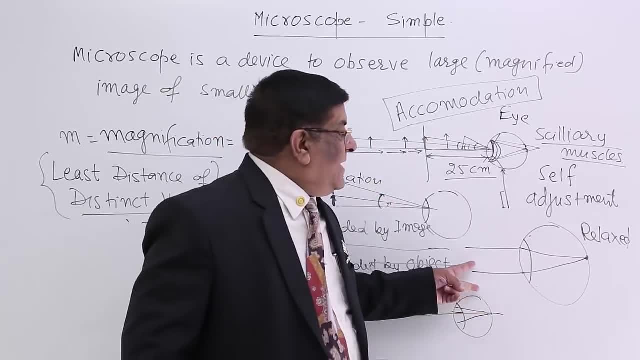 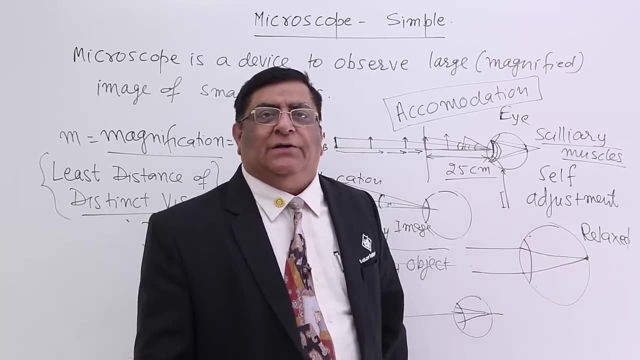 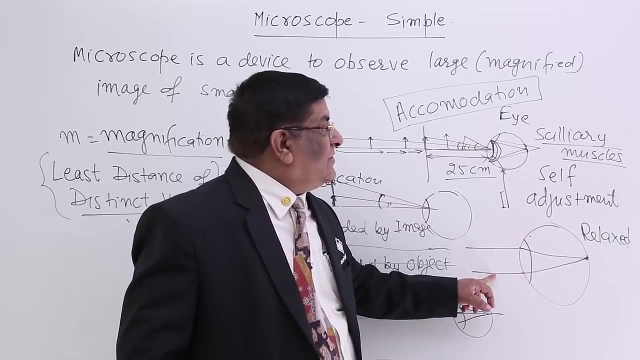 It is large, but the rays coming are almost parallel. There is no fatigue And we keep on working on it. So at this time the magnification may be little less. How much is the magnification in this situation? How much is magnification at this situation? 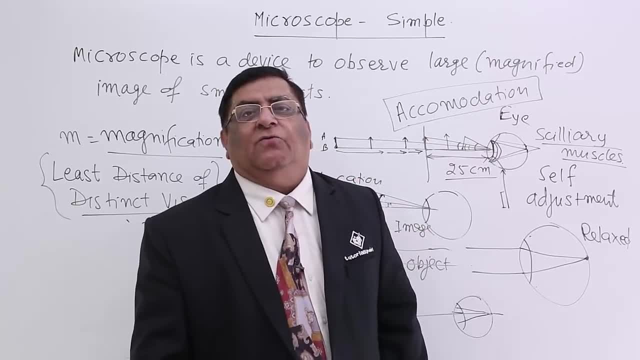 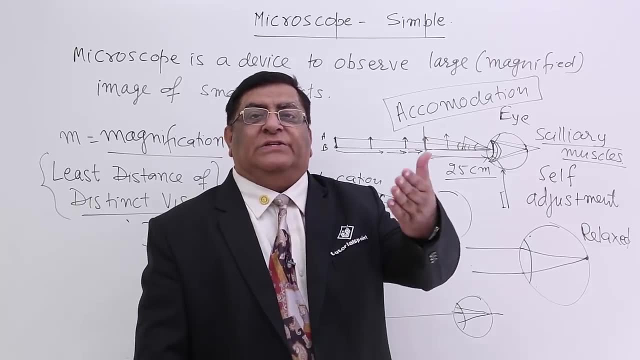 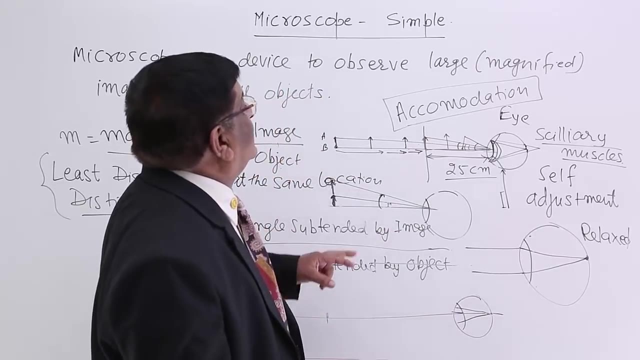 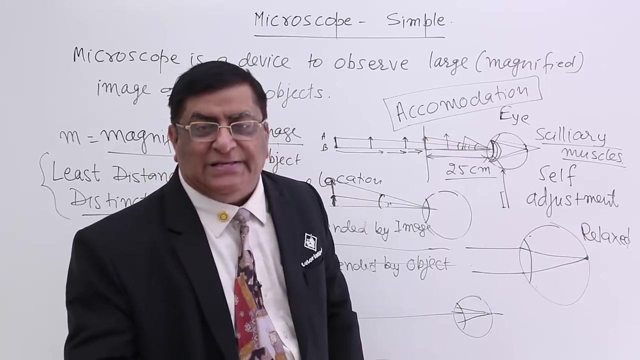 Both we are supposed to calculate when we are studying about optical instruments. So this is about how we see the things in two settings. Now we come to our original topic, and that is simple microscope, which is made by a spherical lens, that is, a convex lens. 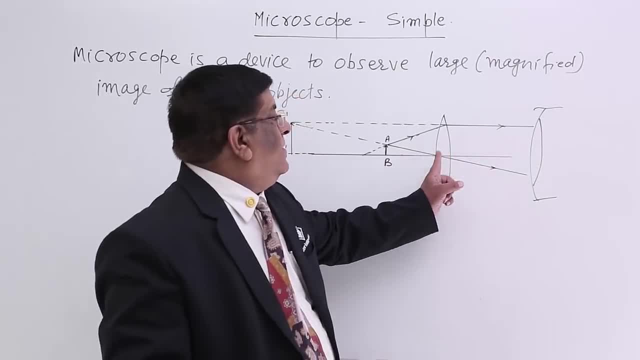 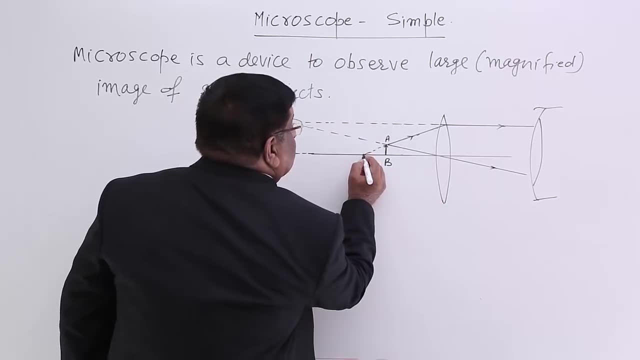 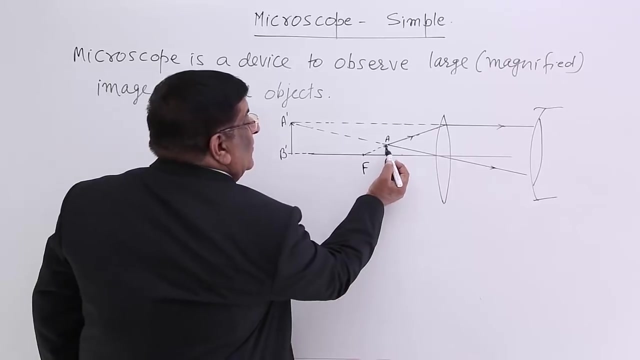 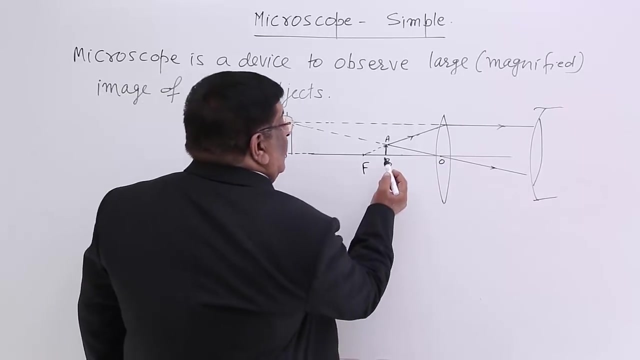 See, here is the lens- Convex lens- we are going to use as microscope. This is focal length on this side. F, focus: We have placed an object between focus and optical centre. anywhere From B there are rays on the principal axis. 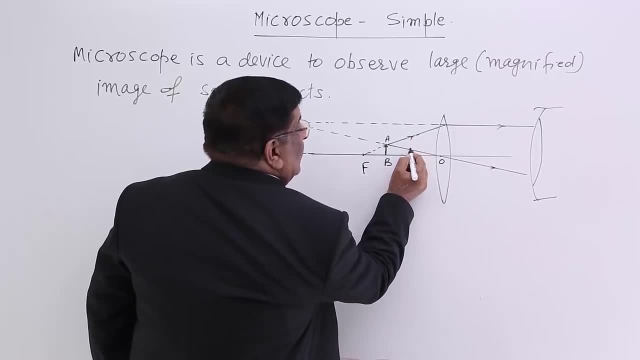 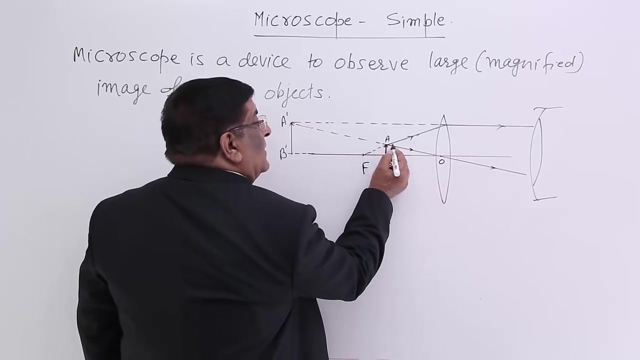 From A. we take the two rays. One ray, which is going in the direction of optical centre, will go and deviate it and enter our eyes. Other, we take one ray which is coming from the direction of focus. It starts from here, but which direction we have taken? 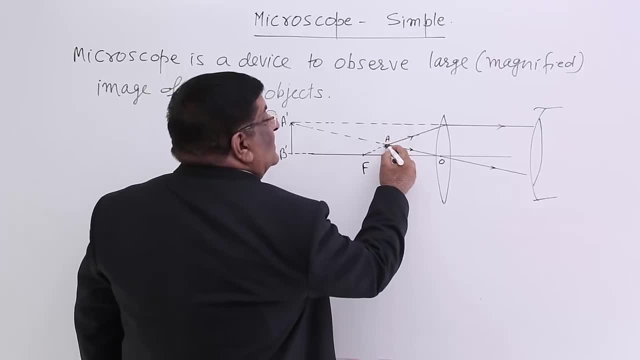 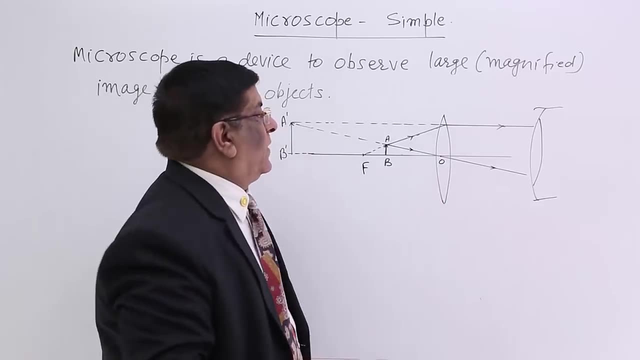 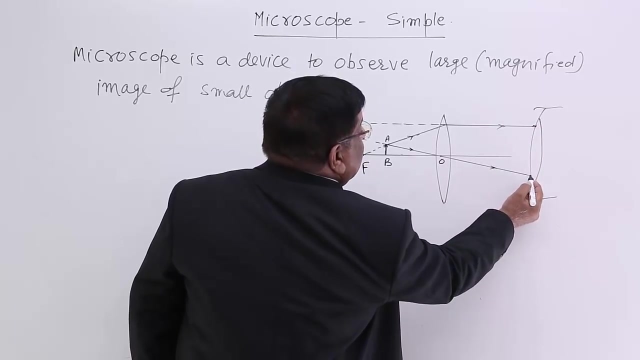 The one which is along the focus, So that this ray, after refraction, will become parallel to the principal axis. That is the rule we have studied. Okay, So this becomes parallel to the principal axis and enters the eyes. This also enters the eyes. 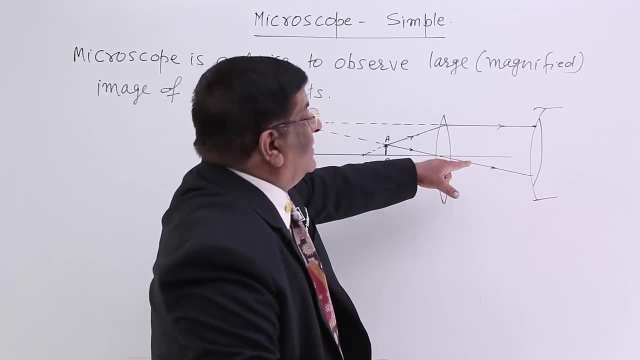 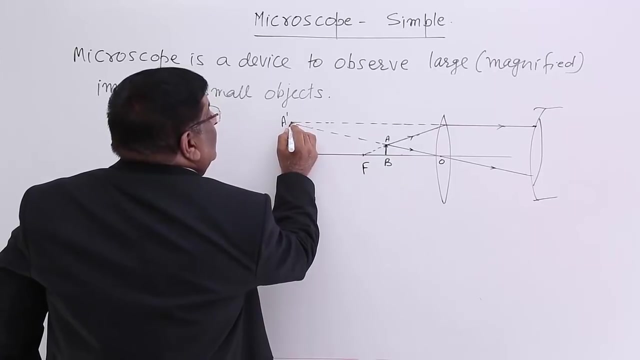 Now these two are diverging. They never meet each other. So where is the image? formed Eyes backtrack it and backtrack this, And it appears to us that both are coming from this point. So this point, we see the image of A at A dash. 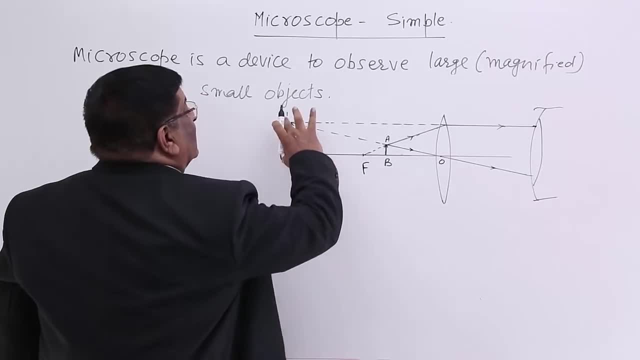 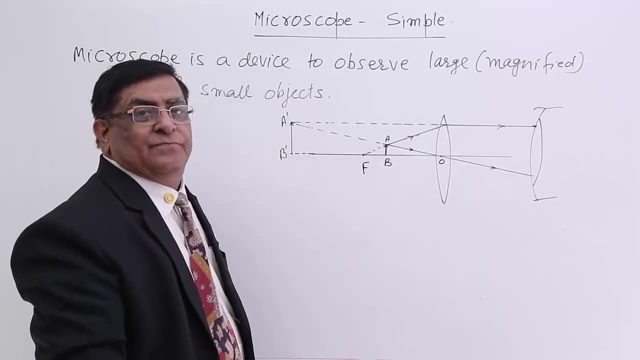 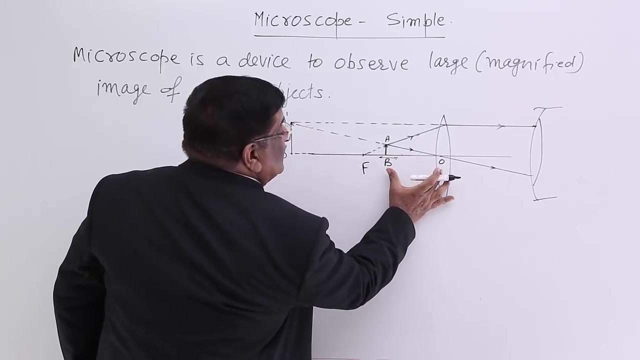 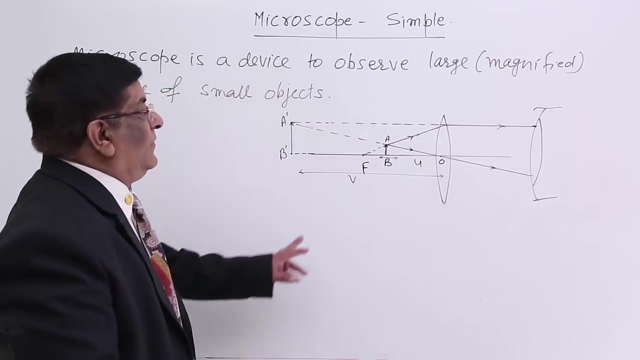 B on the principal axis at B dash, and this A dash, B dash is the image And you are seeing this is larger. Now if we move it here or here. This way, if we are changing U, then we are changing V, So U and V can be changed. 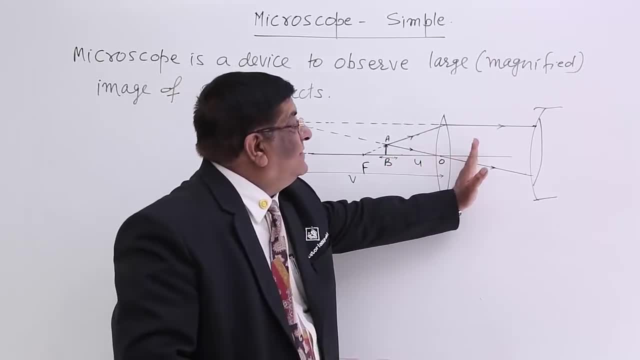 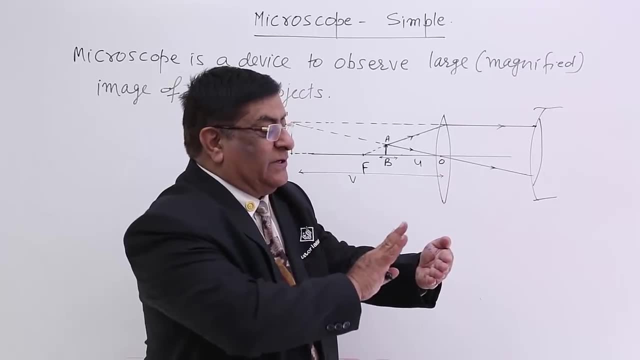 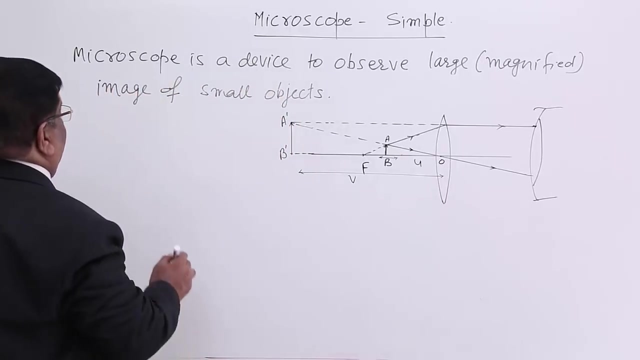 By simply moving this lens this way. If we keep an object here, put the lens here and move it this way, What we are doing- We are changing U according to V- will also change. Now, what is the magnification? Magnification is? we have studied for spherical. 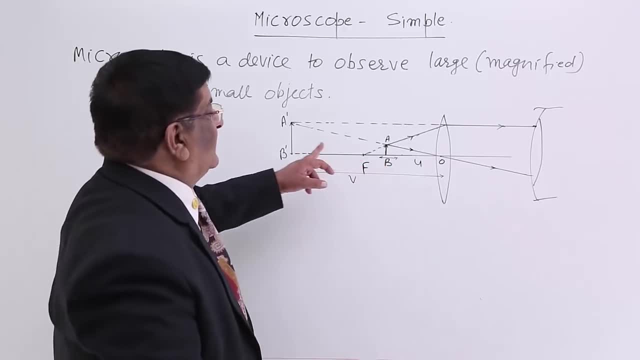 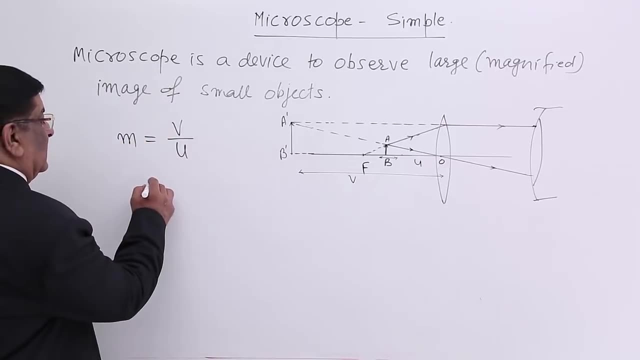 It is V upon U. Both are on the same side. V upon U is the magnification. Now we know another formula. that is, 1 upon V minus 1 upon U is equal to 1 upon F. Let us multiply this formula with V. 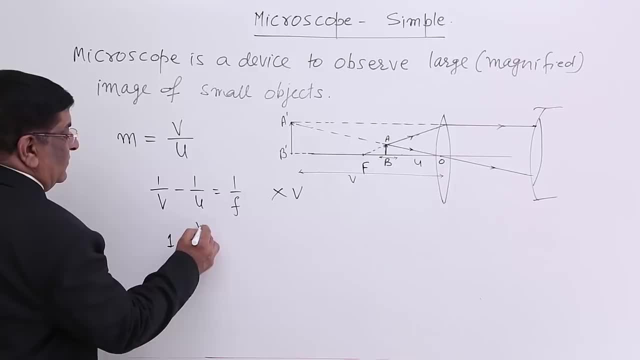 So this will be: 1 minus V upon U is equal to V upon F. Now, what is this V upon U? This V upon U is magnification. So this we take on this side and this we take on this side. So what do we get here? 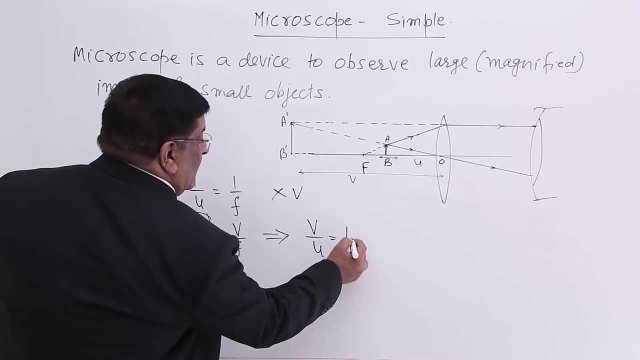 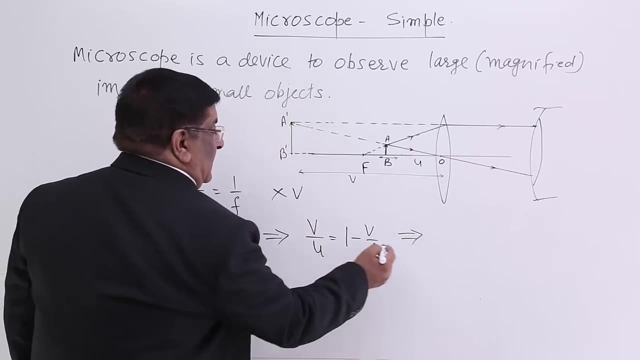 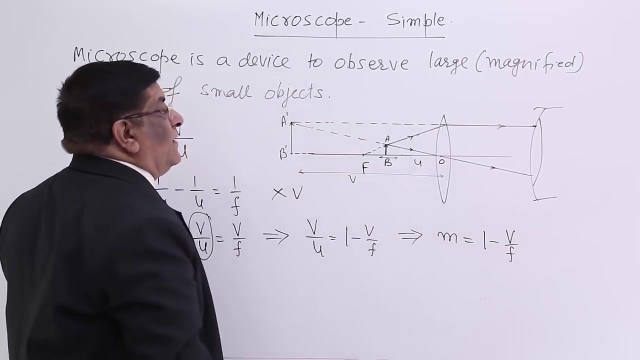 V upon U is equal to 1 minus V upon F, And this leads to- this is magnification Magnification- is equal to 1 minus V upon F. Now we adjust this U in such a way that this image is formed at a distance d. 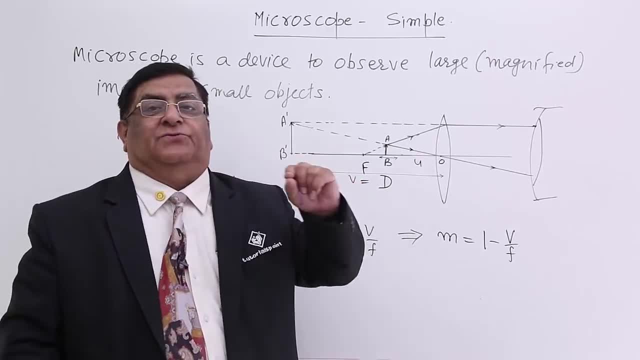 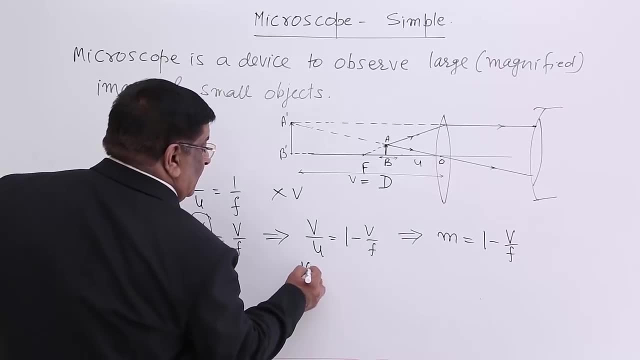 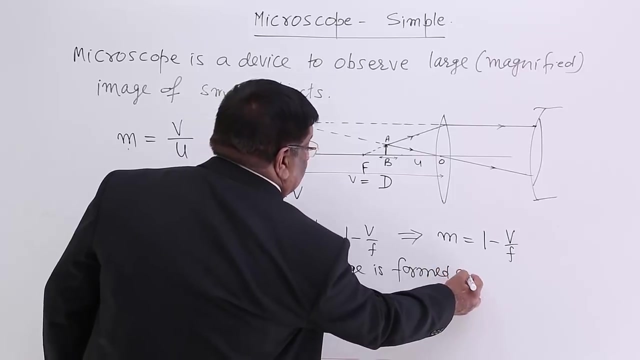 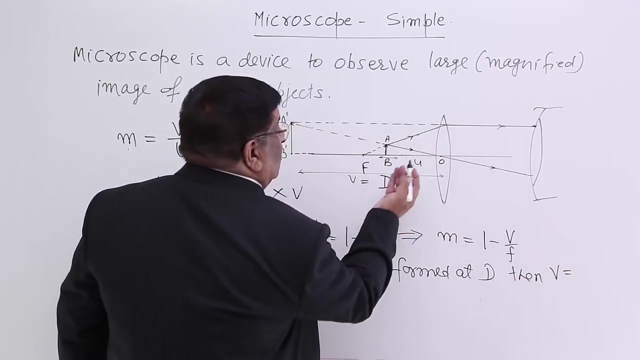 Why? Because at d. this is very distinct for us, very clear for us. So if image is formed, If image is formed at d, Then V here is equal to d on this side. That is minus d, Because d is on this side. 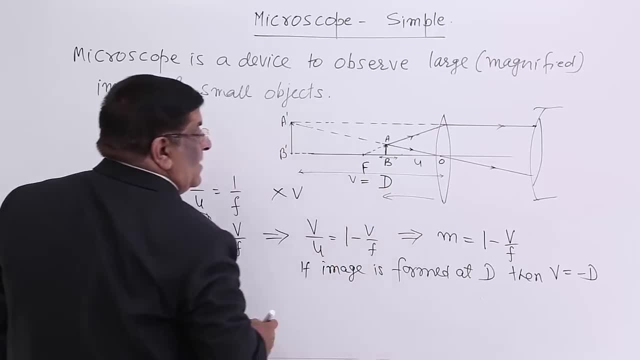 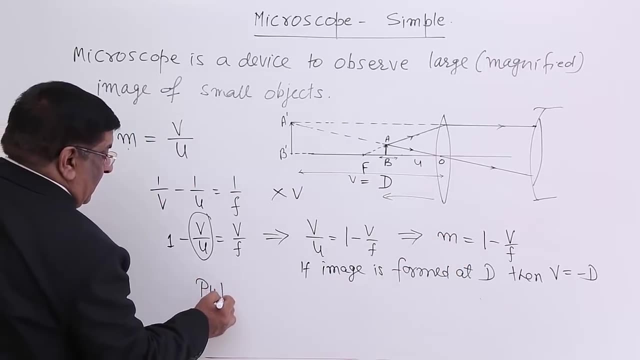 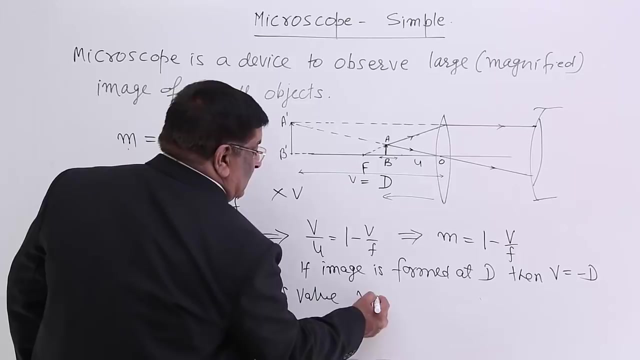 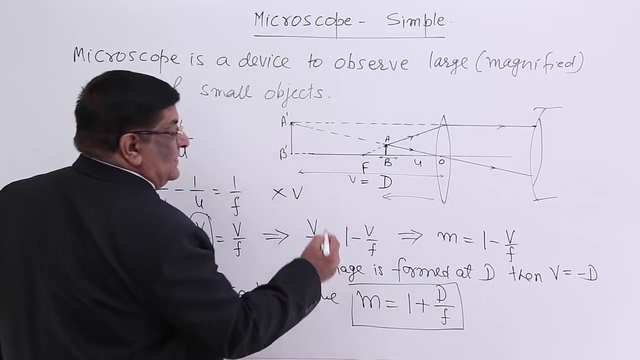 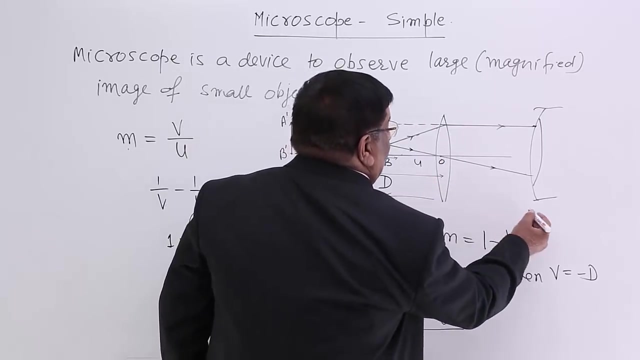 So this will be minus d When we put the value. Putting that value here, Putting this value, We see magnification is equal to 1 plus d upon F. This, This is the magnification formula for this simple microscope. This is a simple microscope. 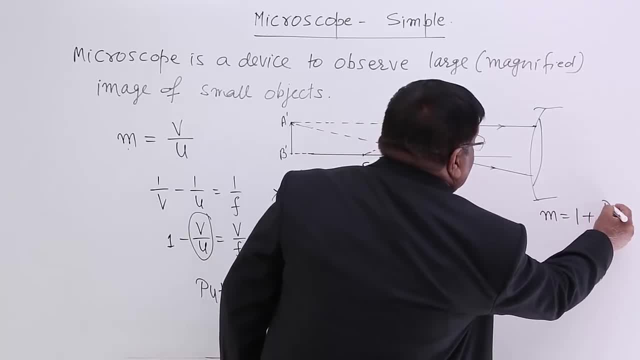 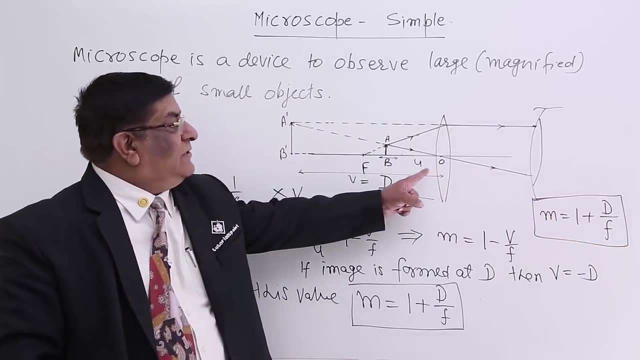 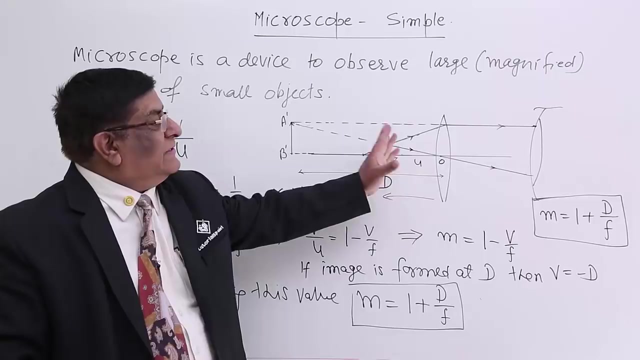 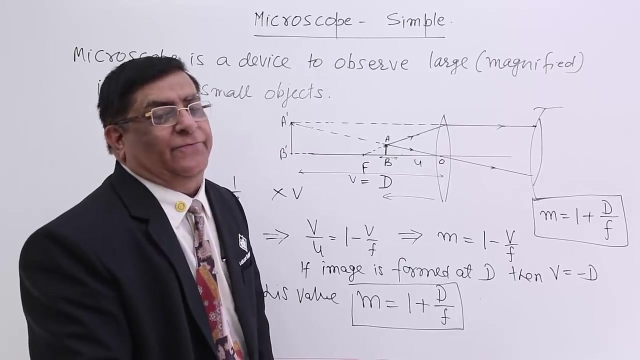 So remember, M is equal to 1 plus d upon focal length of convex lens We are using And how we use it. We keep the object below under focal length, Then it works as a microscope. And this is the magnification: 1 plus d upon F. 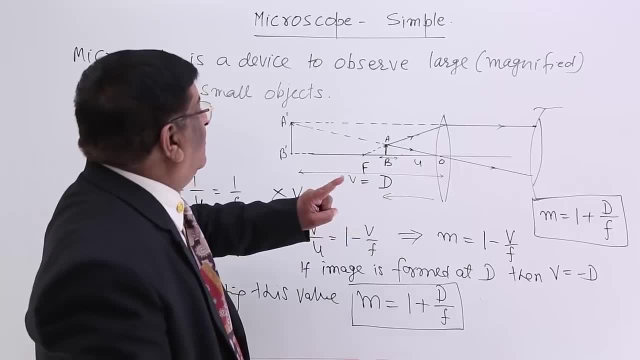 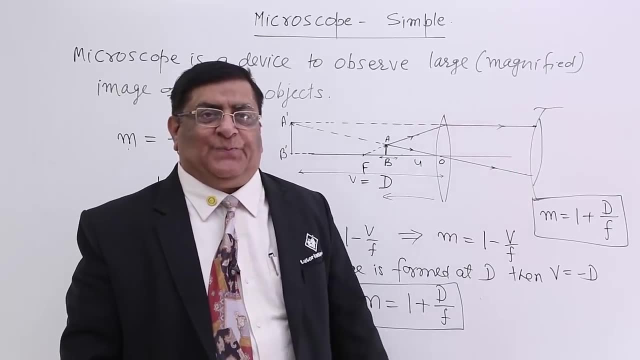 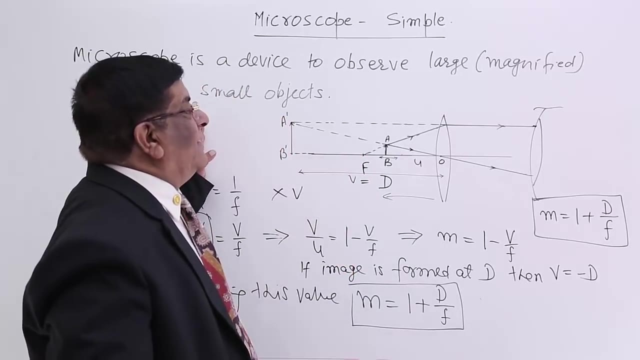 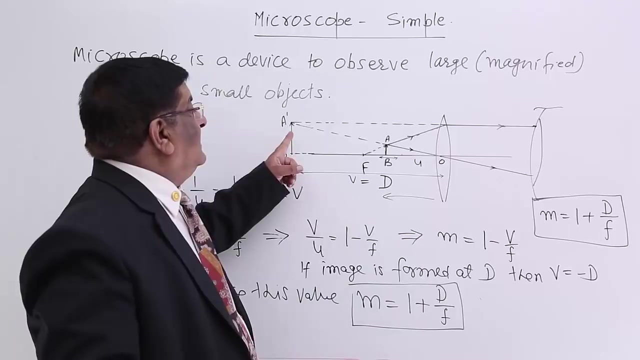 Now this is a setting when we have made the image at distance d, Naturally eyes will be under tension. Now suppose We want that This image, Let it be away, No problem. But we want to be relaxed, So we want these rays to come parallel. 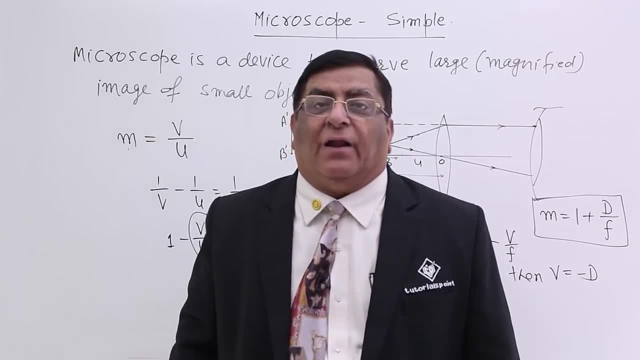 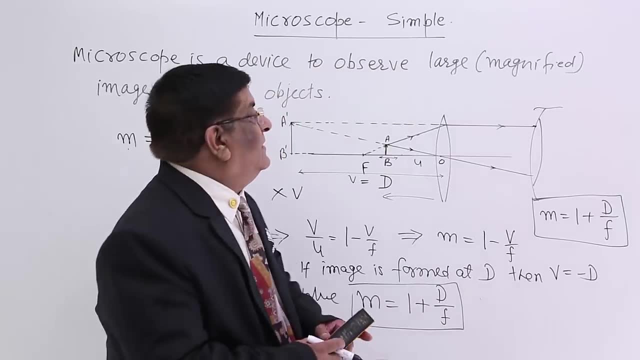 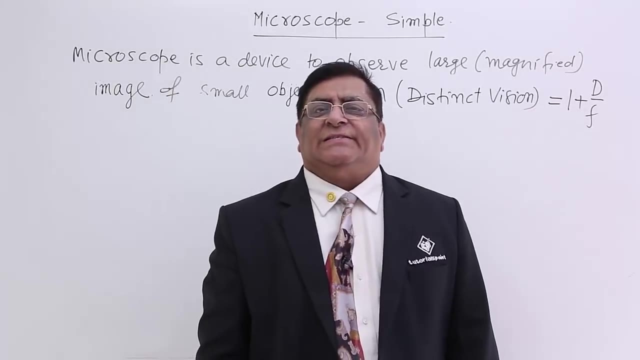 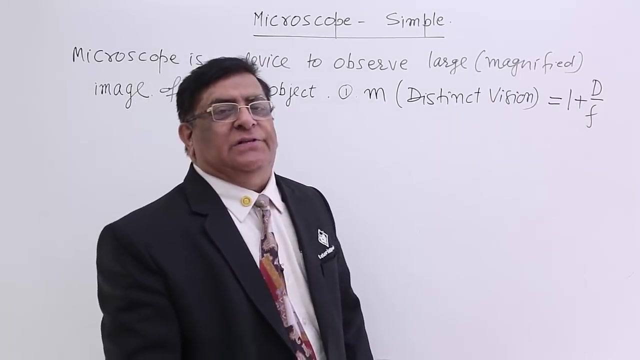 That we will say setting for parallel rays, Or we give it a name setting for relaxed eyes. So setting for parallel rays. See, We have seen one setting of simple microscope And their magnification is 1 plus d upon focal length. Now we will see the second setting. 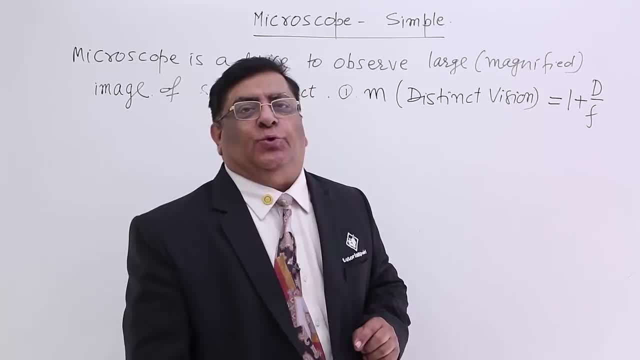 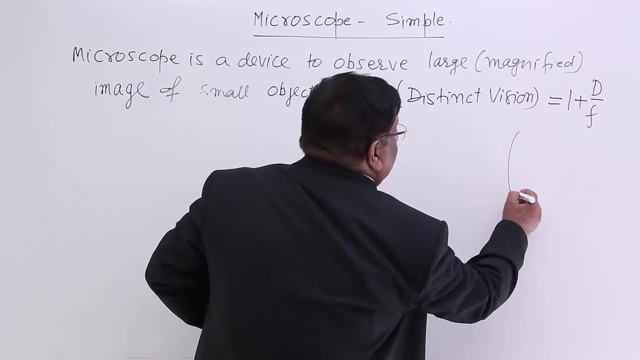 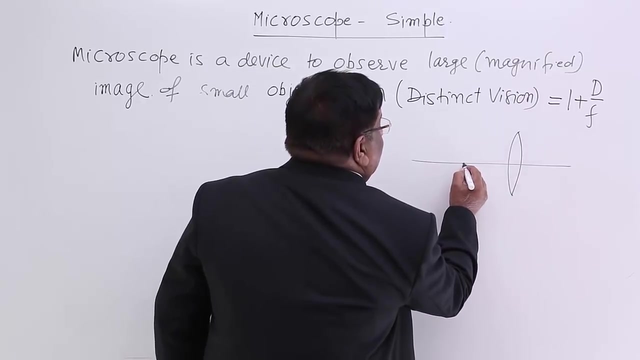 In the second setting, The rays coming should be parallel So that there is no tension on our eyes. For that purpose, Here is a lens. How do we get parallel rays to our eyes? The answer is If we keep object at focus. 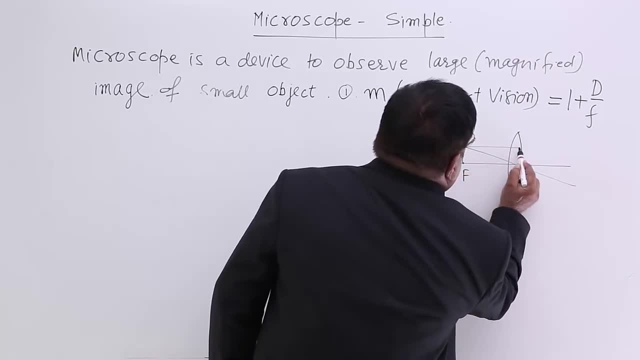 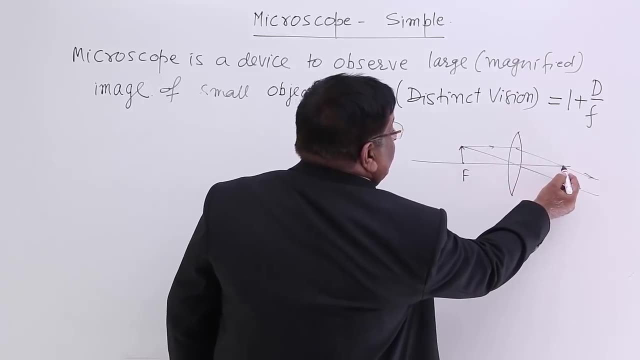 Then The rays coming from here Will become parallel, Parallel. The one which is parallel Is going through focus, same distance, And the one going through optical centre goes straight. And If This is on focus, They has to be. 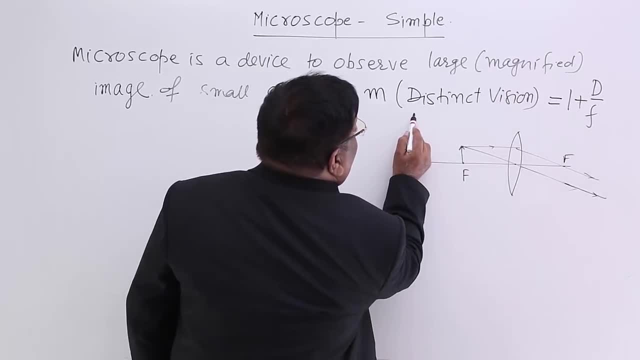 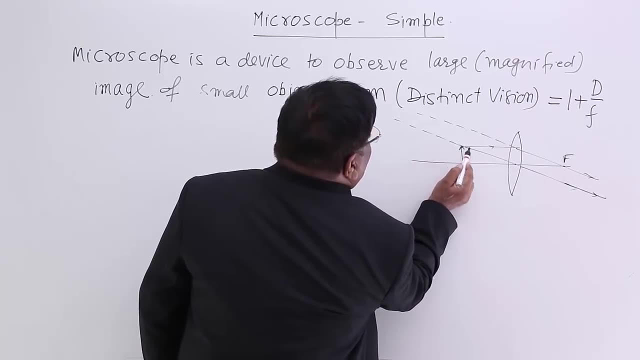 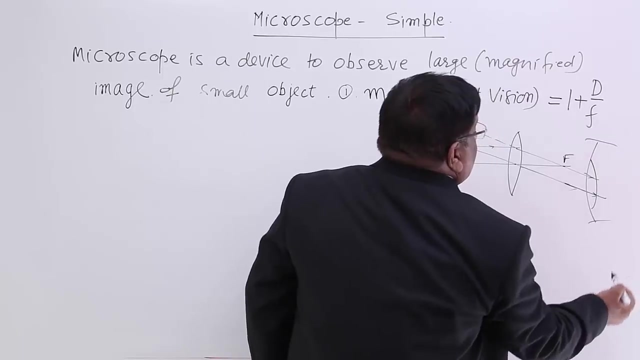 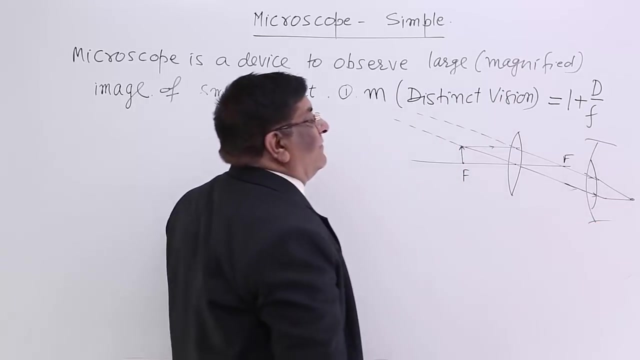 Parallel. Now, if they are parallel, Then These are supposed to come. The image will be formed At infinity. Yes, And Here we see Now. They will focus very conveniently On our Retina And there will be no tension. 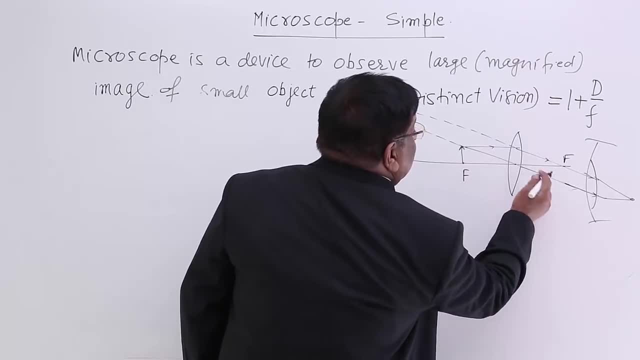 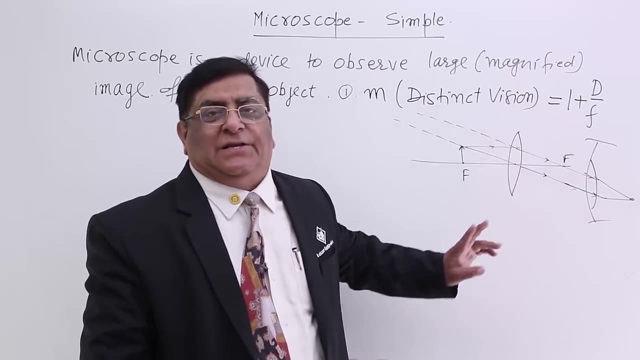 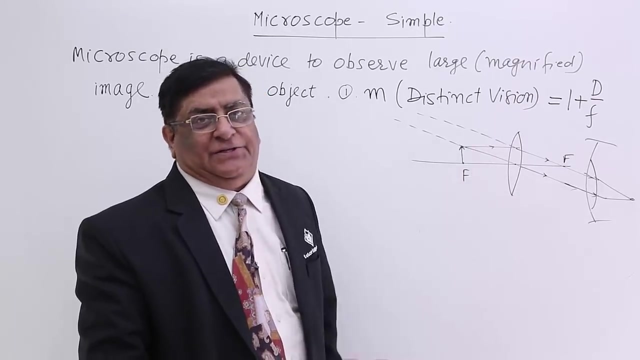 When we see an object By the parallel rays, Image is sending parallel rays, Then This setting is for relaxed eyes. Do we have any magnification in this? Okay, Now let us calculate Magnification in this. These rays are coming from. 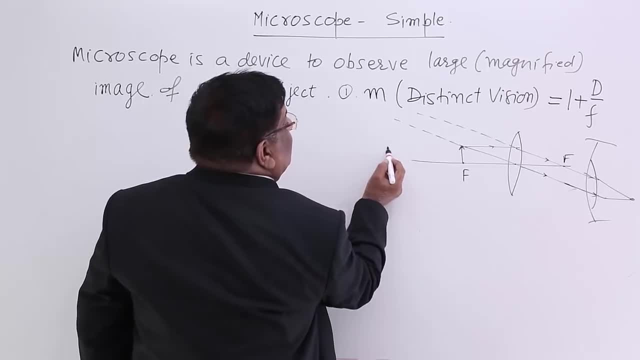 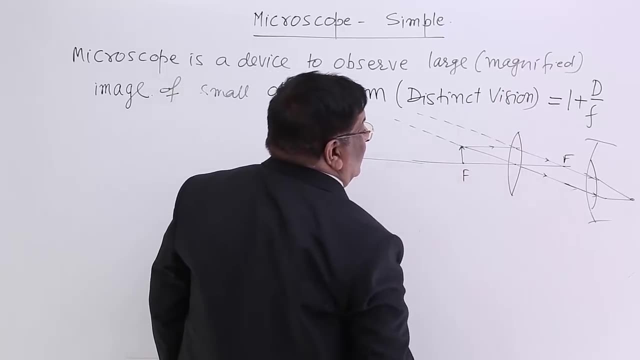 Image. Image is somewhere here, Here, Here, Here, Here, Anywhere. Image is somewhere there And these are coming from the image And we see That They make an angle To the eyes. They make an angle. 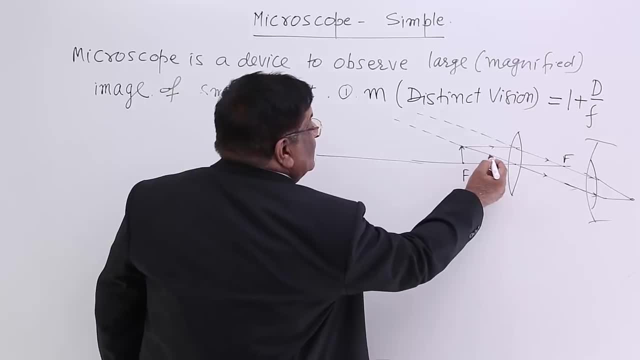 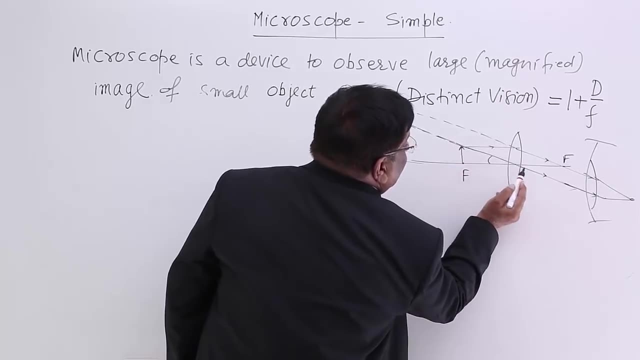 That is equal to This angle. This is the direction From where The rays are coming. So Let us say This angle is beta. So what is beta? Beta is Angle Subtended By Image. So 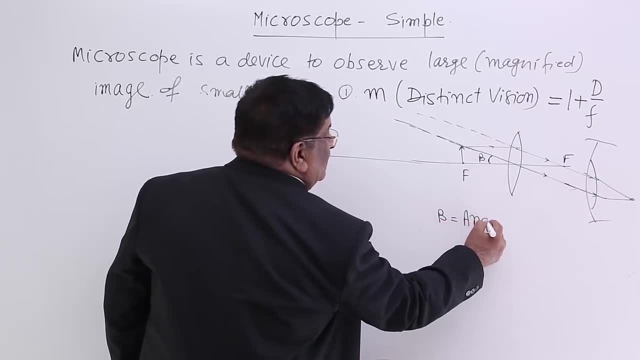 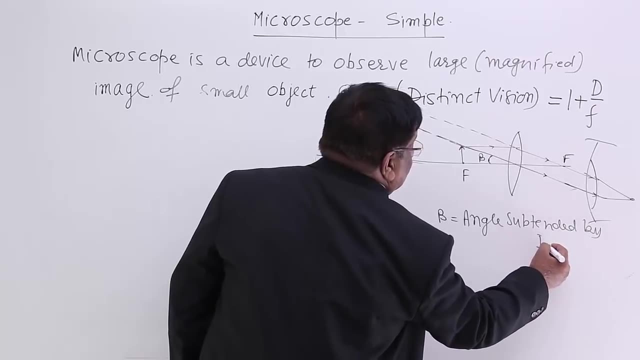 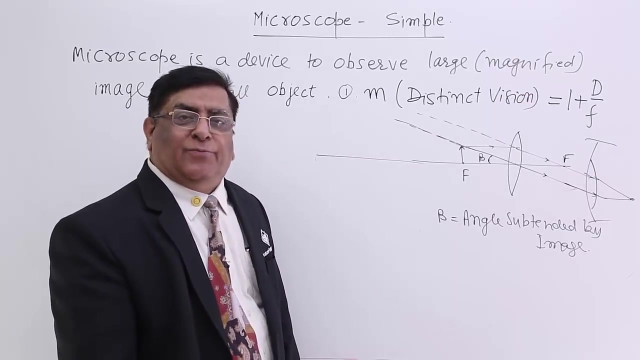 Let us say: This angle is Beta. So what is beta? Beta is Angle Subtended By Image. So This Angle Subtended By Object. Now, What is the angle Subtended? 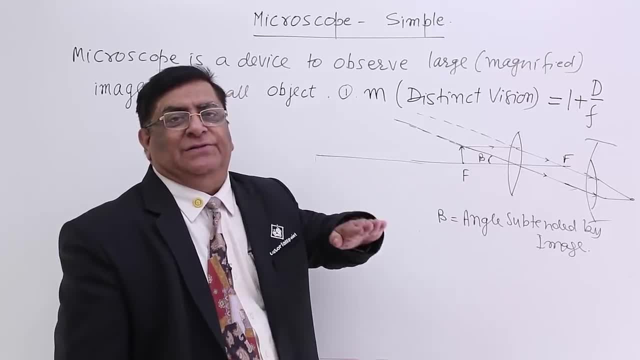 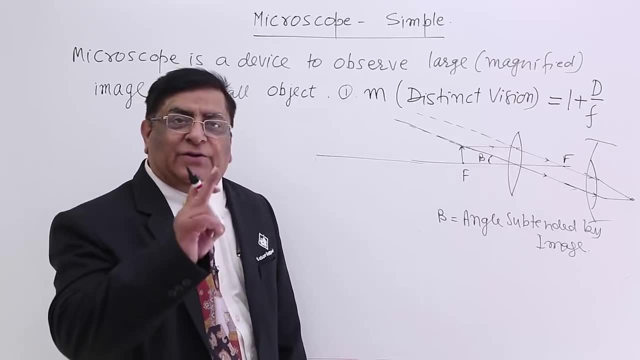 By Object. We divide the two angles, Angle By Image, Divided By Angle By Object, And that will give the magnification. Now, The condition for that, You studied That Condition for that is: 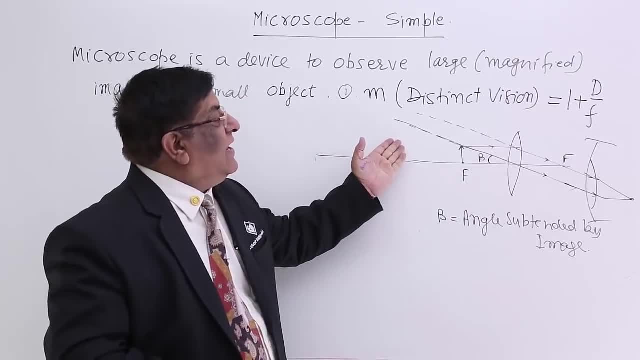 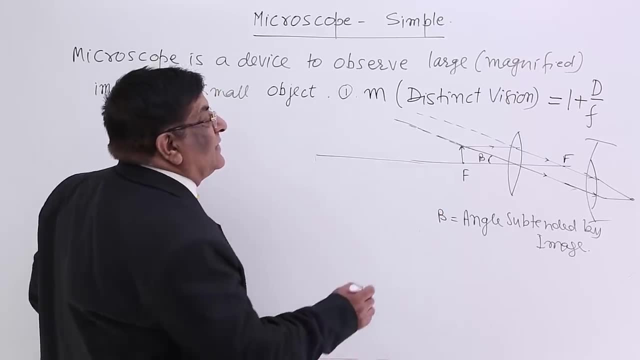 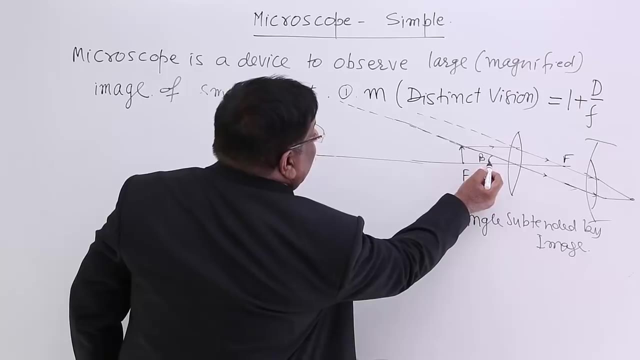 Both should lie At the same place. Now We do not see Where. Image And Object At the same place. There is one method. We know That Image Is Coming From Image Rays. 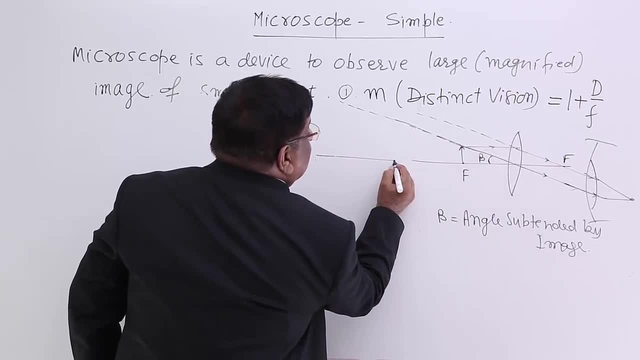 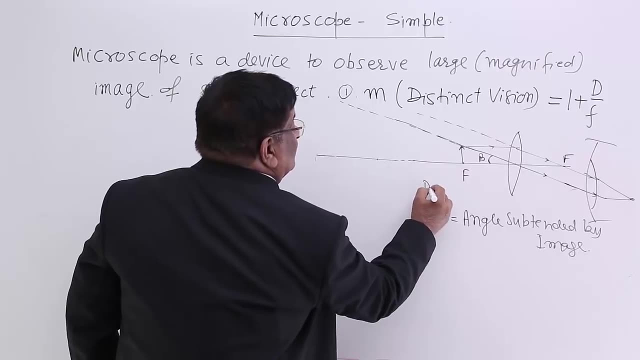 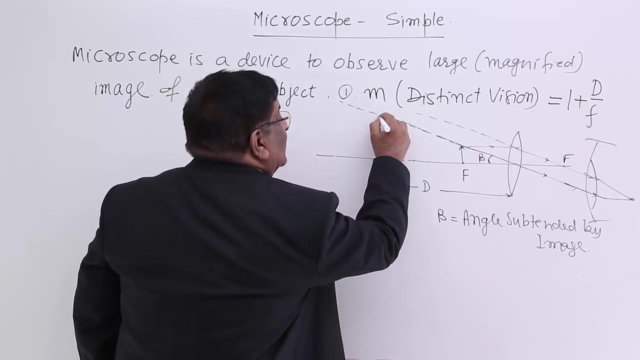 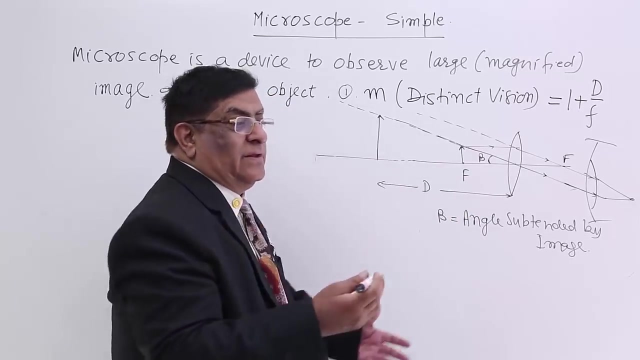 Are Coming From This Direction Which Is Making Angle Beta. So What We Choose? We Choose Image Here This: How Much Is The Angle Made Beta? 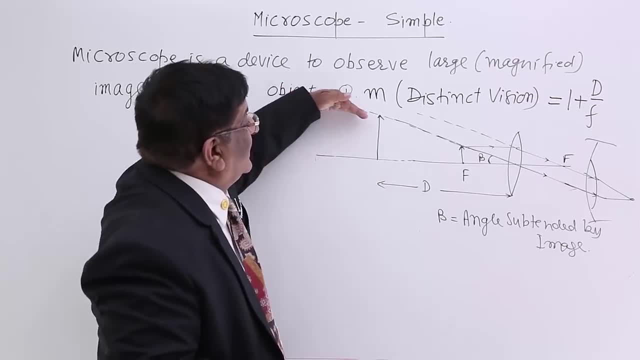 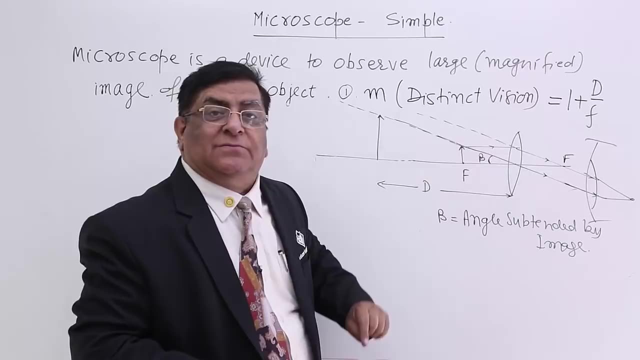 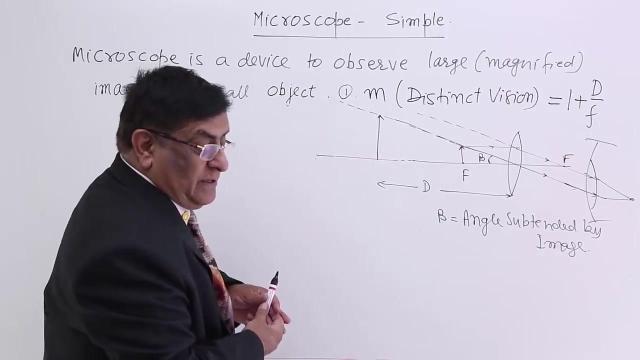 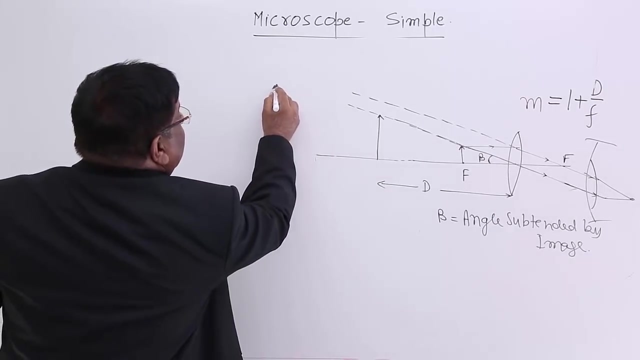 How Do I Say That This Is Image? Okay, This Is Not Image, But This Is Representing Direction Of The Image, Maybe At Any Location. 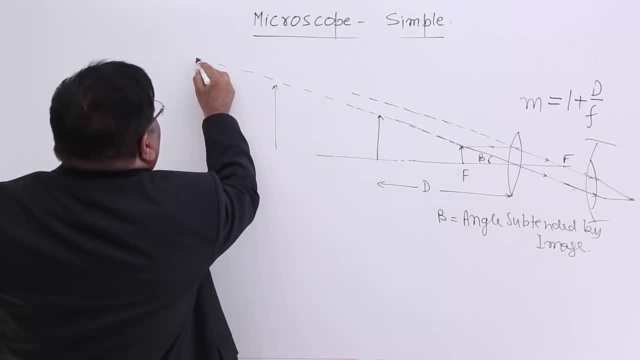 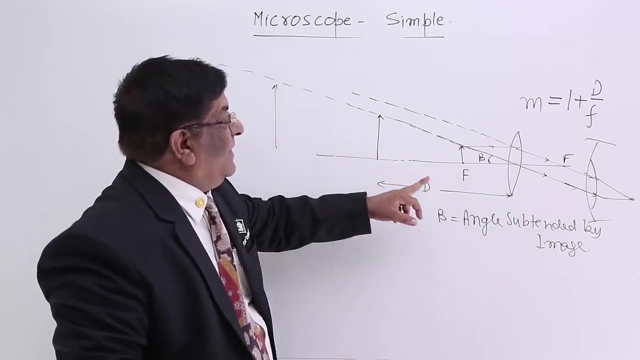 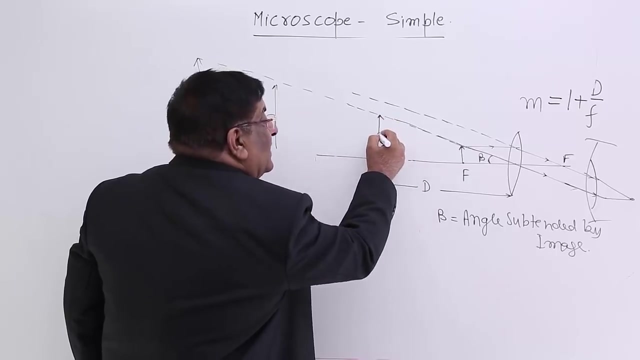 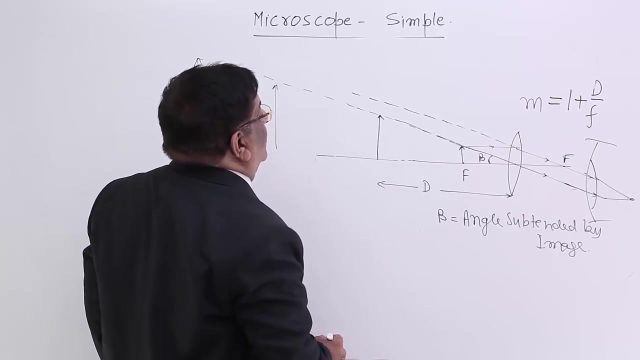 Maybe It Is Here, Maybe It Is Here Anywhere, But This Makes Angle Beta, That Is For Sure. So Image Is Making Angle Beta Now. 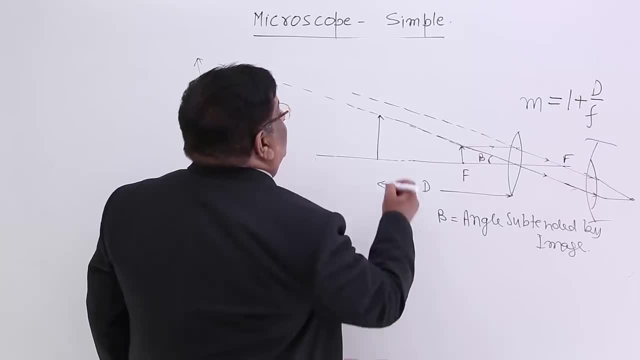 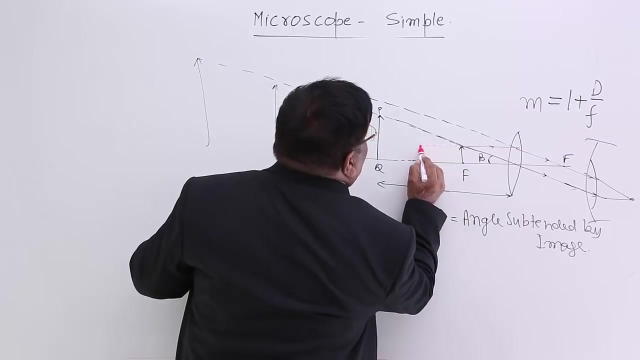 Image. I Will Give Certain Name To It. Let Us Call It P Q. That Is Image Now At The Same Place. How Much Is The? 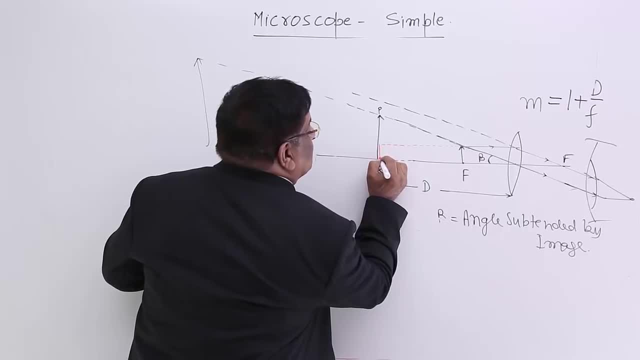 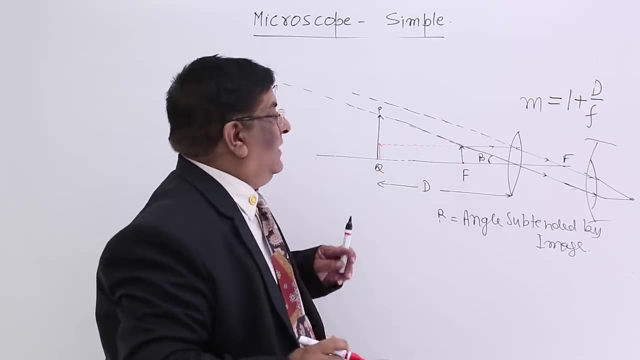 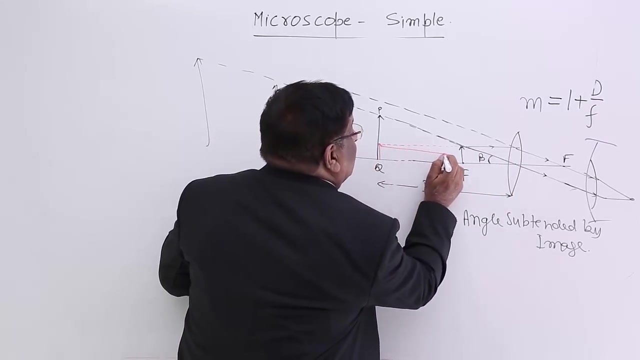 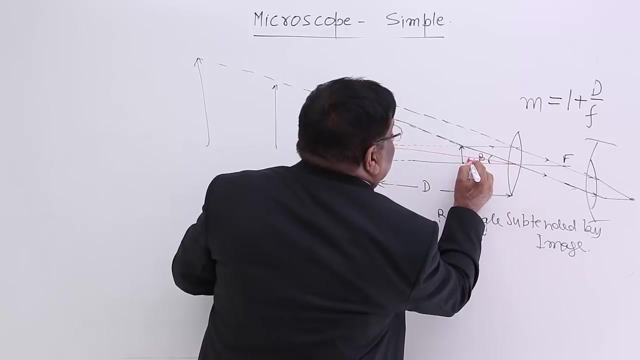 Angle Made. This Is This Object, If It Is Placed Here For The Sake Of Comparison Only. So It Is Here. How Much Angle Will? 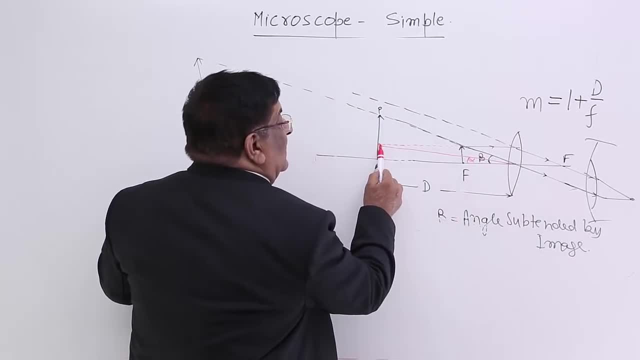 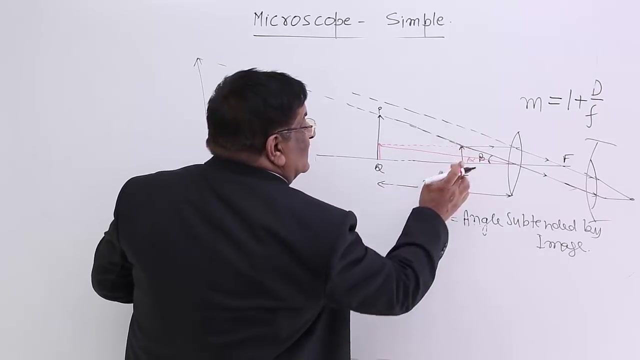 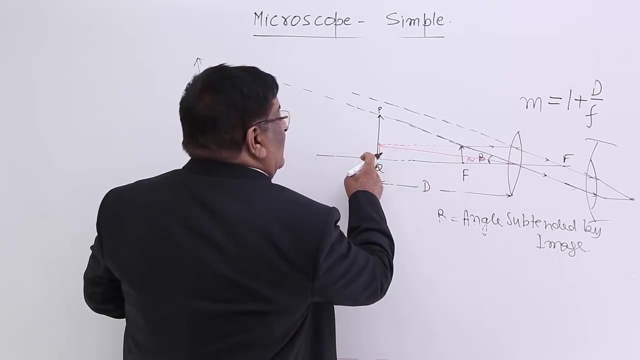 It Make At This Location. It Is Place At Same Location Of The Image. I Have Chosen This Location Because I Know A Known Distance. 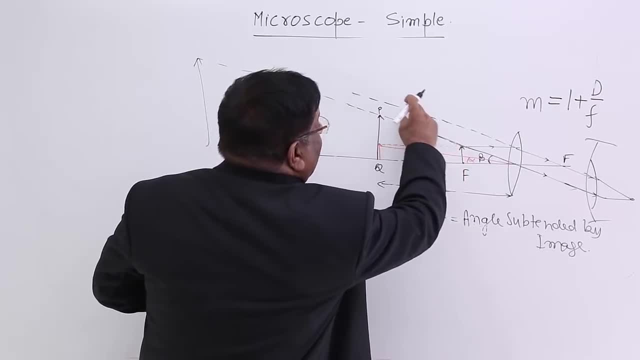 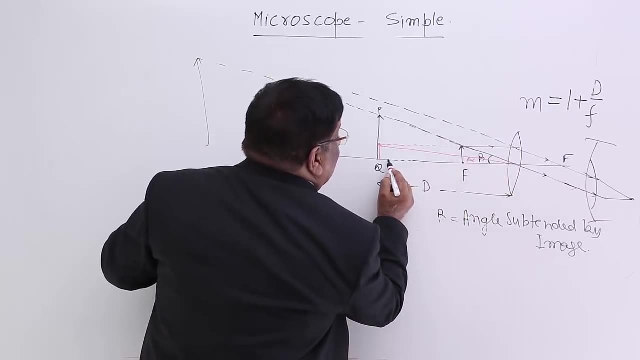 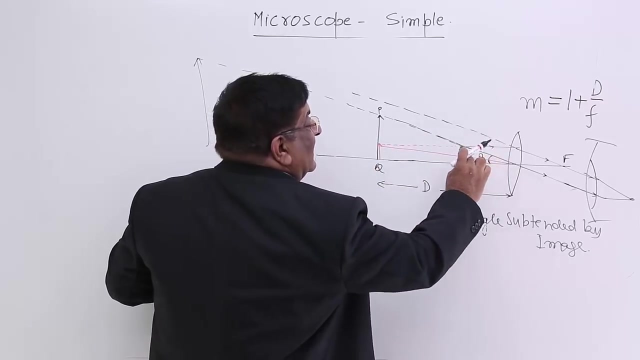 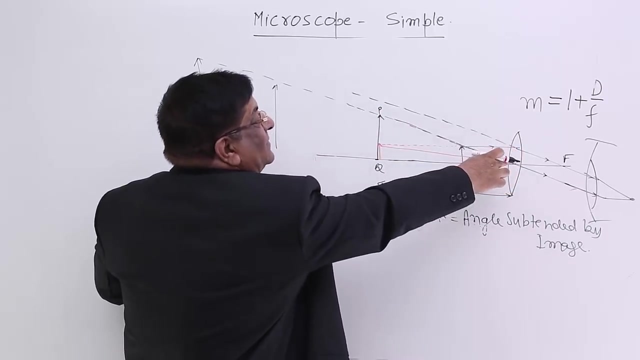 Which Is D Okay. So At This Place, This Is Image Made By The Object. This Is Bottom Of The Object. This Is Top Of The. 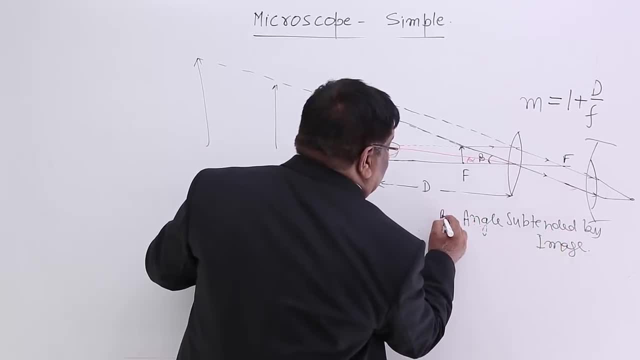 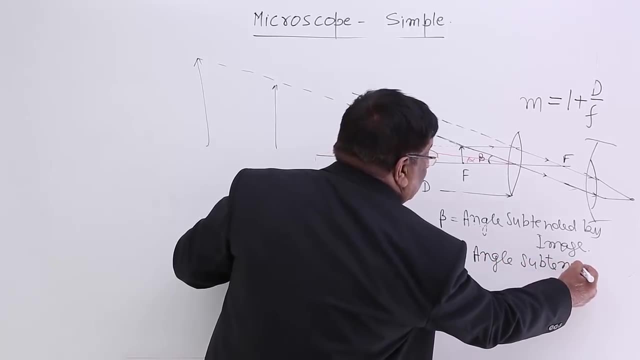 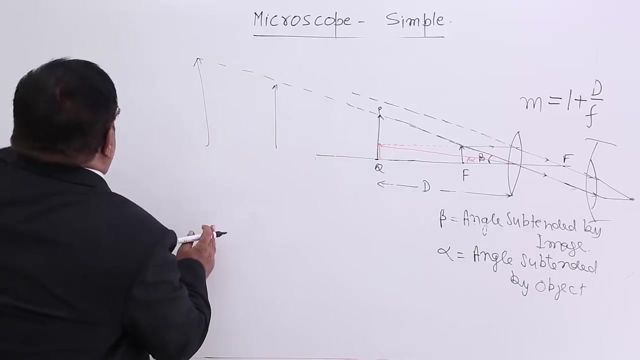 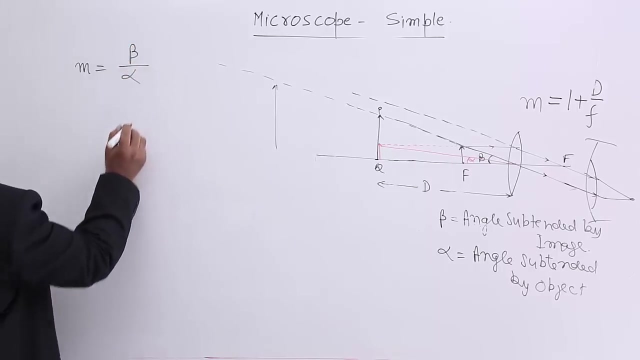 Object And This Subtend An Angle, Alpha. This Is Bottom Of The Image, This Object, Therefore, Magnification. Magnification Is Equal To Beta Upon Alpha. 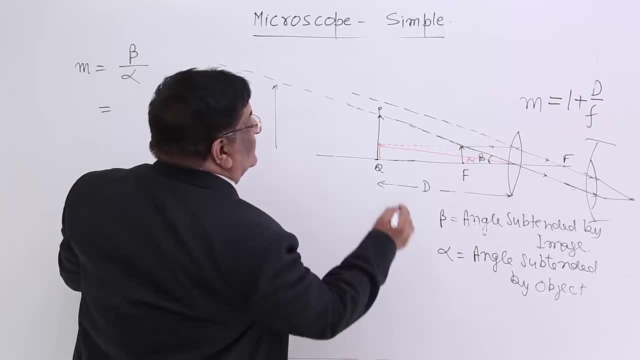 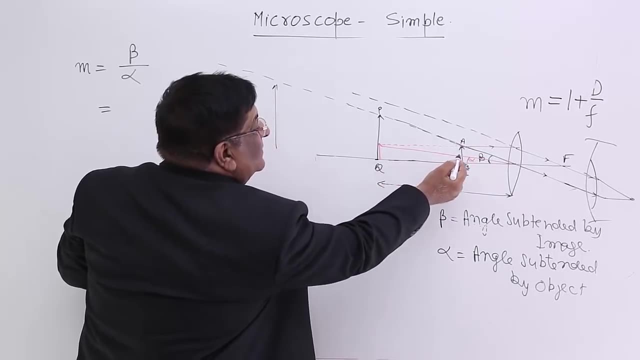 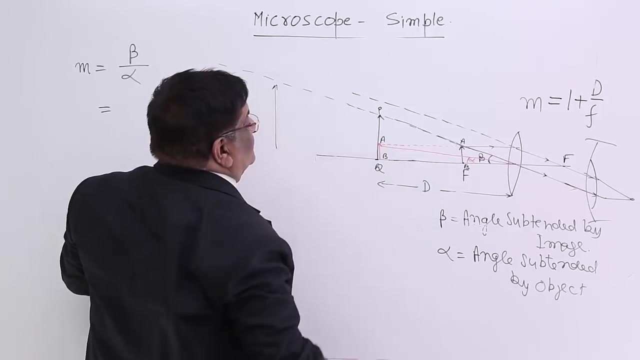 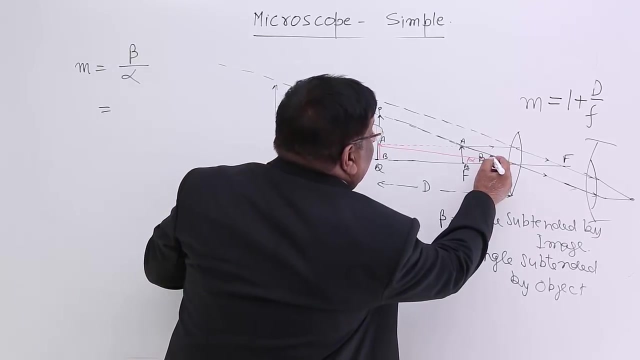 Now I Do The Calculation Here. This Is Object A, B, A, B. And When I Do A, B Now, Magnification Is Angle Beta Upon. 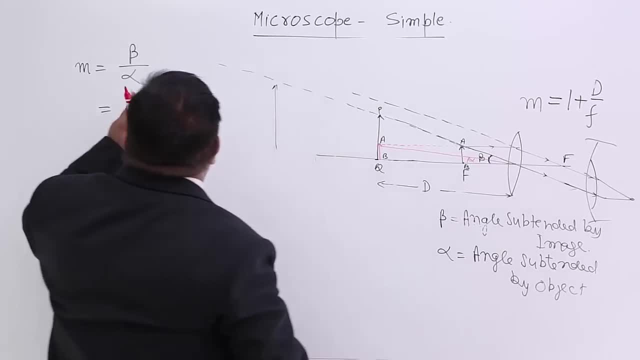 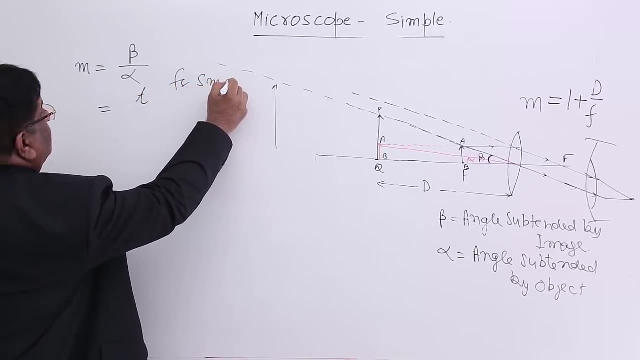 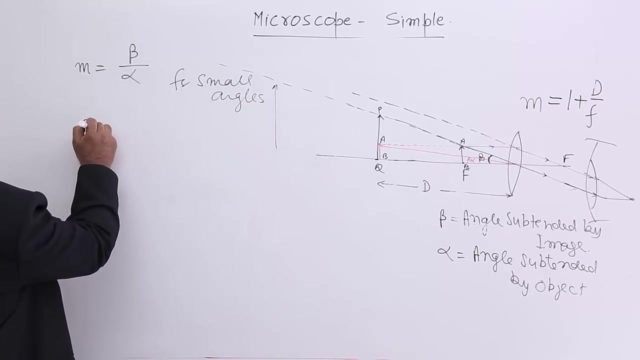 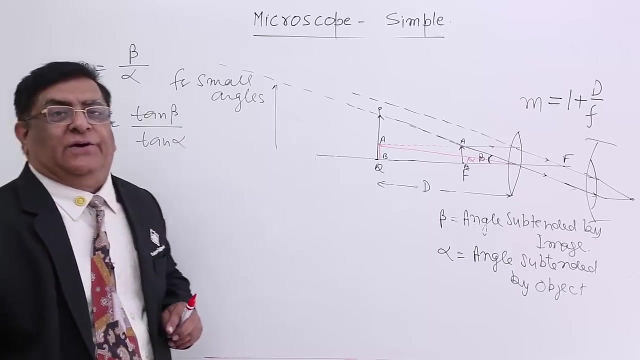 Angle Alpha. This Angle Beta- I Do A Measurement For Small Angles- Beta And Alpha Are Equal To Their Tangents For A Beta Upon Tangent. 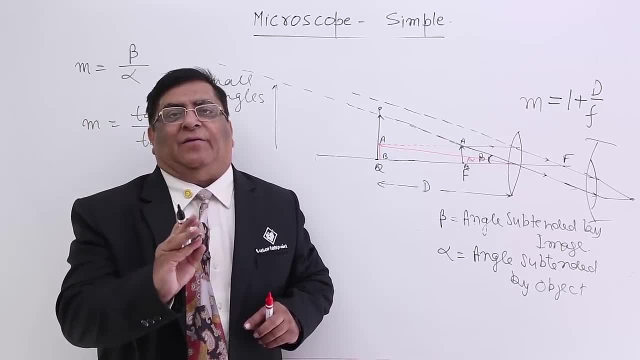 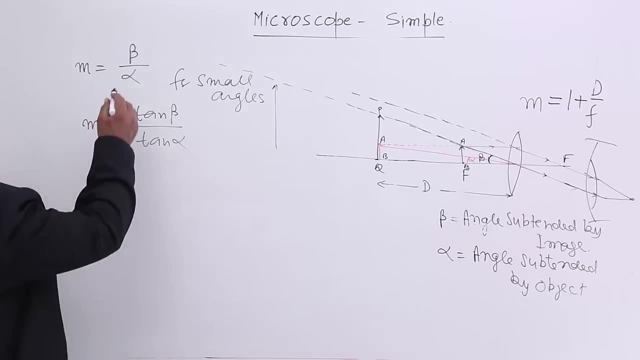 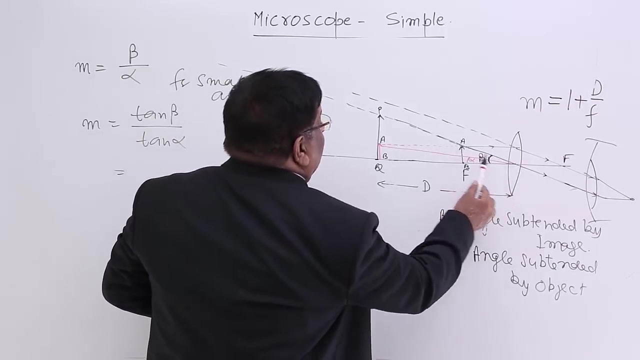 Alpha. We Know That For Small Angles Beta, Sign Beta And Tangent Beta Have Almost Same Value, So We Can Transform As We Need. So 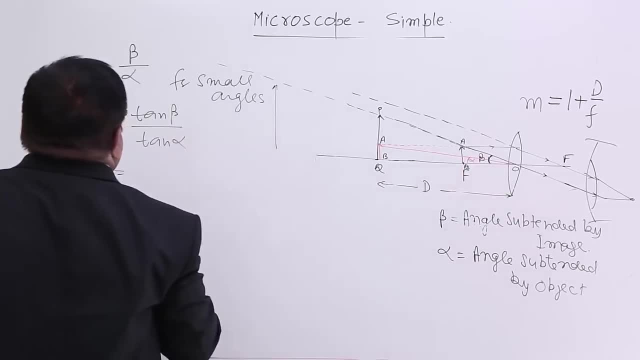 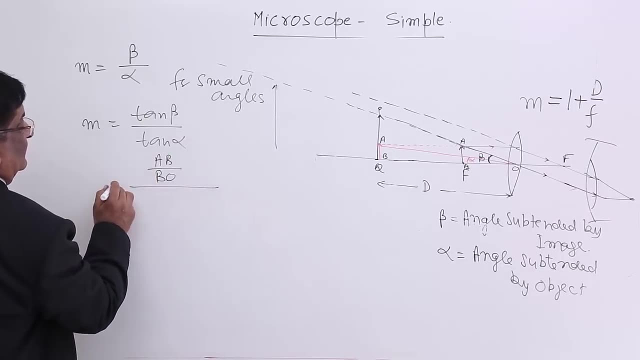 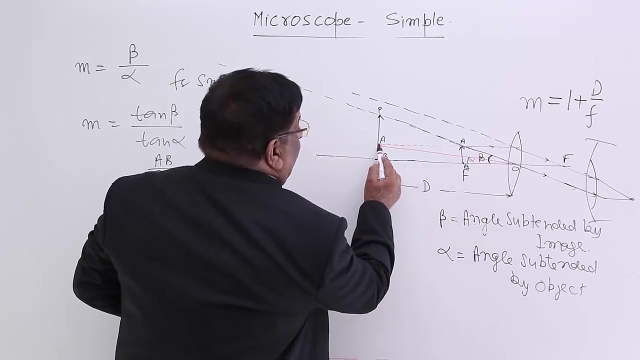 This Is A B Upon B O. This Is A B Upon B O. Tangent Alpha. This Is Alpha. Its Tangent Perpendicular A B. 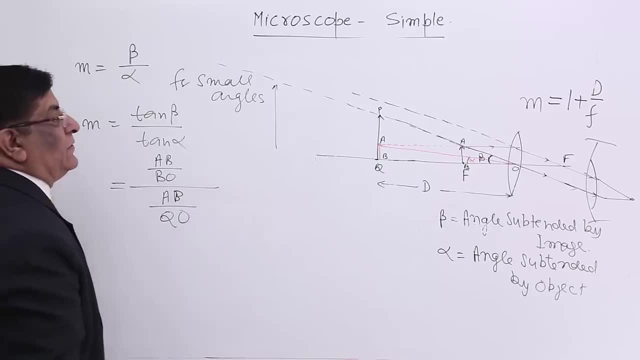 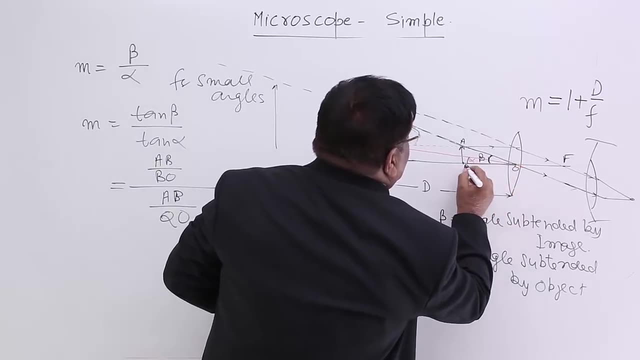 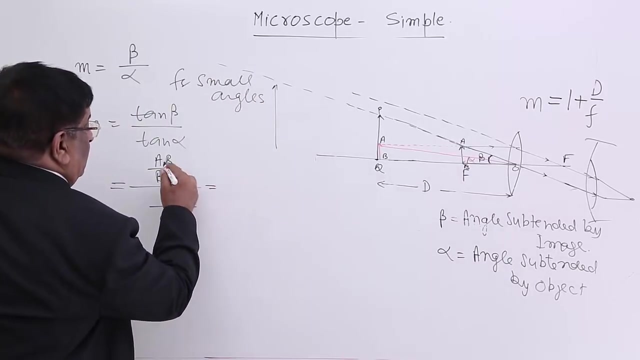 Upon Q? O. A B? Upon Q? O, Because This Is B? O This Distance, This Is Q To O, So This Is A B Upon. 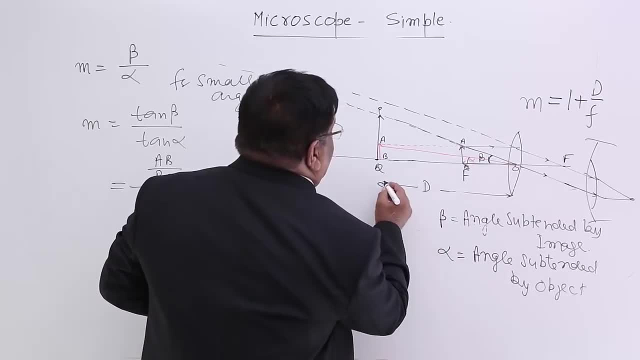 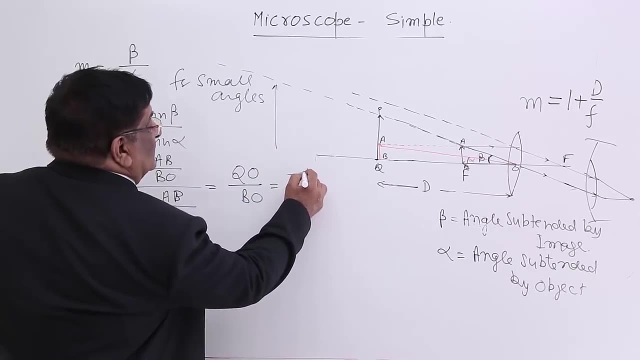 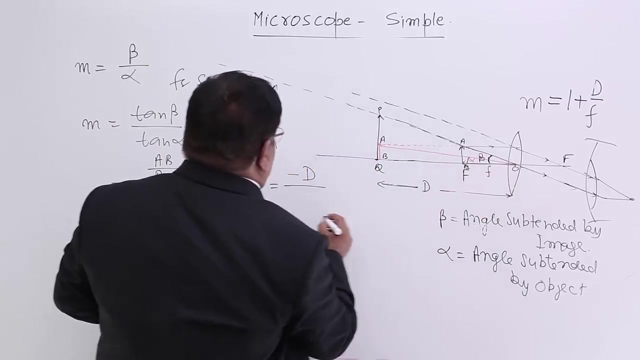 Q? O. Now Simplify The Two. This Becomes Q As Minus D Divided By B? O. B O Is Focal Length, So This: 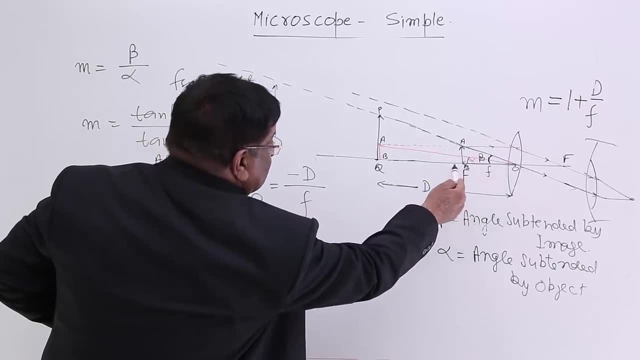 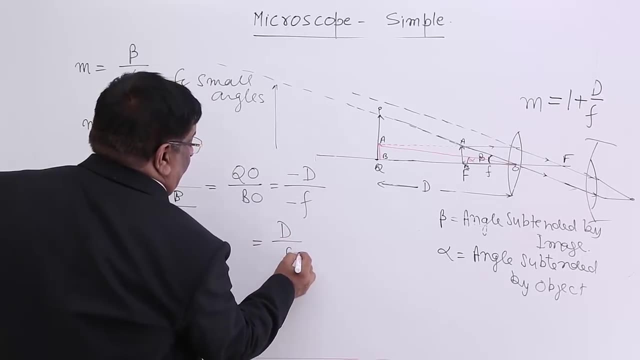 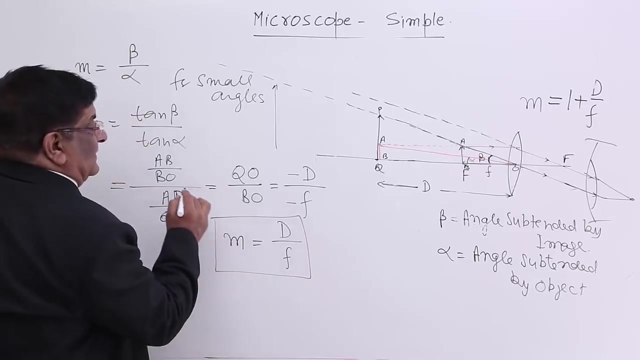 Is Minus. D, F I Have Taken On This Side, So This Is Minus. So In This Particular Case, Why Should We Take It? 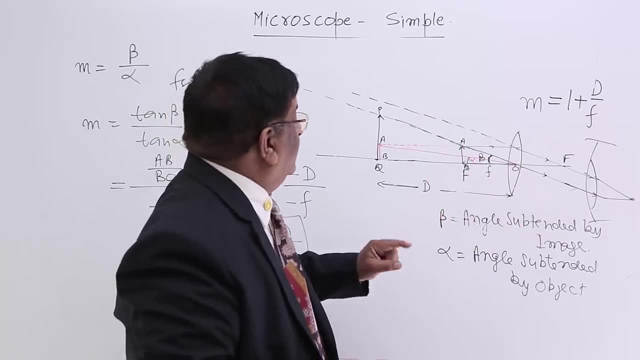 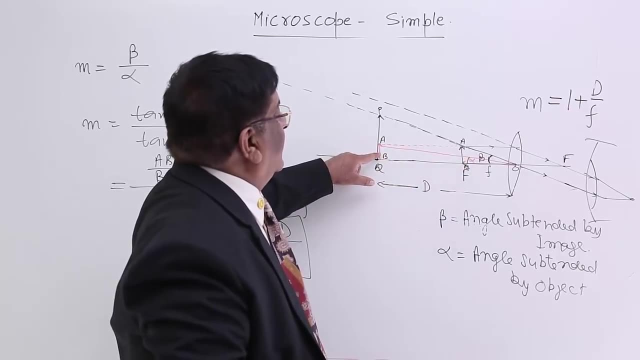 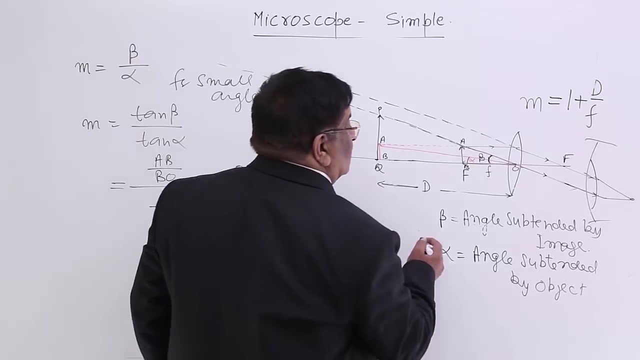 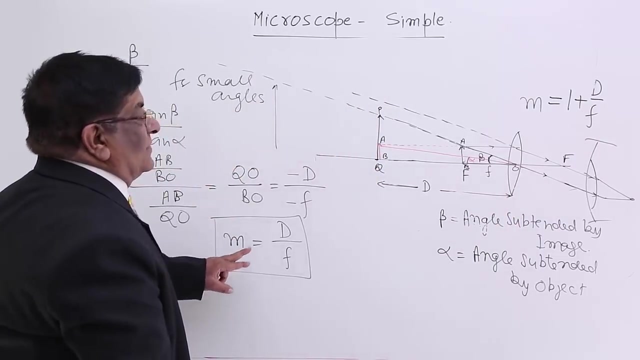 As D, Because We Put Our Newspaper At The Distance D. We Are Used To That, So I Put It On. So This Is Calculation For 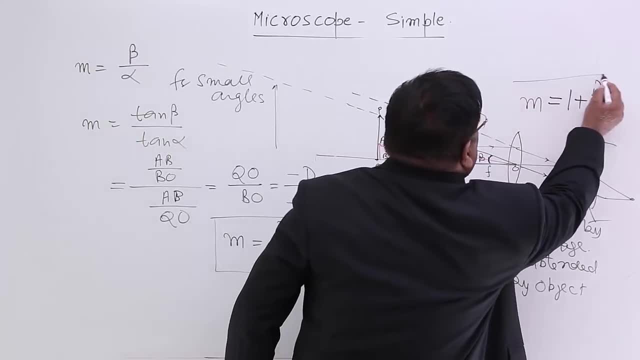 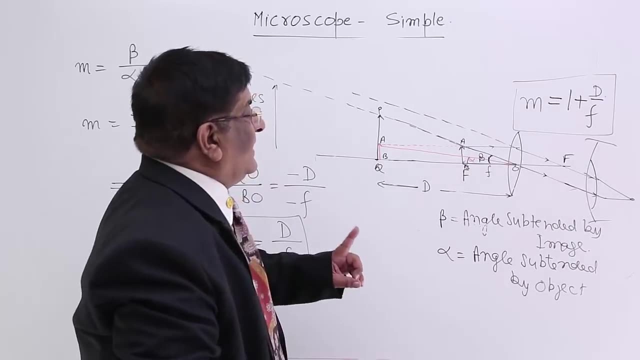 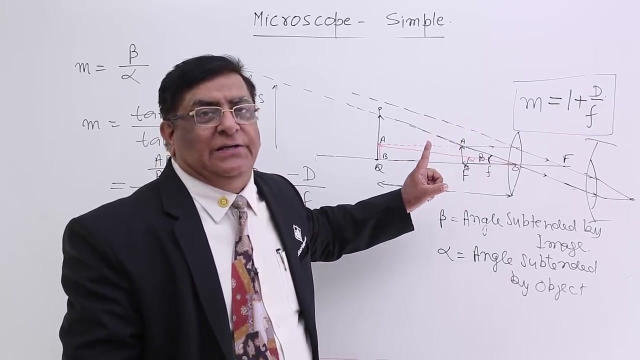 Parallel Race Or Relaxed Eyes. This Is Calculation For Distinct Vision. So We Have Two Setting: One For Distinct Vision Where Image Is Clearly. 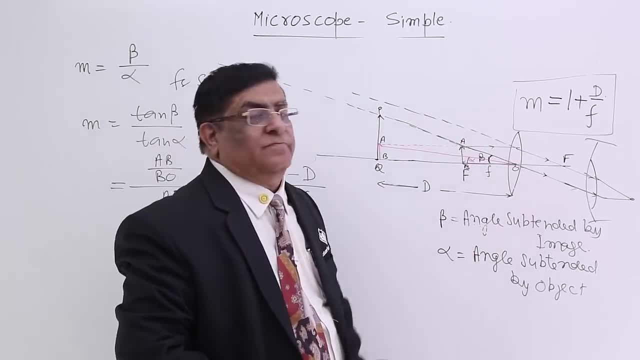 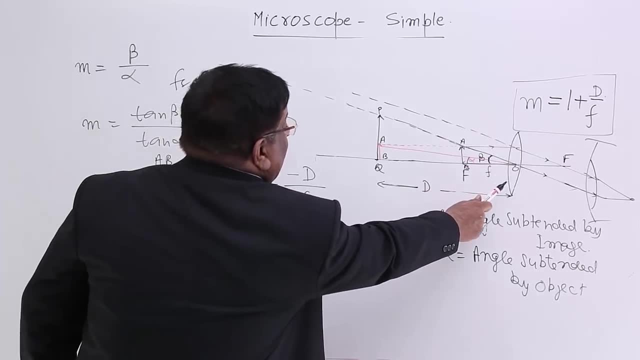 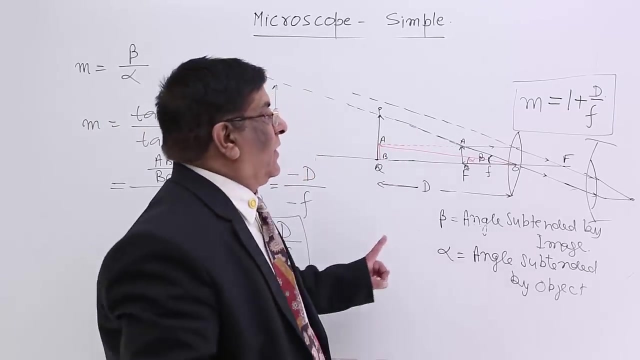 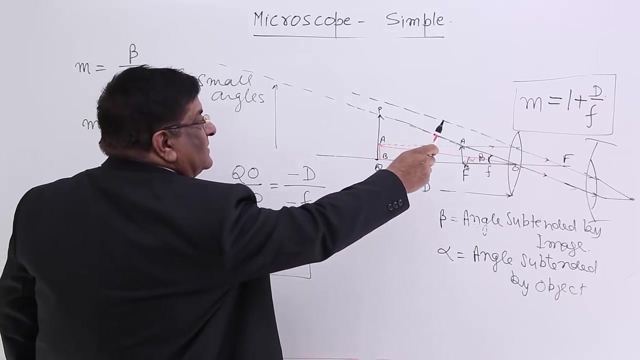 Coming From The Image, So You Please Remember These Two Settings. And This Is For Magnification By A Simple Microscope And After This, If This